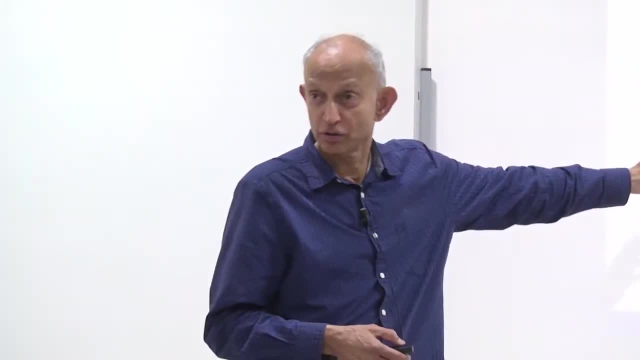 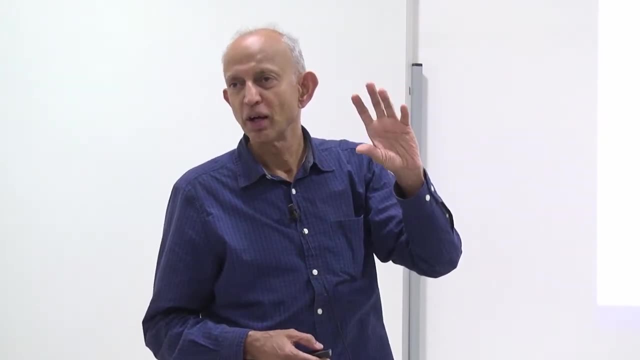 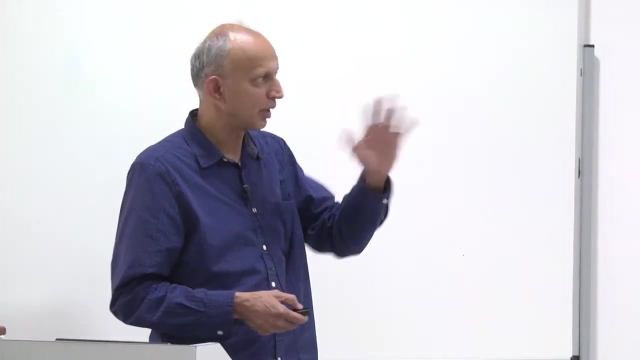 That's what we want to show. The advantage will be the time will be much faster. You'll have to do essentially SVD on a very small matrix and from that you'll get everything. So that's the advantage. By the way, one thing I did not say is length squared sampling can be a pretty 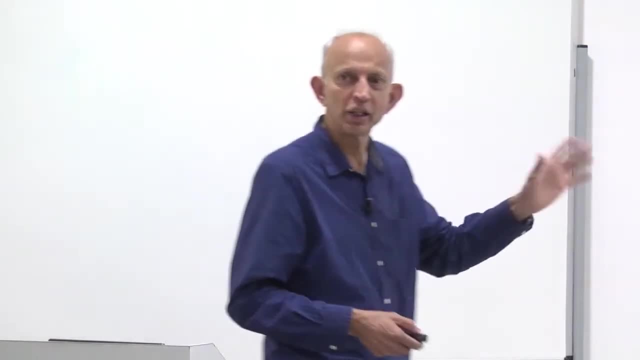 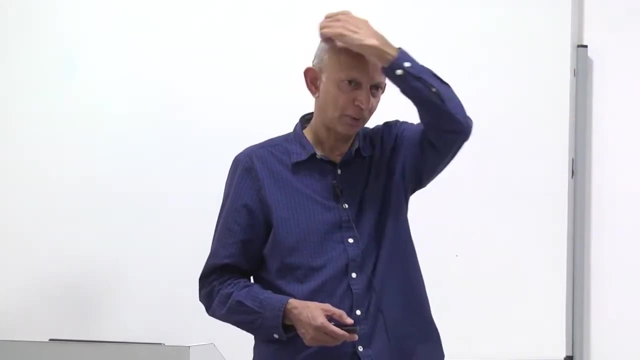 good thing, Yeah, And it can be applied to infinite matrices as well. I didn't go into that much. So if you have infinitely many columns, but of course you have to have a convergent sum of squares, Otherwise you can't do it. 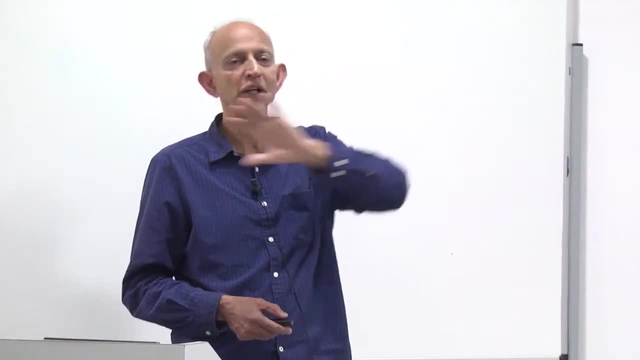 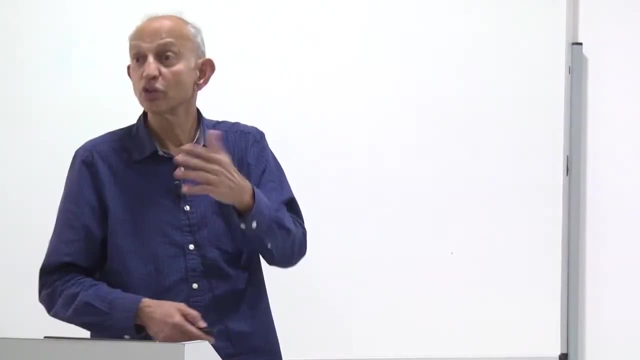 Then you can sample a finite set: the infinite number of columns, but finite dimensional. You can sample a finite set and all of this goes through, but we didn't see that. So that's another advantage of doing this, as opposed to full SVD. 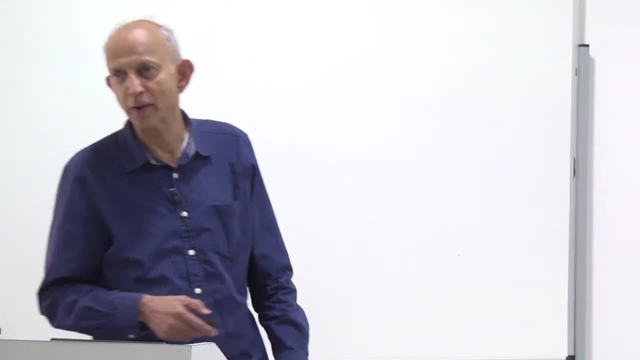 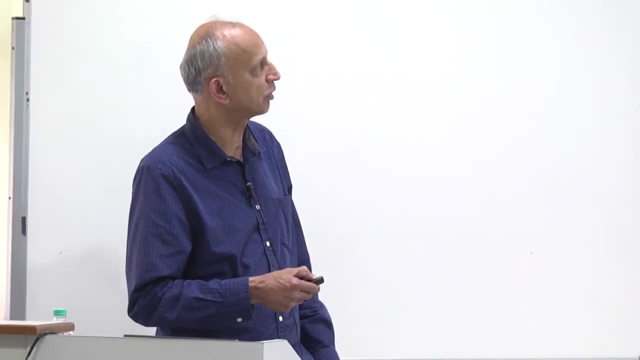 because if it's infinite, then full SVD is impossible, right? Okay, so SVDs all again. I'm just repeating this: SVD is the best approximation of each rank. What we'll show is, if I pick a length squared sample of just. 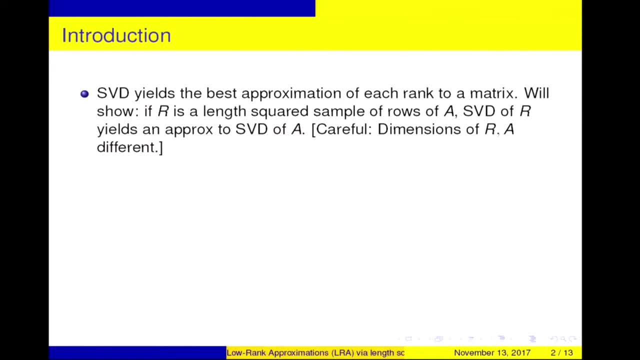 rows of A and I do SVD on R. just on the matrix that looks like that. that gives you a decent approximation to the SVD of A. Now we have to be a little careful. A is the dimensions are different, right. 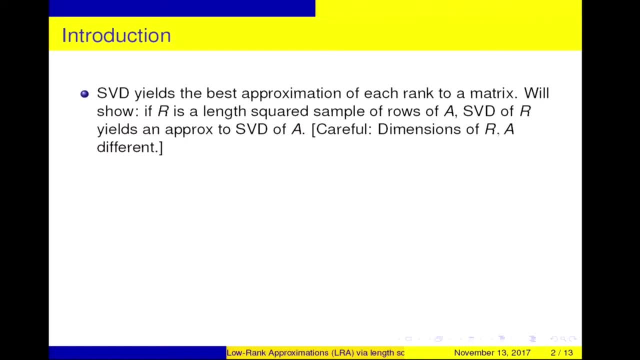 So you have to relate this speed to it, the SVD of R to the SVD of A, in a nice way. we'll see that, okay. So in fact, most of the central result here will not be anything to do with length squared sampling at all. 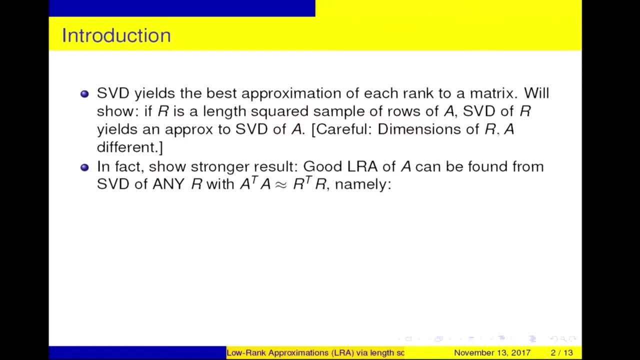 It's a purely matrix perturbation result and we'll prove the following: If I get a good low rank approximation of R, provided R transpose R and A transpose A are close. Now just nice to recall the dimensions of those. So if A is N by D, 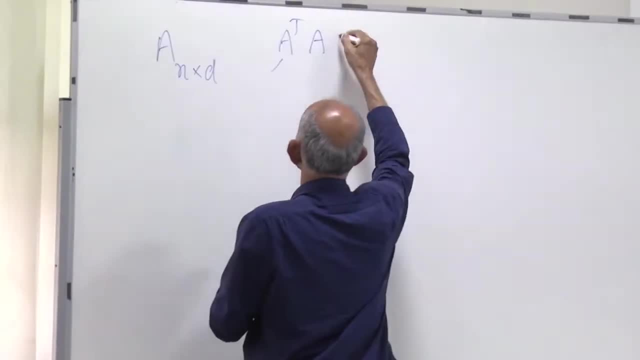 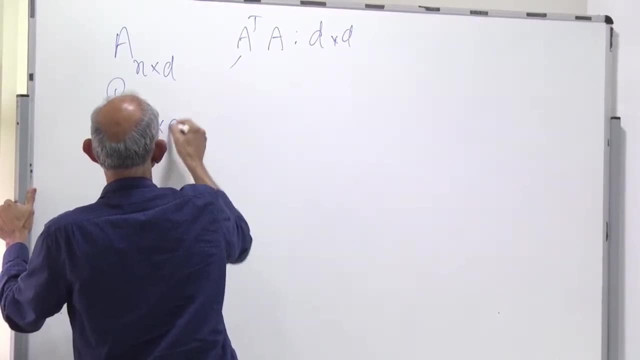 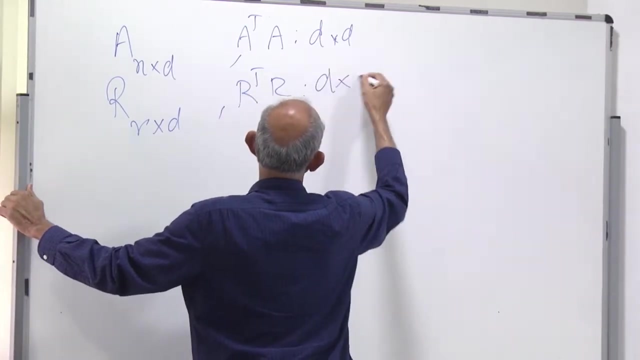 A transpose A is D by D, and so is R transpose R, R. only some number of rows have been picked, so it's little r by D, but R transpose R is also D by D. right, And maybe again just a picture. 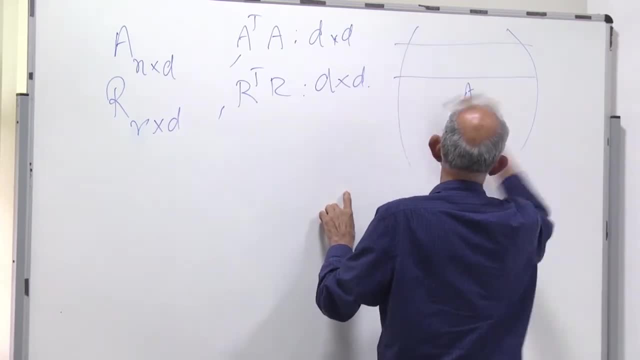 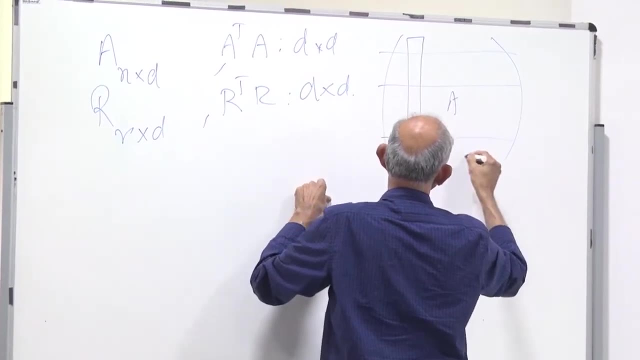 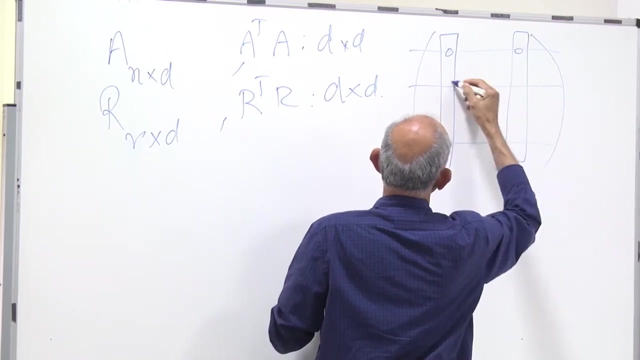 So if I have this as my A the rows I sample only a few rows: A- transpose- A wants to take the dot product between every pair of columns right And R- transpose- R just takes the dot product of the sample in the sample row right. 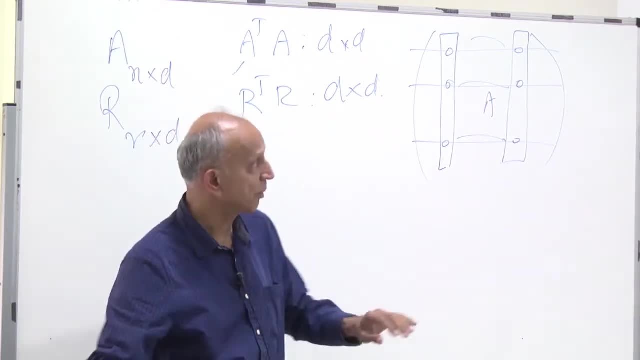 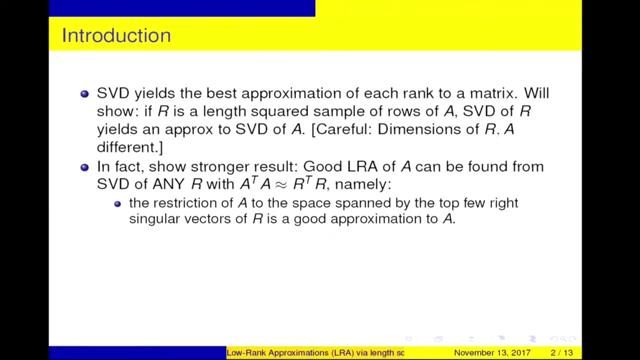 I mean just writing a picture of it. So they are the same dimensions, so it makes sense to say that they'd be roughly equal. And what we will actually show, and I'll show, is the following: again, the dimensions are different. 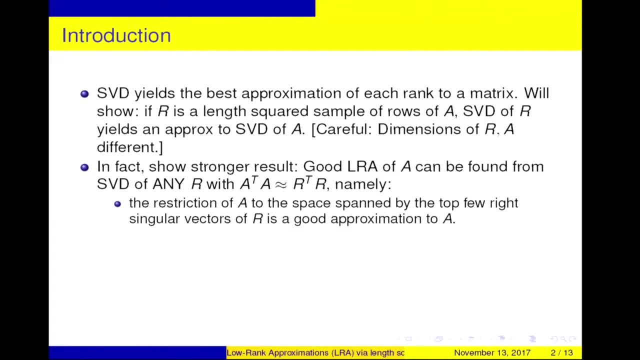 So the relation will be this: If I restrict A as a linear transformation to the space spanned by the top few right singular vectors of R, that's a good enough approximation to A. Now, that's the right dimensions, right. The right-hand side dimension of R is right. 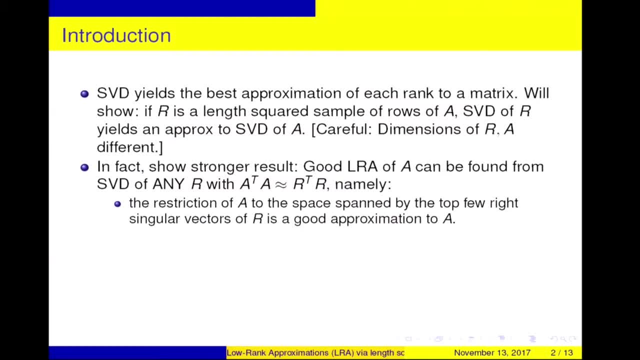 Okay, this is what we'll show. So the main result really doesn't have to do with length squared sampling, it just has to do again with this. I will show you In a way I perturbed A. you can think of it as I perturbed. 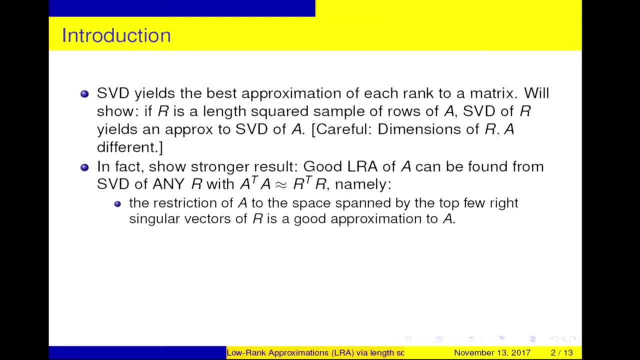 A transpose A. to get a slightly different matrix: R transpose R. Except it's a lot simpler because it's a product of two matrices which are smaller. If the perturbation is not bad, then this is true. We'll prove that, okay. 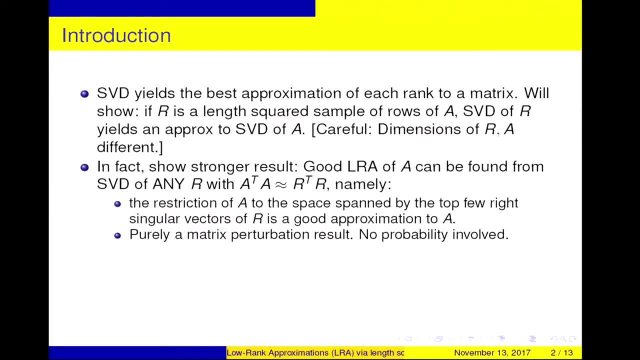 And then this is really again purely matrix perturbation results. There's no probability in that. I'm not involved in that part, But as we saw, we will see again. we'll recap That if I have a length square sampled R, then A transpose A. 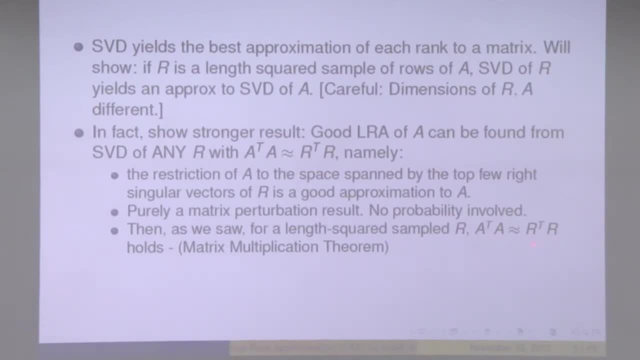 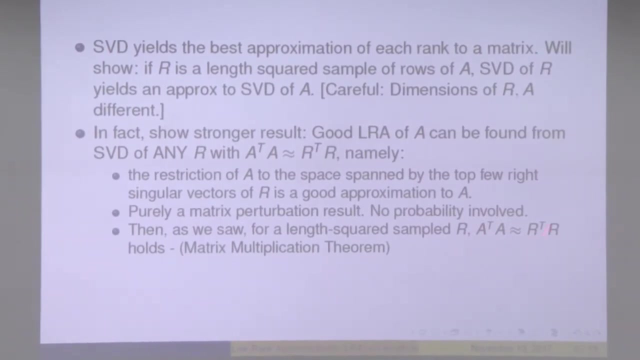 equals R transpose R, roughly approximately. And that's the familiar matrix multiplication theorem. So if I were multiplying the matrix A transpose with the matrix A, I might do that by picking some columns of A transpose which are rows of A. Okay, so there's the matrix A transpose, and so on. 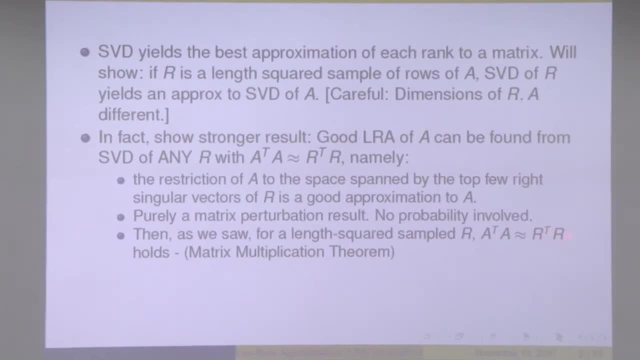 And that's my R transpose And then pick the same rows of this A, which is R, okay, And matrix multiplication theorem in spirit- I mean we'll quantify this In spirit- told us these are roughly equal And this perturbation result is going to tell us if these are. 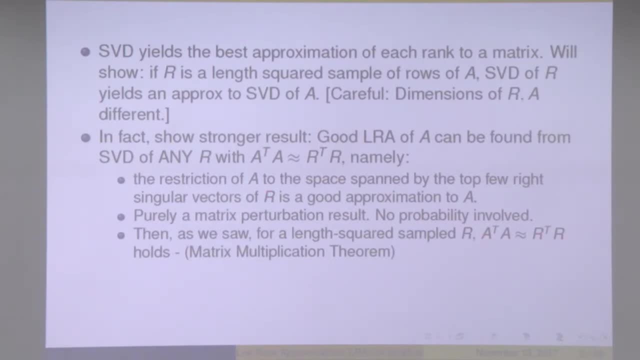 roughly equal, then in fact, SVD of R will give us SVD of A. Now let's recall that R itself. I want the here, I want the right singular vectors of R. R is the right dimension, is very high right. 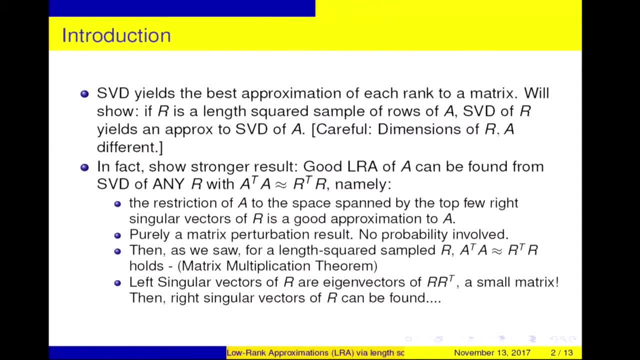 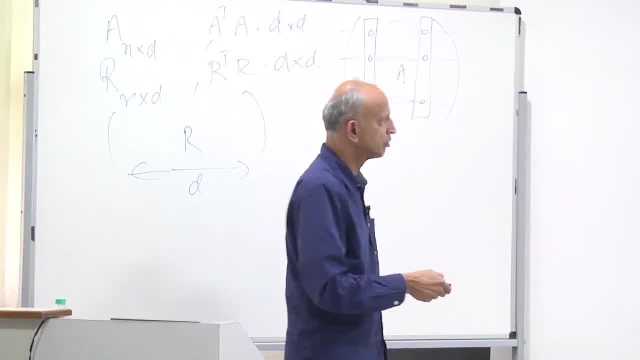 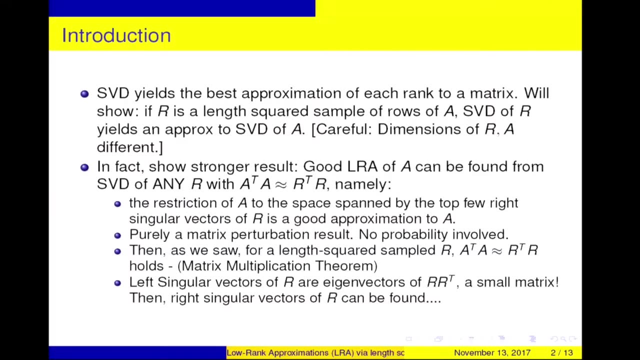 Cuz. R is like this: This dimension is still D, So that seems to be a D dimensional problem. But observe that R is only R by D. I could take R, R, transpose. Okay, that's a small matrix. It's a little R by little R matrix. 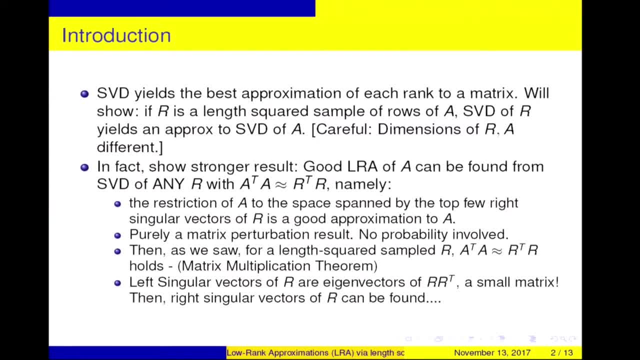 That's got only this many rows and this many columns. I can do. I can find it's right. singular vectors of R. now, I'm sorry, The left singular vectors can be found from this. These are just eigenvectors of R. R transpose. 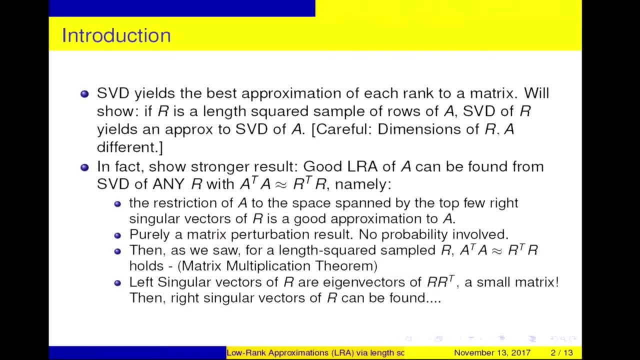 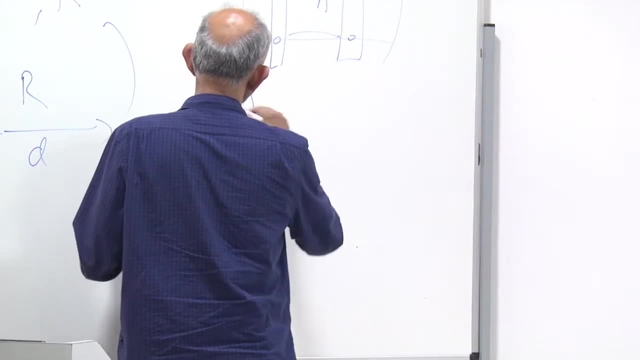 We saw that the spectral decomposition of R- R transpose- is related to the singular value decomposition of R. So the left singular vectors, they can be found, And then you find the right singular vectors by folding them in right. So we saw that. we saw that if I take a matrix A and 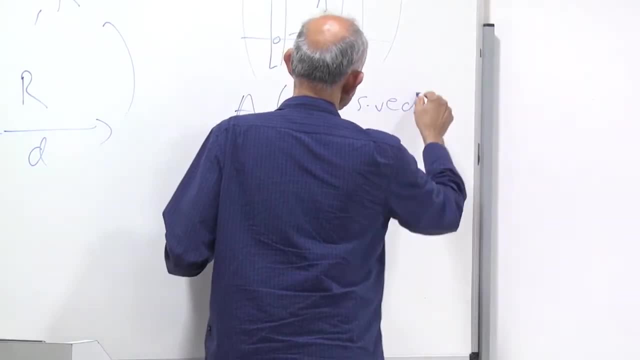 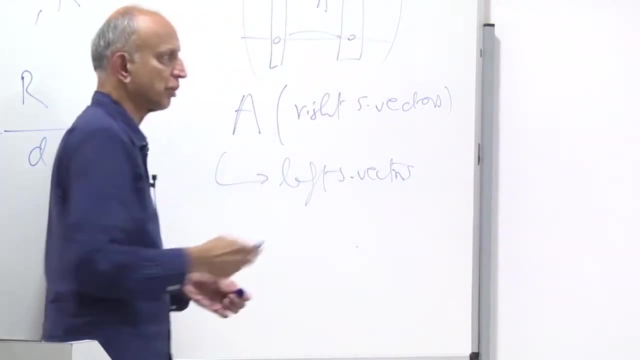 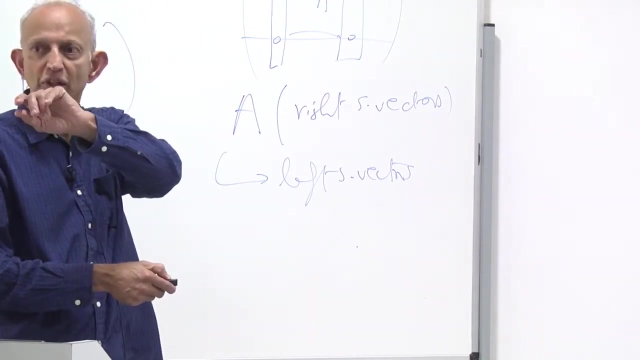 then multiply on this side by the right singular vector, I get the left singular vector And vice versa. So I want, so I have to do I just the essential computation I have to do that answers that question is that I have to find. 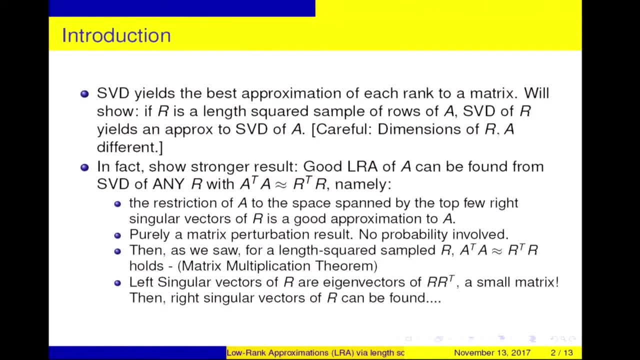 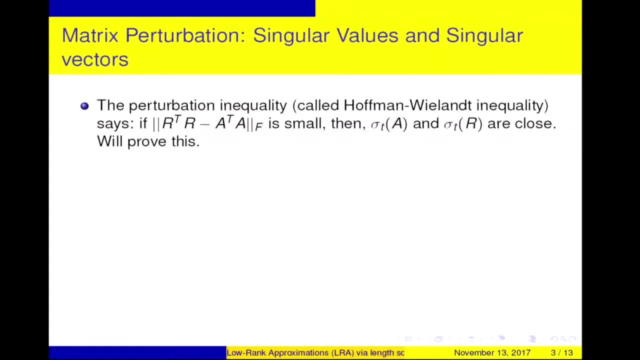 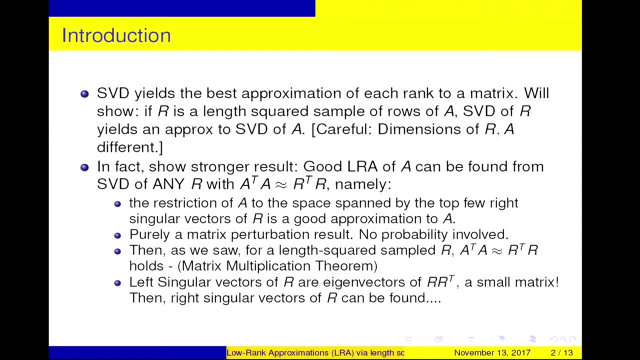 spectral decomposition of very small matrix. okay, But then I have to do some matrix vector multiplications. Those are simpler, right? Okay, this is the gist of the story. So first I'm going to prove the matrix perturbation result And I'll do a self-contained proof. 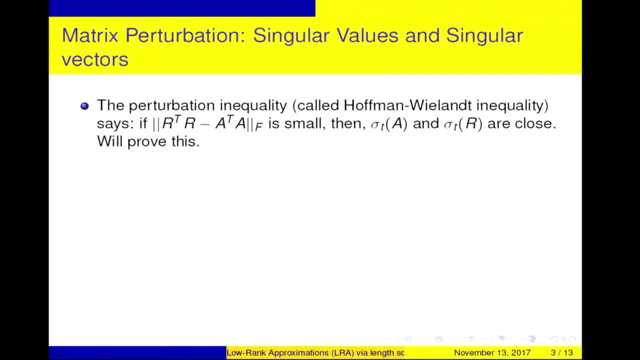 That will involve some classical results, which we'll go over. So singular, values and singular. but here's another point that'll be nice to make, Which is an important point from linear algebra, right. So this is also something standard, but I want to make this point. 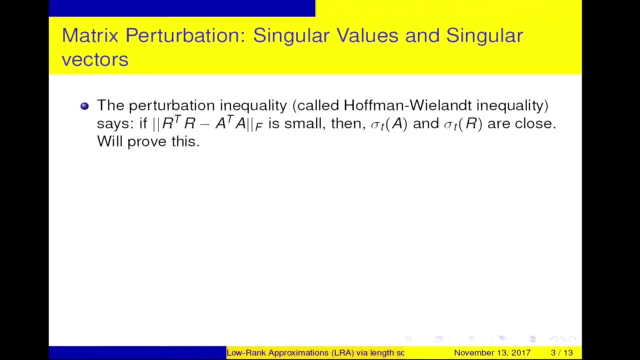 The perturbation inequality we'll use is called the Hoffman-Villan inequality, Which will say that if R transpose R is close to A transpose A in Frobenius norm, then the singular values of A and R are close. We'll prove that okay. 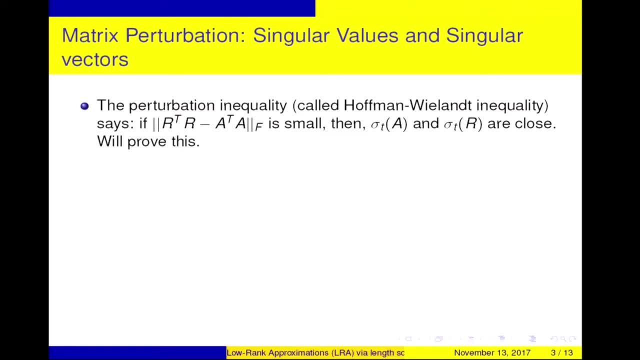 So I've made a small perturbation you can think of of A transpose A. to get R transpose R. If the perturbation is small enough, the singular values don't deviate too much. okay, That sounds very plausible and true, and in fact it's not. but 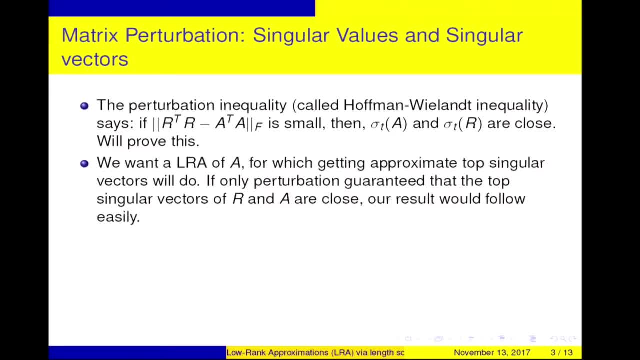 in fact it's true. So now you can ask: what about singular vectors, right? So we really want a low rank approximation of A and that would be possible intuitively if you get a good approximate top singular vectors of A right. 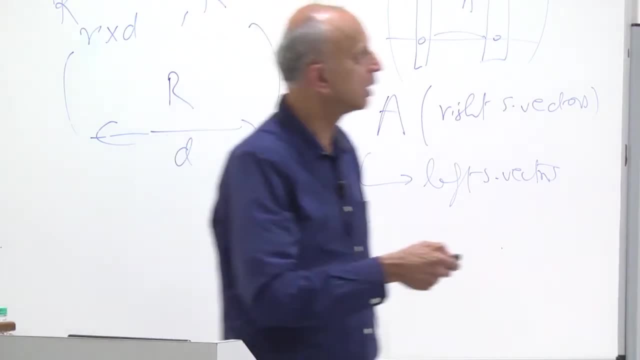 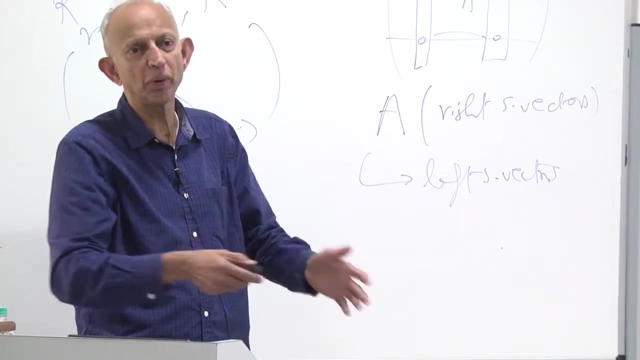 If I get the top few singular vectors- may not be exactly but approximately- that should be good enough to get a good lowering approximation of A. If I get them exactly, I get the best possible. If I get them approximately, I should get it approximately. 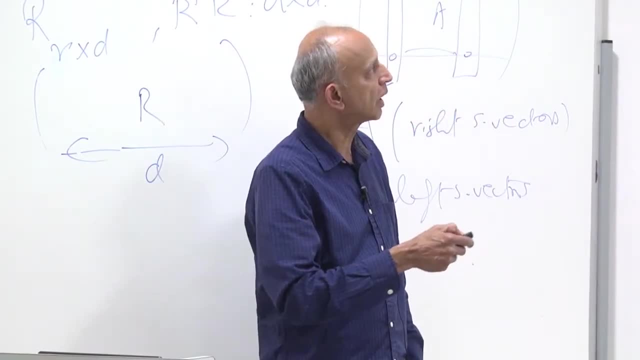 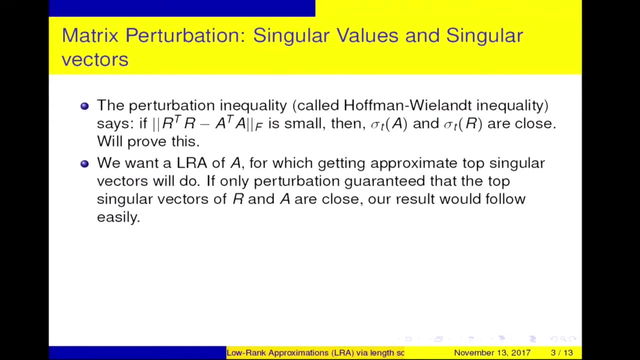 Now if my inequality here- Hoffman-Wieland or any other inequality- actually guaranteed that the top singular vectors of R and A are close, So if this is small would imply that R and A have very close singular vectors, then A will be very simple, right. 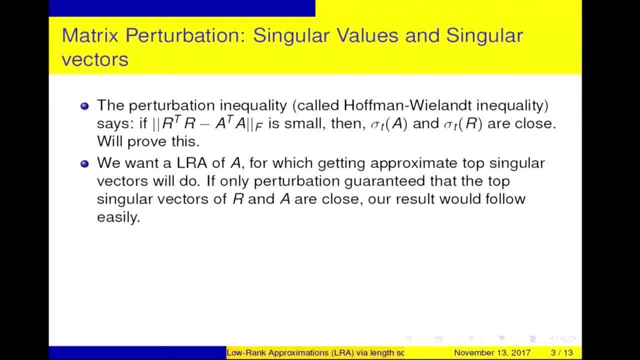 Then that would say: find the singular vectors of R. they are close to singular vectors of A and they give me a good low rank approximation. Okay, unfortunately that's false. this is false right, Even though perturbations don't change singular values too much. 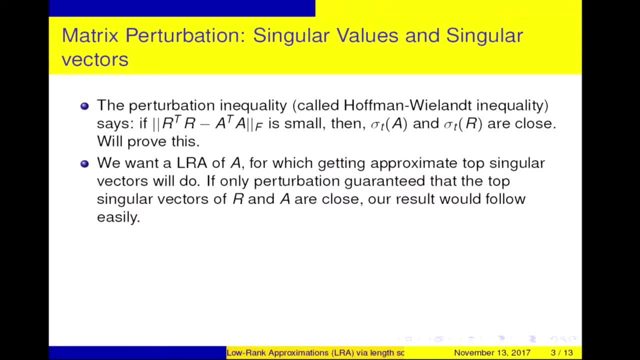 they can completely change singular vectors. okay, Singular vectors are singular. that's maybe one reason to call them singular vectors. singular values are not, So multiple singular vectors are points of discontinuity of singular vectors. that means, like multiple eigenvalues: There are many eigenvectors corresponding to the same eigenvalues. 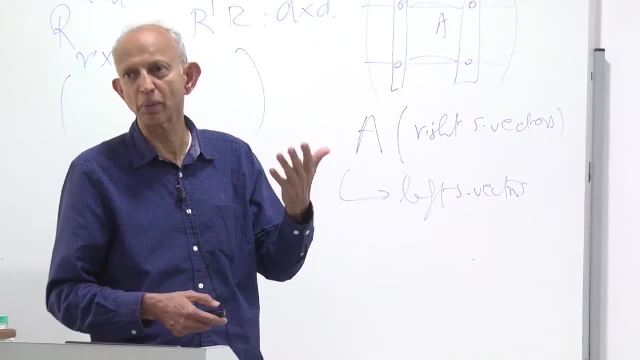 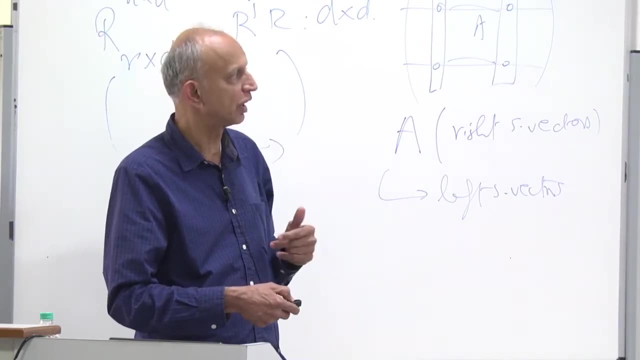 then it's called a multiple eigenvalue. Here's the multiple roots of the polynomial right. Similarly, if you have a singular value that has associated with many singular vectors, then there's a discontinuity. I'll elaborate, but I'll give you an example first. 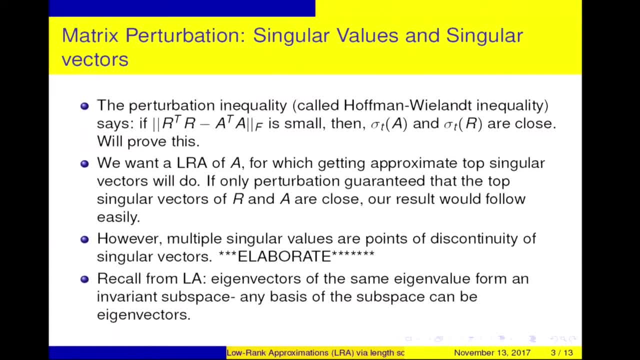 But before all that, please do recall from linear algebra that if you had ties for, say, eigenvalues, you have a bunch of eigenvectors. they form an invariant subspace And I could have chosen in linear algebra- right, I would choose. any basis of the subspace can be my eigenvectors. 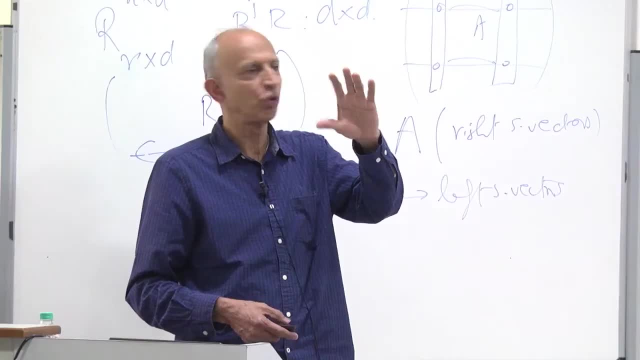 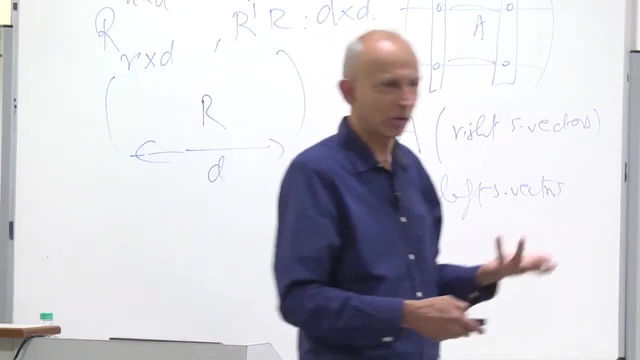 And that's the reason for the discontinuity right. So if you flip things a little bit, you might flip from one basis to another, And so that's a complete flip of the eigenvectors, And the simplest example is this right. 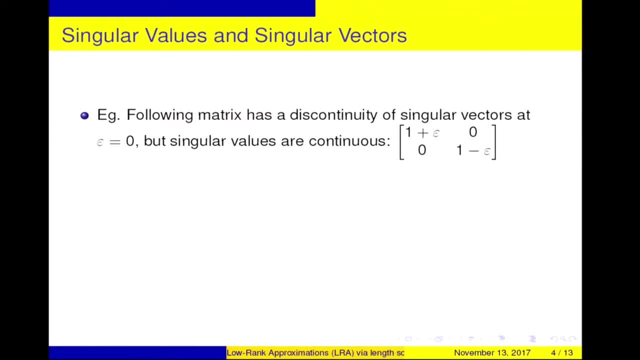 So if I have a matrix 1 plus epsilon, 1 minus epsilon 0,, 0. At epsilon equals 0, there's a discontinuity of the singular vectors, not of the singular values or of the eigenvectors, But not of the eigenvectors. 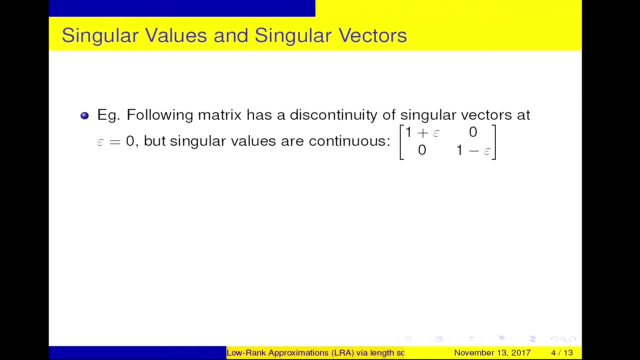 the eigenvalue is continuous at epsilon equals 0,. all right, So it's the eigenvector that's discontinuous, because if epsilon is positive, the eigenvector is the first unit vector, If epsilon is negative, it's the second unit vector. 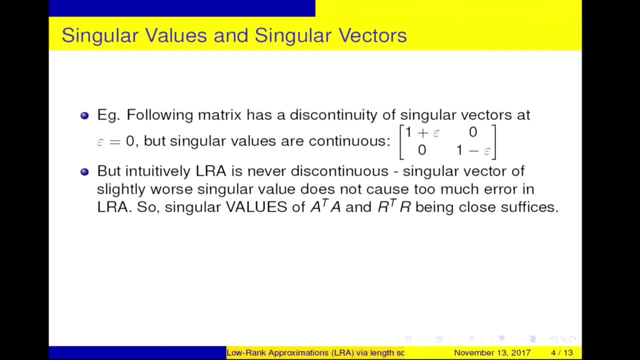 So it flips completely right. So, but the point to remember is that low rank approximation, intuitively, is not discontinuous, right? If I take the singular vector of a slightly worse singular value. so suppose I had this picture and epsilon was positive, right? 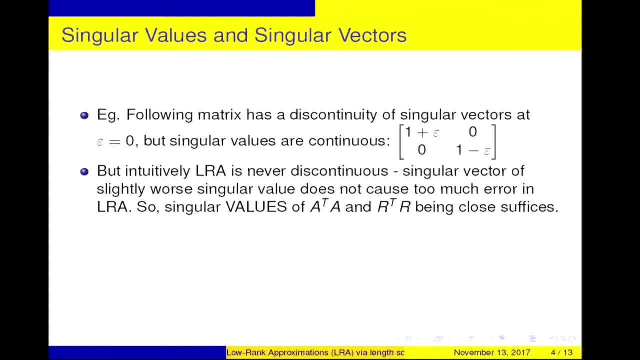 So the eigenvector or the singular vector is the top one. But this is a close by eigenvector with eigenvalue 1 minus epsilon, so 1 plus epsilon. So if I took this vector instead of that intuitively I shouldn't be very far off right in the approximations I get. 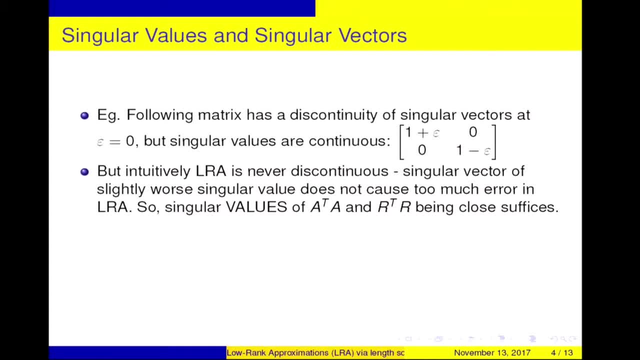 That is true. I am badly off if I want exact eigenvalues. If I want ax equals lambda x. I'm not gonna get it if I took this instead of that, right. But I'm okay if I want just an approximation. 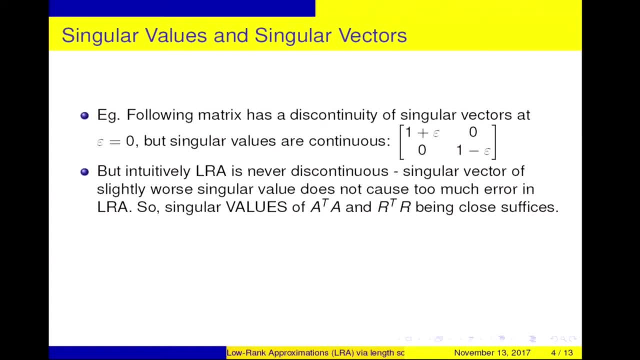 So that's what we'll use, okay, So presumably this point is clear. I'm just recapping, jogging your memory on linear algebra about continuity of eigenvalues. Eigenvalues are continuous, eigenvectors are not. Now, this is just for your information. 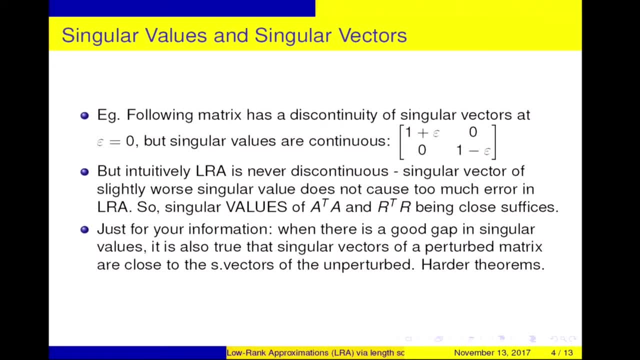 I won't prove this. In fact, it is true that at points I'm not gonna prove this, I'm not gonna prove this. But at points of continuity, at points where this discontinuity does not occur, eigenvectors or singular vectors also behave nicely okay. 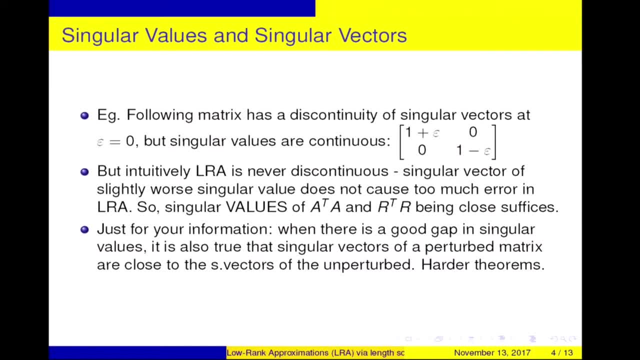 So these are harder theorems. So when there is a good gap in singular values, so discontinuity occurred when two singular values were the same, okay, Preventing that means singular values are quite different. So if there's a gap between successive singular values, 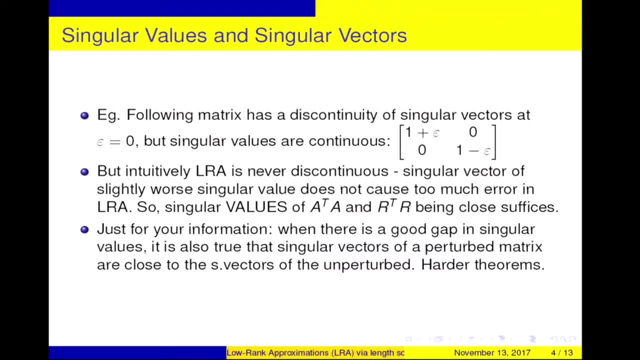 then it's also true that the singular vectors, they behave nicely continuously in a quantified way. So not only continuous, but Lipschitz right, That's what this is saying. Singular vectors, matrix, are close to singular vectors. These are harder theorems, sorry. 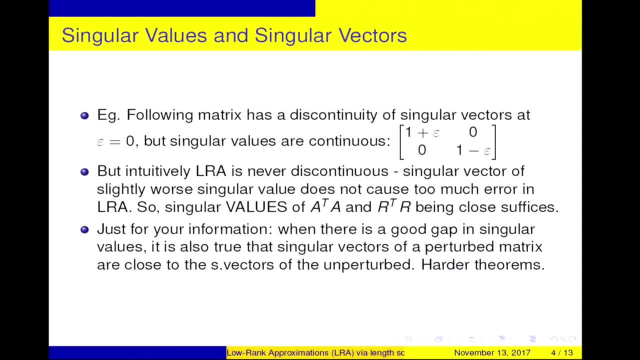 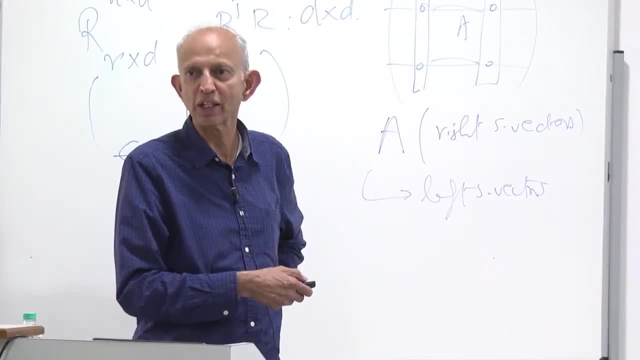 These are called the sine theta theorems or Wadden's theorems. they are due to Wadden, The simplest versions are due to Kahn and they're called the sine theta theorem. If you want to look it up, you can do that. 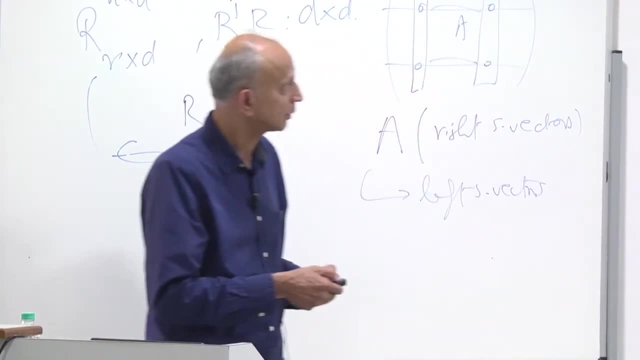 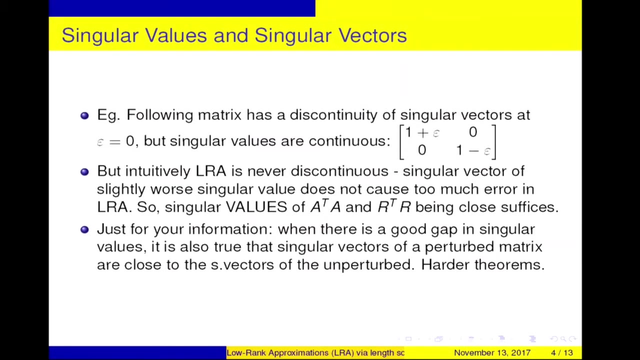 Yeah, again, I won't prove this. We don't need that, right? So we saw that. this says: I don't need these theorems Because low rank approximation I'm okay by. if I missed, I'll buy a little bit the singular value. 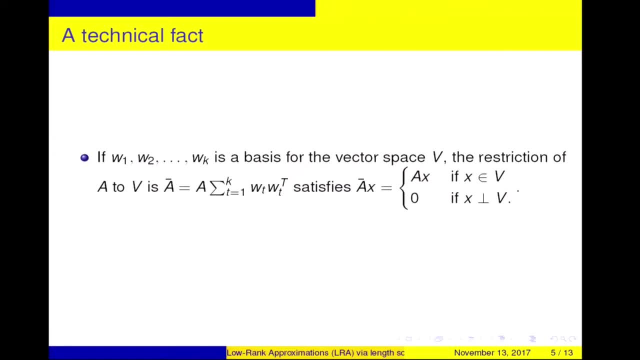 Okay, so just a technical fact. This is just a definition of the restriction of a linear operator or just linear transformation to a space. So if you have a subspace V spanned by this basis- and I'm gonna take a linear transformation here- restricted to 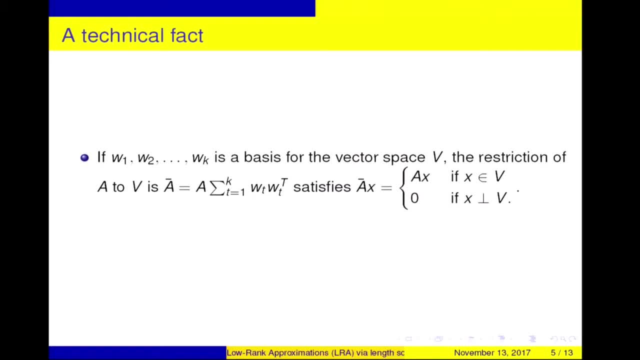 A restricted to V. I just say the restriction is A bar, which is that is restriction in the sense that A bar X is the same as AX if X belongs to V and zero if X is orthogonal to V. Right, And both are quite clear. 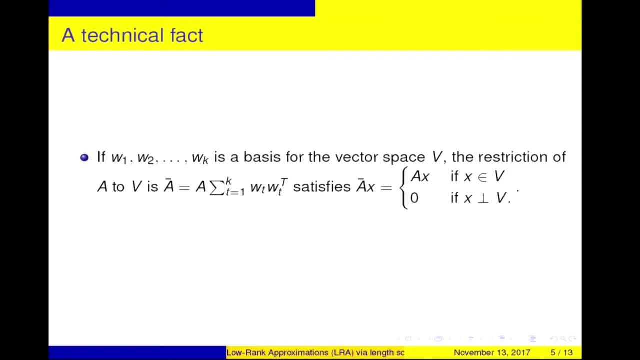 I mean the zero is completely clear. If X is orthogonal to the space V, it's orthogonal to all these Ws. so it's zero. And the first one is just: yes, just a little manipulation, right? So we have a bar x now. x belongs to the space. 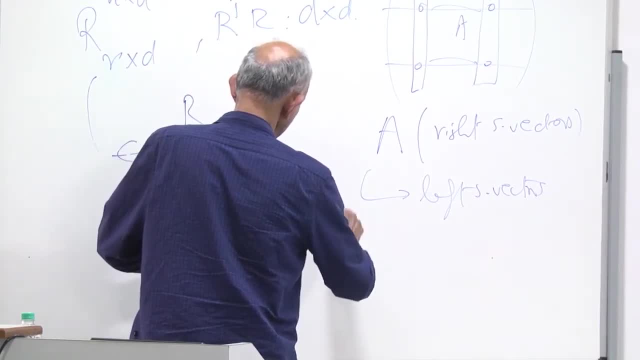 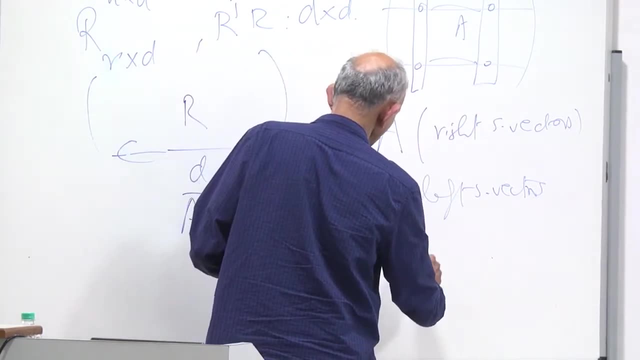 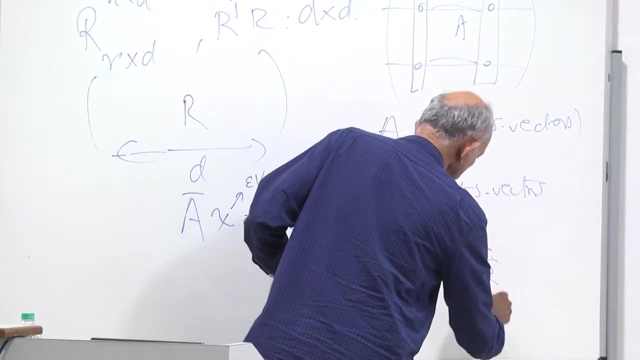 So x can itself be written as sum of alpha t, w, t. And then you write, you expand out a bar and you get- you've done things like this before- Times this quantity right, I'm going to put a t prime here, alpha t prime, w t prime. 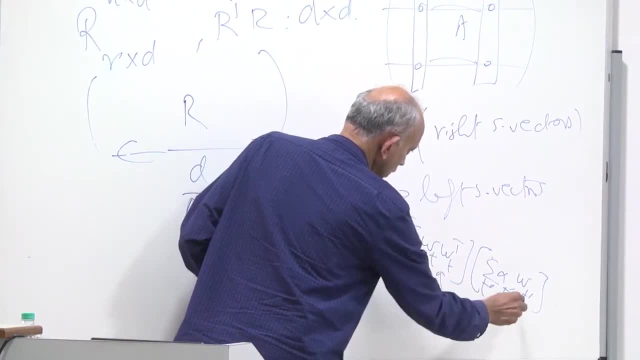 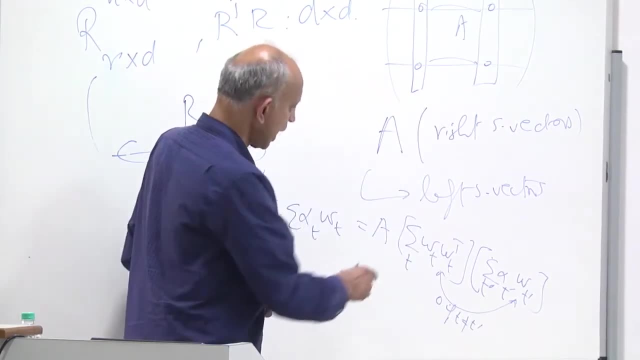 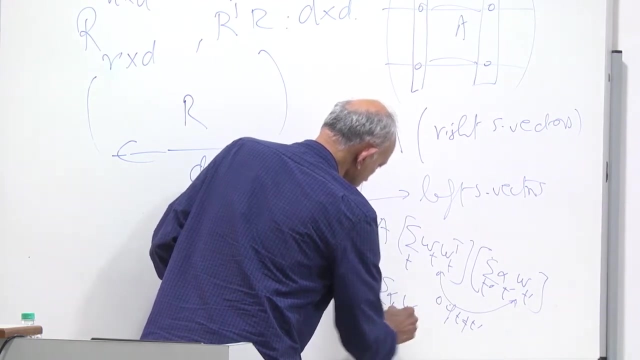 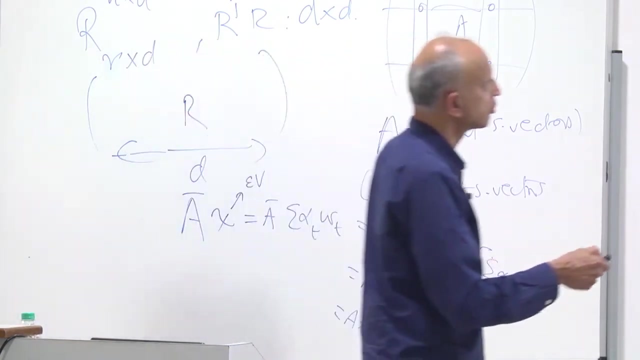 And you see that these are all zero unless t equals t prime. So those terms go away and only the terms that w2 remains. so then you just get alpha t, w, t, And that's equal to a. Okay, so restriction just means. 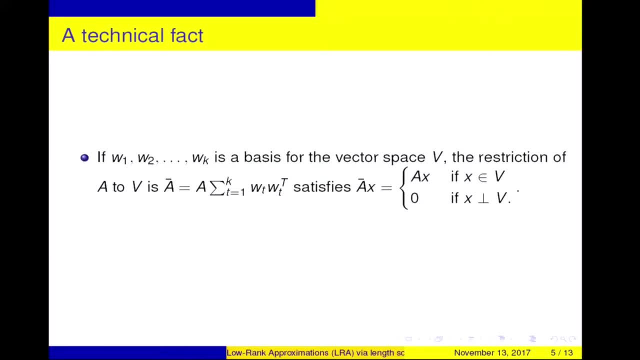 It does what a does in the subspace: orthogonal, just zeroes out, orthogonal to another space. Okay, now the statement of the main theorem. So we'll state the main theorem, which is, as I said, purely a matrix perturbation result, and then we'll prove it. 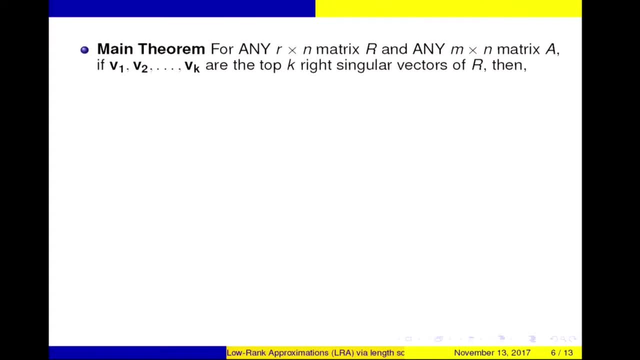 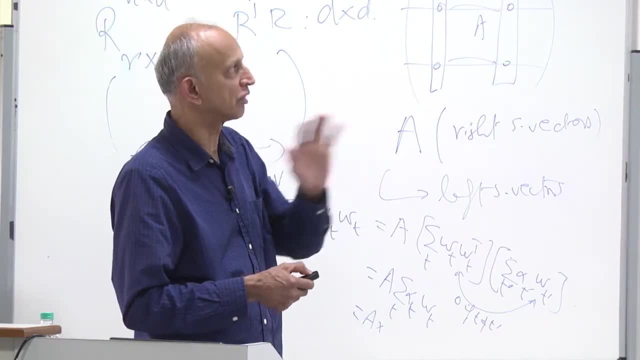 So now, r is not necessarily length squared sample, it's just any matrix which is r by n. It is not even a sub-matrix necessarily, right? R has no relation to a. okay, So it's for every pair of matrices, r and a, it's just a and. 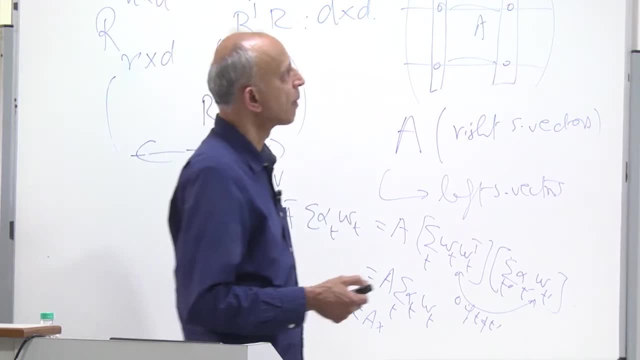 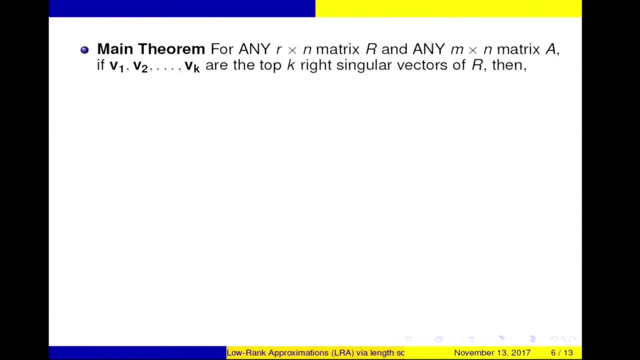 it just applies as long as the n is the same right. So if v1 through vk or the top k right. singular vectors of r. So I want to say, if I found the right singular vectors of r, that gives me a good approximation to a okay. 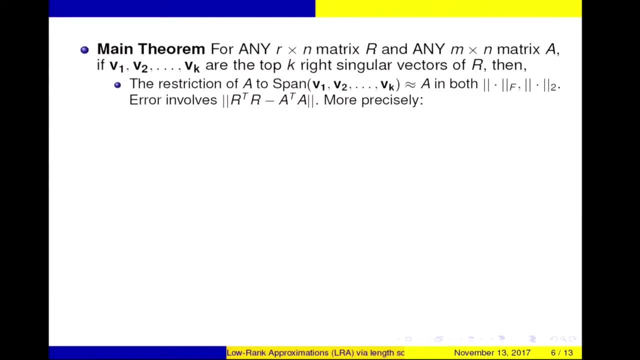 Then the assertion is: conclusion is: the restriction of a to the span of this is approximately a in both Frobenius and spectral norm. Of course that won't be true for all r. r can be arbitrary, But the error involves how different r is from a in this. 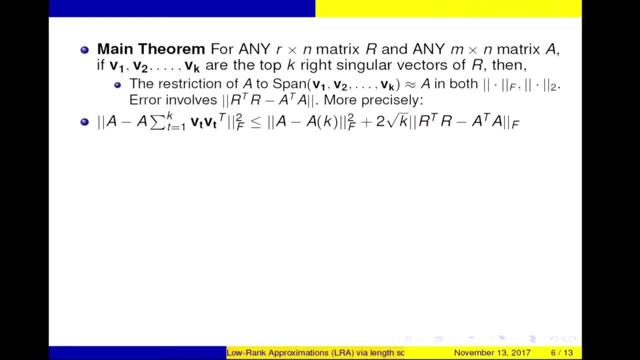 sense, and here's a precise statement, two precise statements. so spectral intravenous norm. So let's go over these. so I should say that. So I take a this from the last slide: is the restriction is that thing, is the restriction of a to the span of. 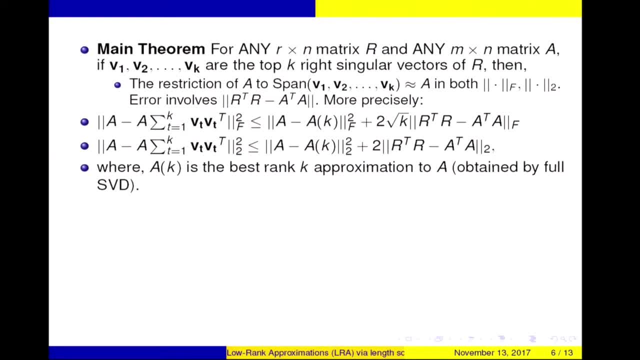 that that's written verbally, right? This is in symbols. that's what the last slide said, right? Okay, in Frobenius norm that's less than or equal to a minus ak. Frobenius norm squared Now ak. I'm sorry, I used a slightly different notation last. 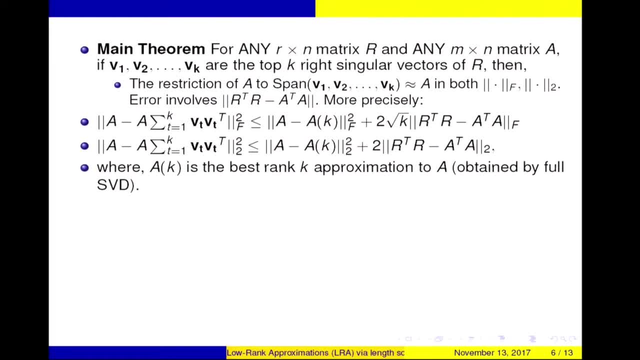 time I said a sub k, but this is also just the best rank k approximation to a, which we saw last lecture, obtained by SVD right. So the best you can do. you cannot do better than that right. you'll be worse by a little bit and 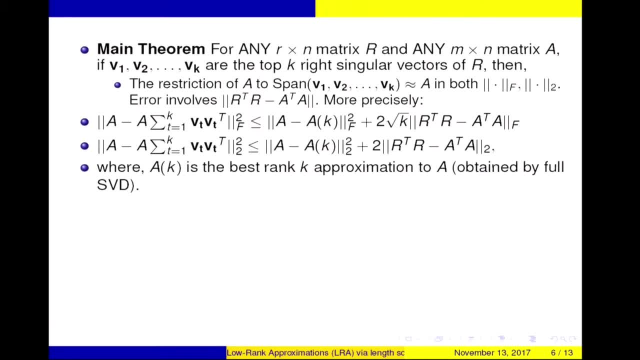 the little bit is root k A times the Frobenius norm of that. okay, So just make sure the scale's balanced. I take the square of the Frobenius norm of a and this is like the square right. I've taken a. transpose a. 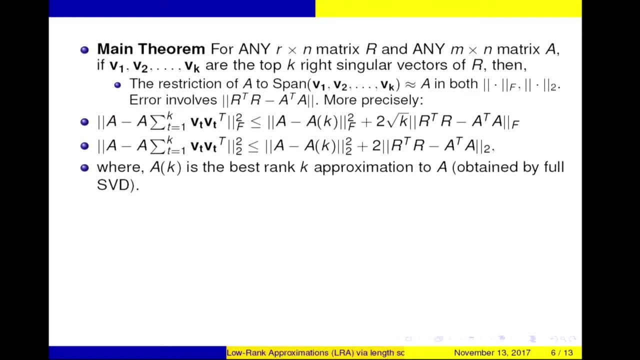 So the dimension's balanced right, just okay. So that's statement number one, and also in spectral norm. this is the best possible because, again, SVD was the best you could do In spectral norm and the error does not have a root k. 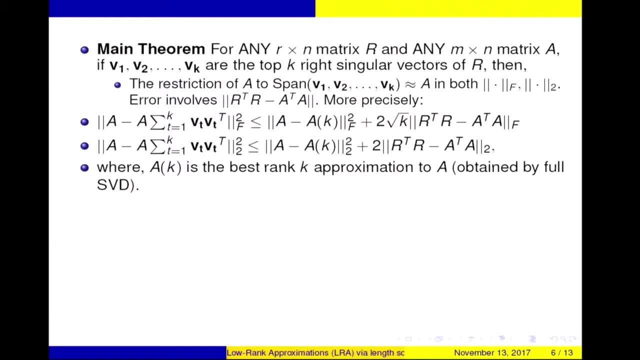 It has just the spectral norm there also Not Frobenius, but spectral. So both of these are spectral norms in this case. So again, this is repeating what I said: A minus ak squared is the best possible error with exact SVD. 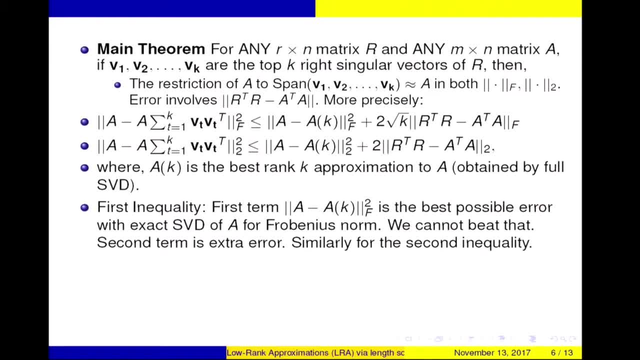 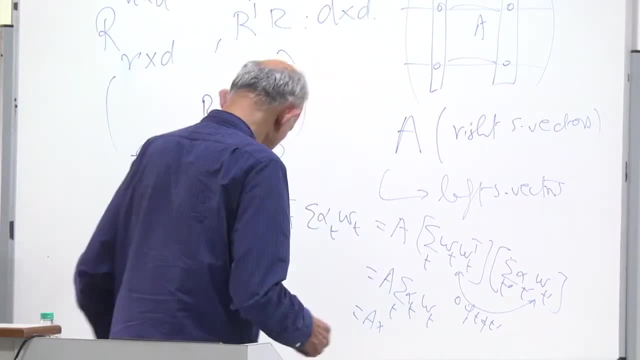 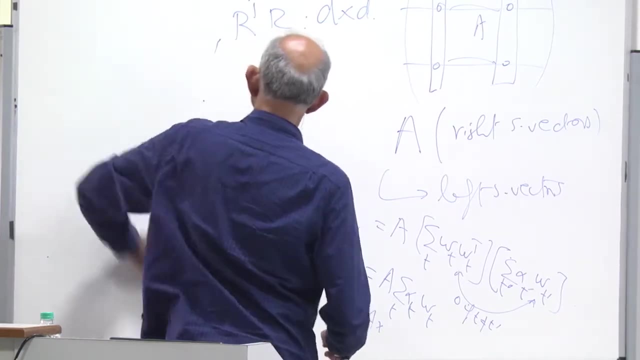 We cannot beat that. that's the best we can do right, And This second term is the error. that's a little bit more Okay and we get that Now. one note: I should have said perhaps, said I should have put it on the slide maybe, but I can tell you. 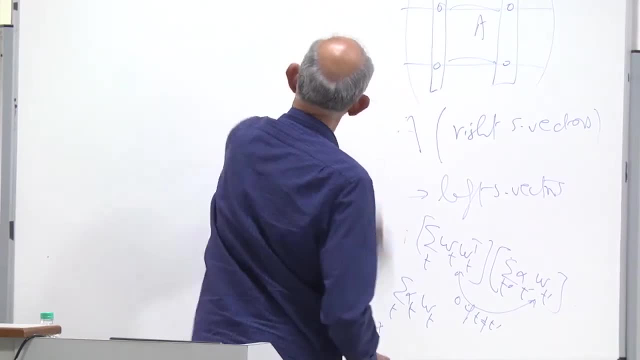 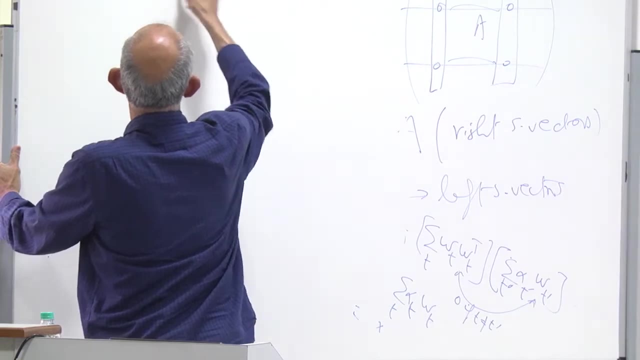 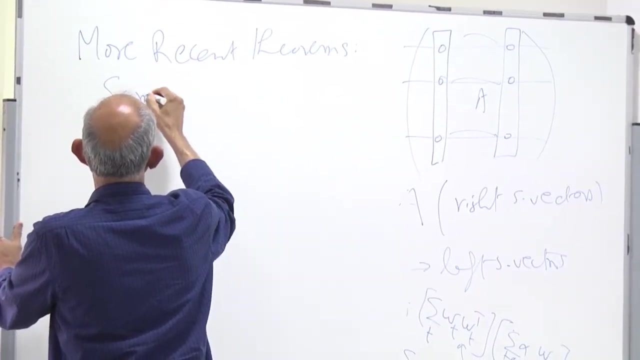 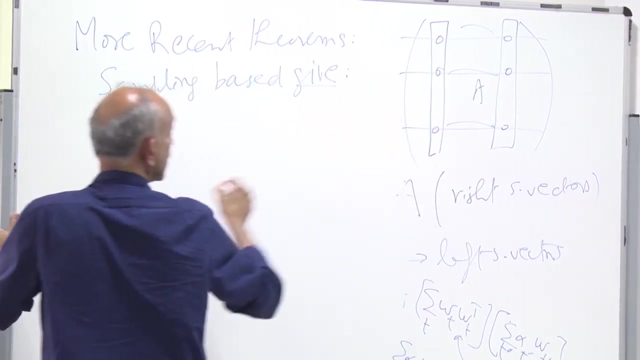 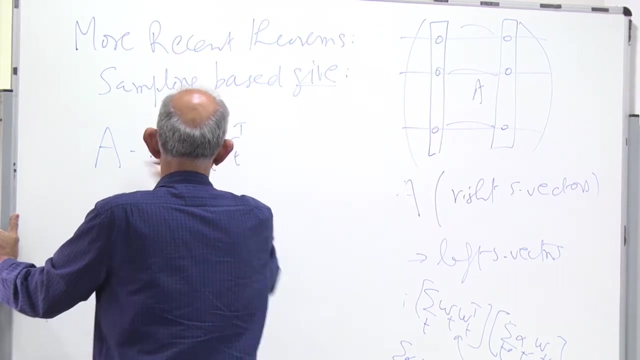 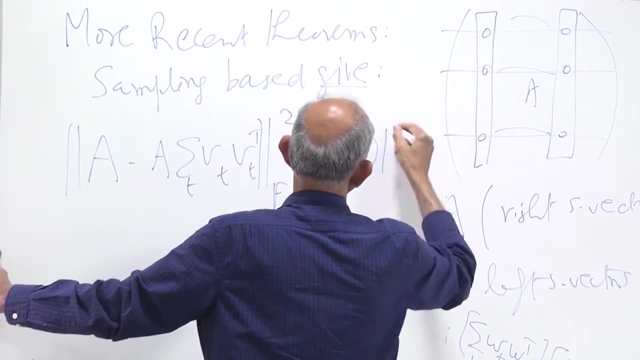 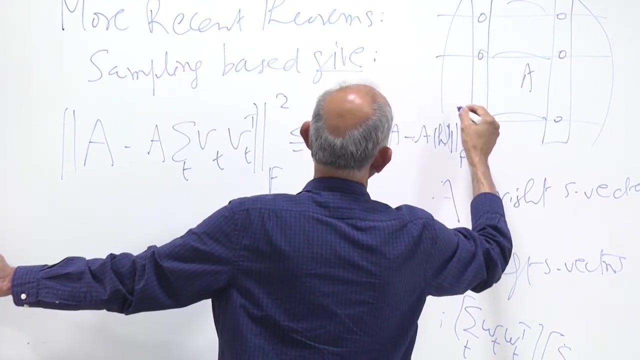 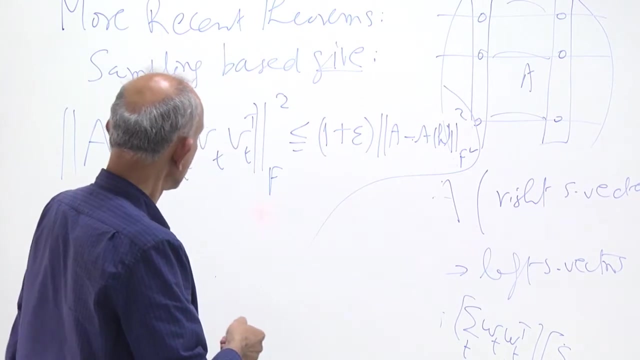 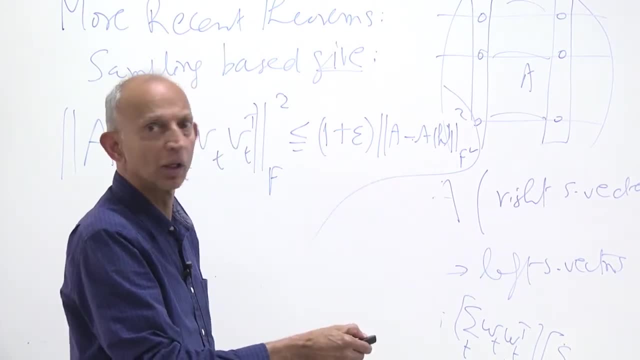 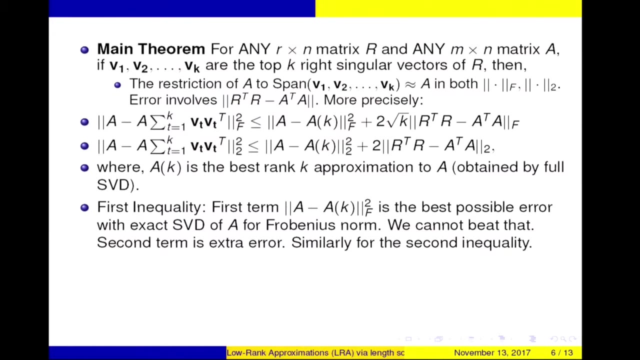 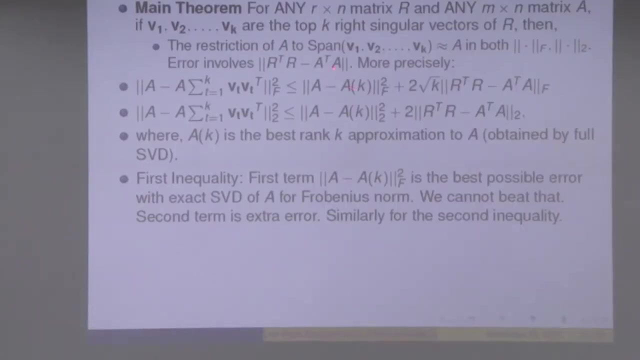 Because so a minus ak right, If you were going to use principal component analysis, for instance, this would be hopefully very small, So you would use it for matrices which are very close to being rank k, okay. So if this is very small, this may be actually much bigger. 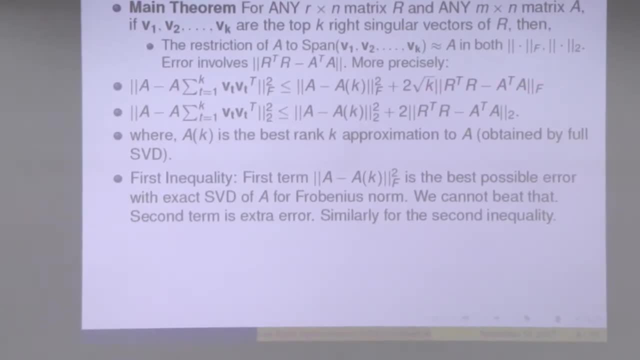 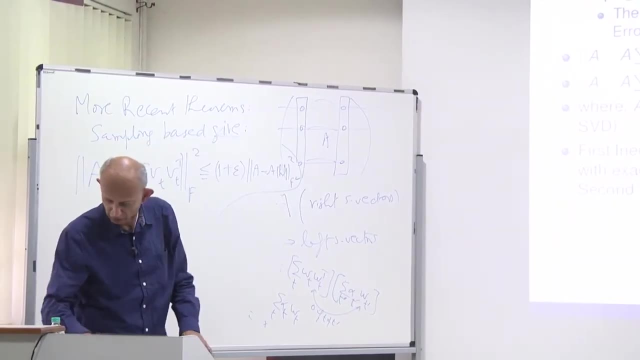 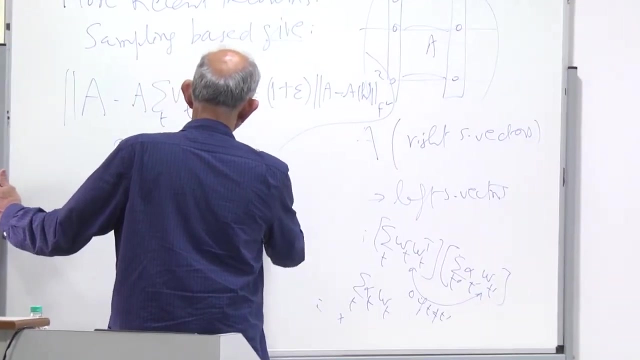 So this error term is pretty big if you did length squared sampling. There are more complicated sampling schemes for which you can actually show these things, which are called relative error bounds, because the error is relative, And so I have a survey paper in which I 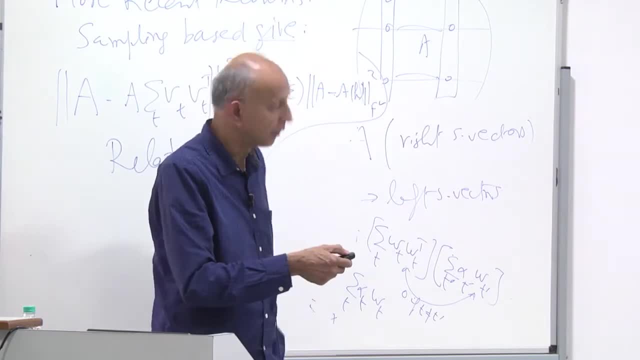 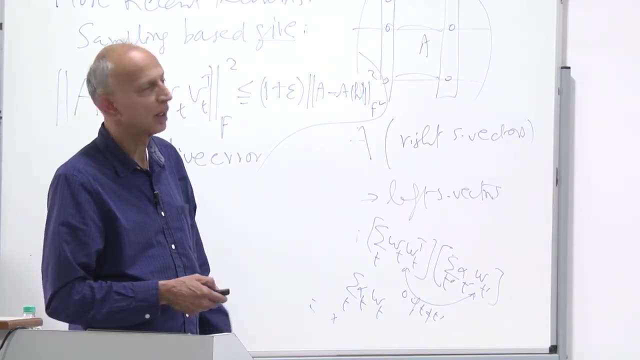 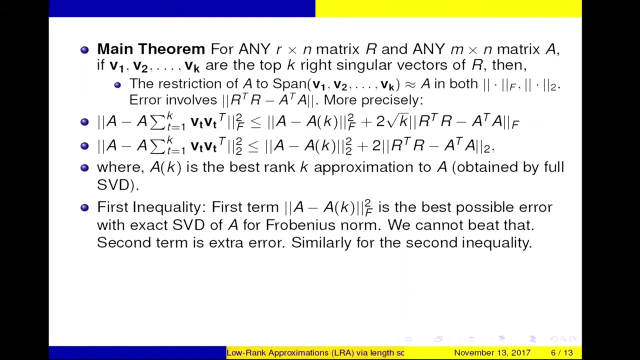 also have these things. But we'll only prove this right. We'll only prove with this absolute error. I can give you references to this. So again, this is how far you're worse off than the best you can do, okay. 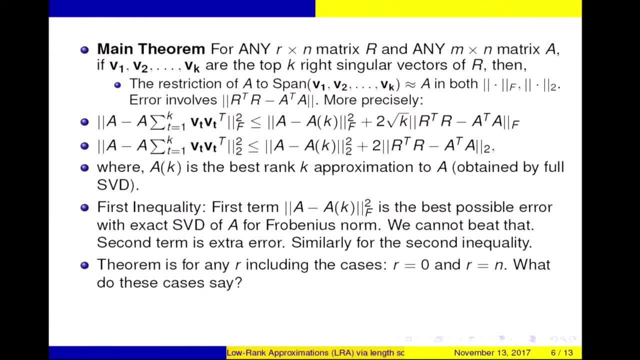 Now one thing that's instructive, before we leave the statement of the theorem and go to the proof: is: the theorem is also true for any r. It's true in particular for r equals 0 and n. It'll be nice to see what you know, what the you know what's. 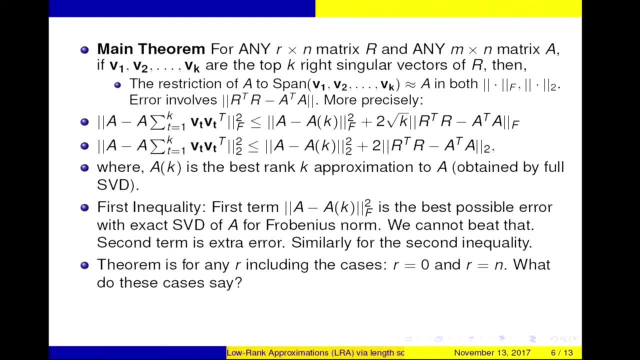 they say to us: What does r equals 0 say? That means I pick no rows in r either. probabilistically other way, I pick no rows, So r transpose: r is 0, right, So this is 0 and there's no Vs. 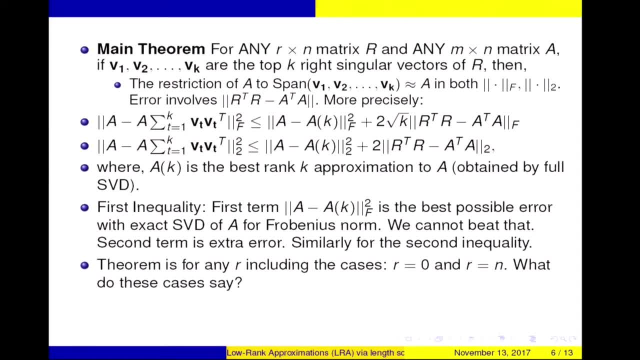 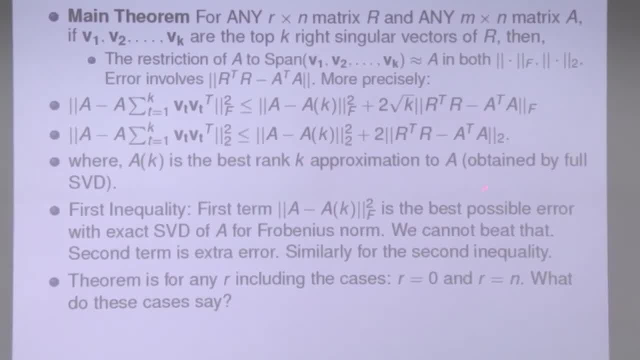 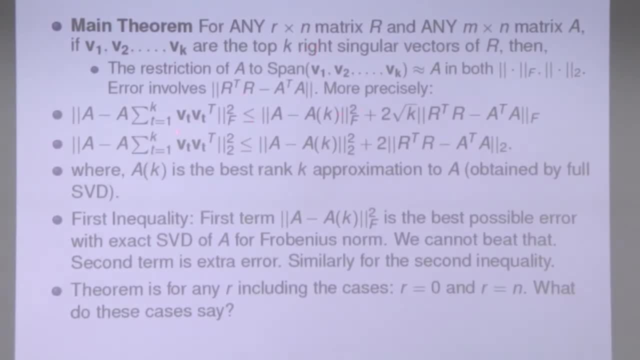 So this is also 0.. So you get a squared right. I should have said excuse me. So I should have said No, I'm sorry. this is true for all k, So I could back off a minute. 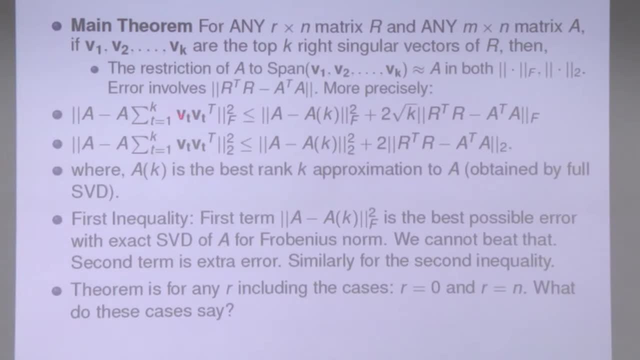 So if r is 0, then there's no singular vector. All of these are 0. So you get af squared here. you get af squared plus a little bit more. this is positive, right? So that's okay. it's not saying very much. 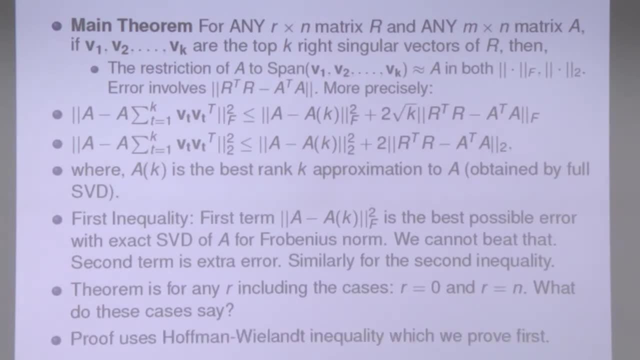 You don't expect it to say very much. What about r equals n? that's also an interesting case. I meant to say r equals d. I meant to say all the rows, okay, So r equals the total number of rows of a. 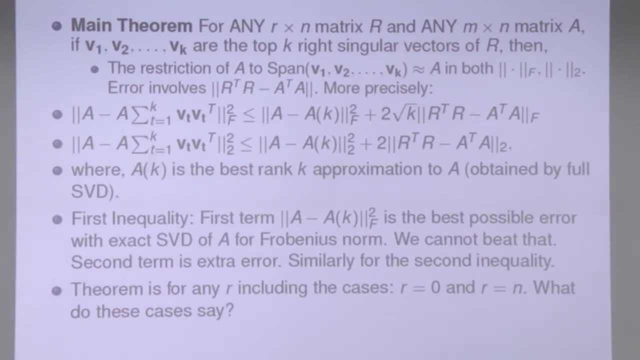 What's a possible r? then A possible r is all of a. So, if r is all of a, this is 0, and this is 0,, right? So still, we are just saying 0, less than or equal to that. 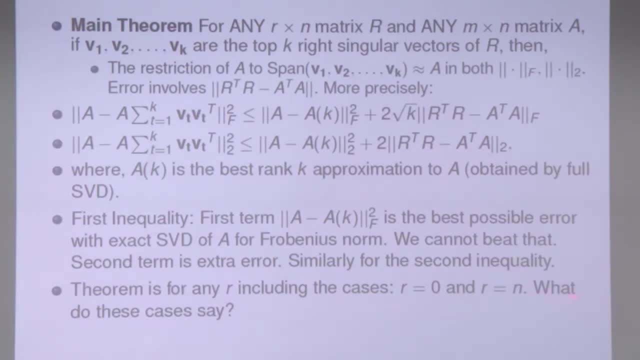 I'm just saying these things as a sanity check. if r equals 0 and n is still true, But they won't be saying anything interesting. It's for other values of r that you expect this. The proof will use the Hoffman-Wheeler inequality. 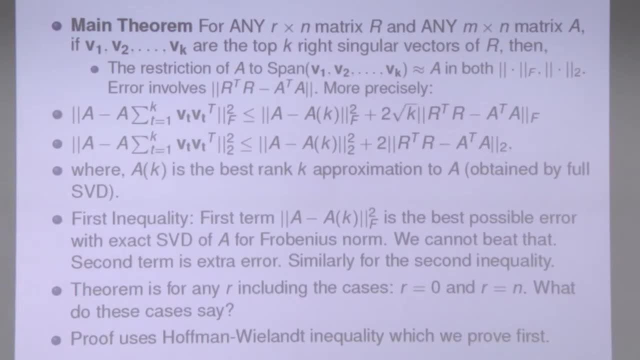 which I'll prove first. I'm gonna spend a little bit of time proving that. There are many proofs of that and this, I think, is one of the simplest. We'll have to do a little bit of combinatorics here, but we'll prove that. 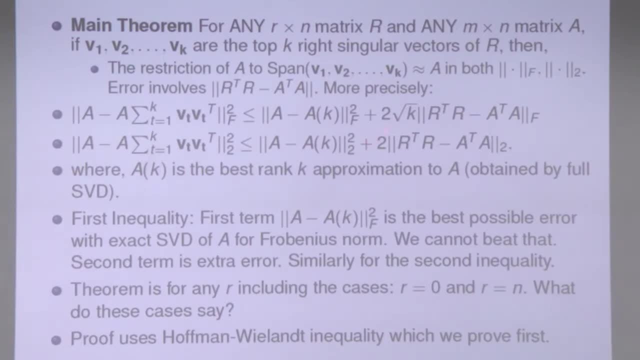 And then I'll go back to proving this. okay, So the model of the story is: for any r, you get a decent approximation of spectral and n- Okay. so for this I need some technical results for the Hoffman-Wheeler inequality. 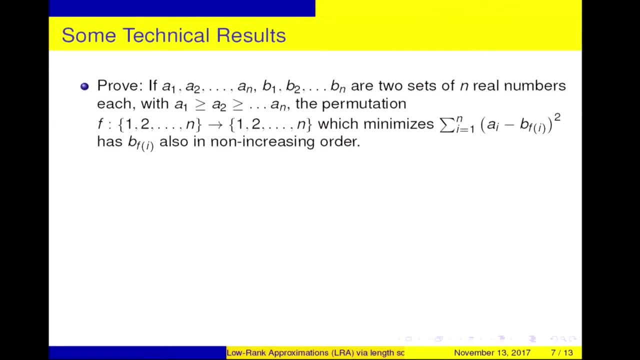 So you have two sets of real numbers: a1 to an, b1 to bn. These are going to be singular values of the two matrices, but later. right now they're just real numbers And the a's are in decreasing order. then the assertion is: 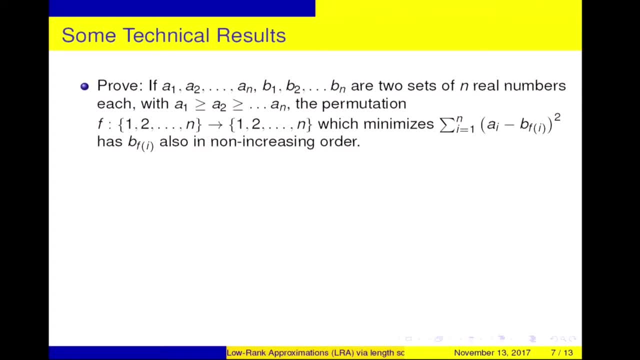 the permutation that minimizes the difference between ai and the B at the permuted spot. So I'm allowed to permute b in any way and I want to minimize this right So intuitively. it's obvious that the best I should be able to do. 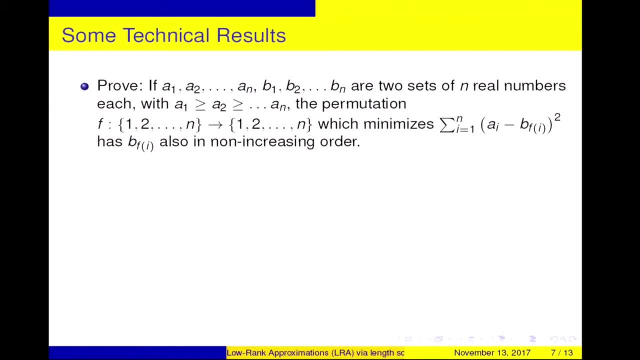 to minimize, that is, also bring b's in decreasing order. Because a's are in decreasing order, If b's are also in decreasing order, you would expect that to be minimized, right? So usually the proofs of these are all very simple and here is the proof usually for such a statement. 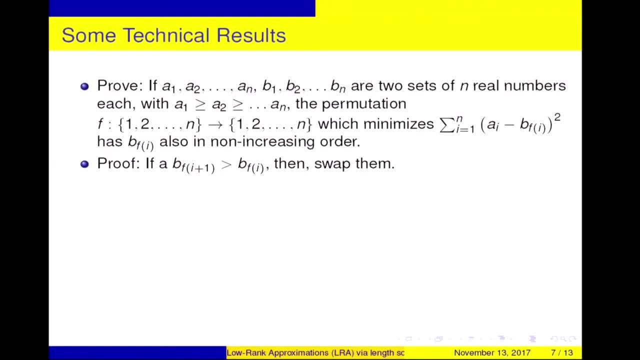 this statement is: if B was not in decreasing order, so let's say the I plus first. if they're not in decreasing order, there must be adjacent ones which are in bad order. right? If B was not sorted, there's a pair that's adjacent, not sorted. 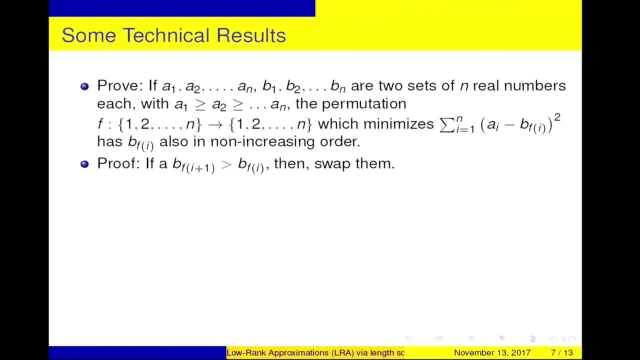 So you have that, and if you just swap you'll improve. So you can check that. so it's just a simple check. okay, Now we have to use another nice theorem called Burkhoff's Theorem. that says: every doubly stochastic matrix can be written as: 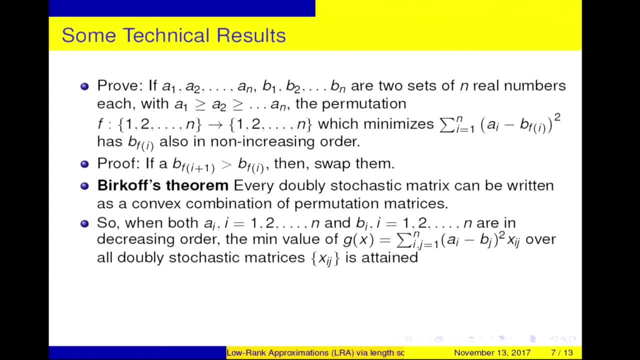 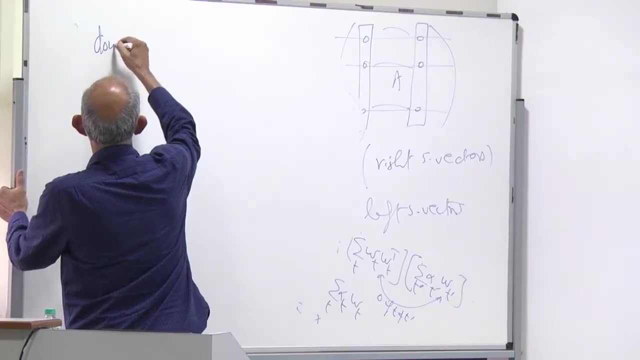 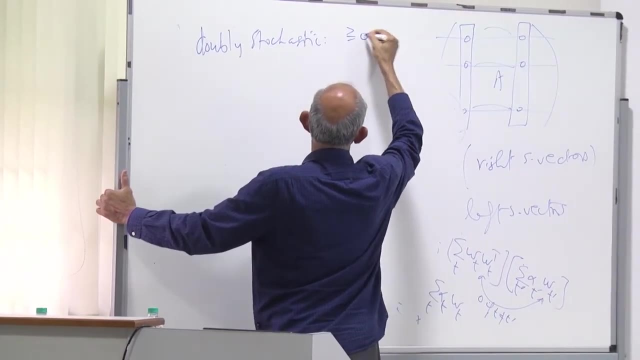 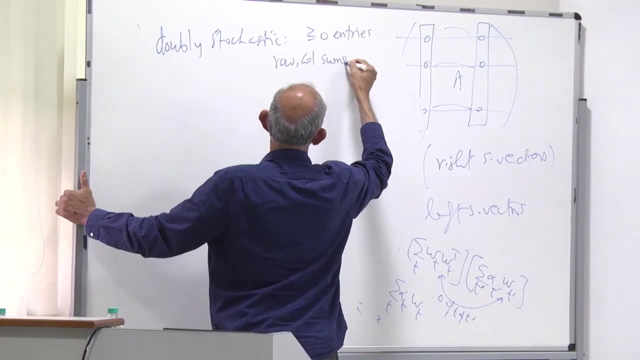 a convex combination of permutation matrices. Did I define that? No, I didn't define those terms, so maybe I should just recall those terms. So doubly stochastic means non-negative entries. all row and column sums are a one, All of them. 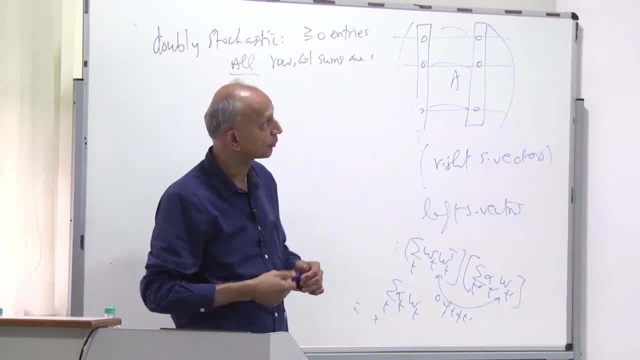 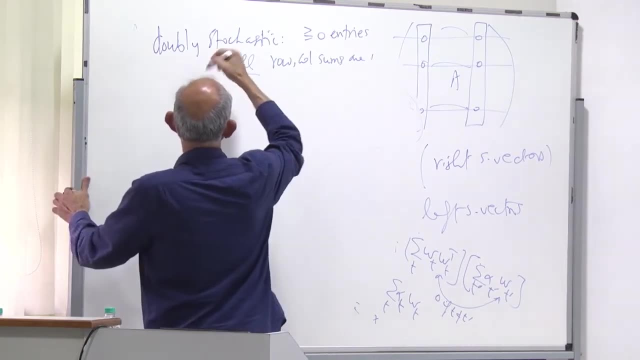 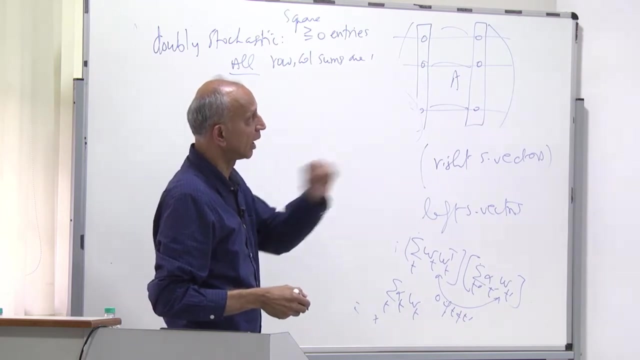 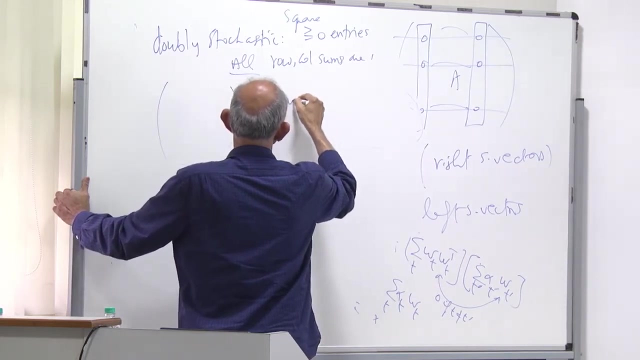 So a matrix with this property is called doubly stochastic, okay, And square also, I should say. I guess doesn't follow right. And then the term permutation matrix just means it's permutation matrix is just called 1, 1 permutation matrix. 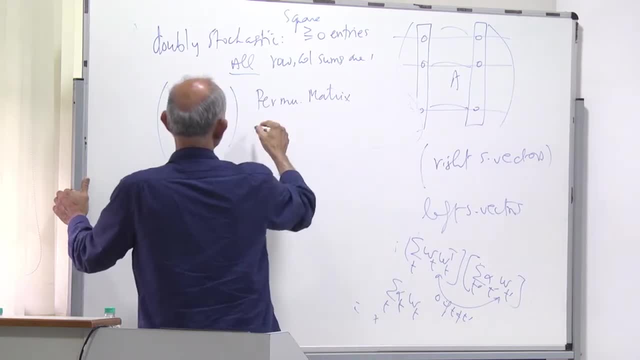 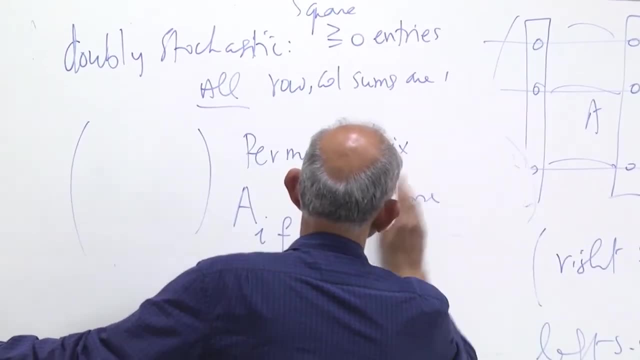 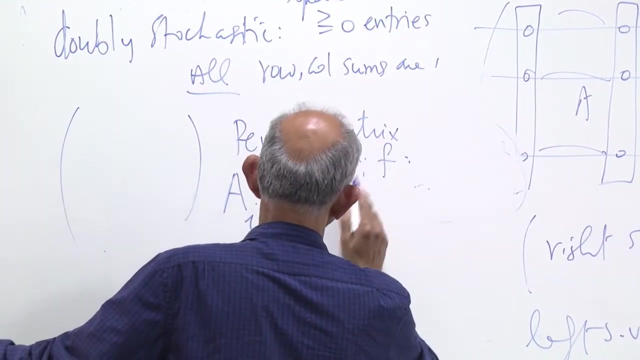 If there's a permutation right. So a i fi equals 1, for some permutation f. I should say there exists a permutation f, so I said this is 1, and equal to 0 for all other entries. Okay, Okay. 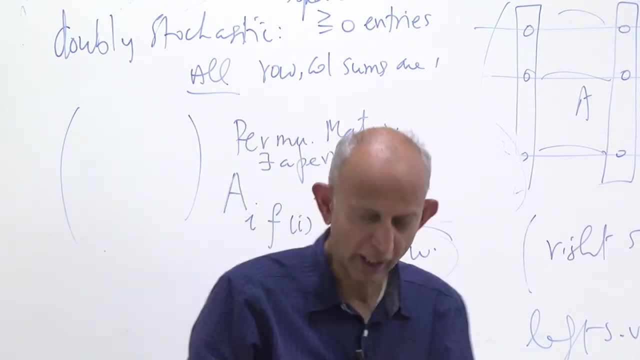 Go ahead, Okay. Okay, It's a diagonal matrix or any permutation. There are a lot of. So says every W stochastic matrix can be written as a combination of permutation matrix. I won't prove that, but I'll just assume that. 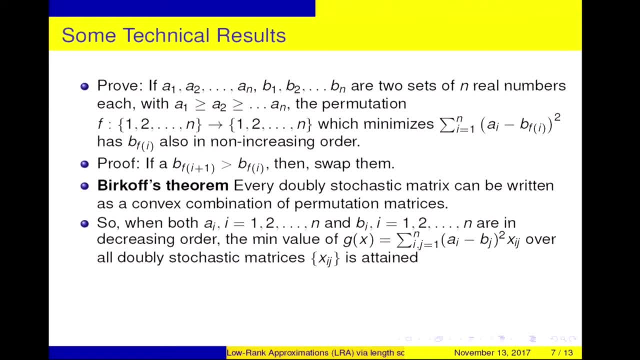 So when Ai and Bi now are both in decreasing order according to this right, The minimum value of this quantity Ai-Bi squared- Sorry, Ai-Bj squared xij- I'm gonna try to minimize that over all x's which are W. 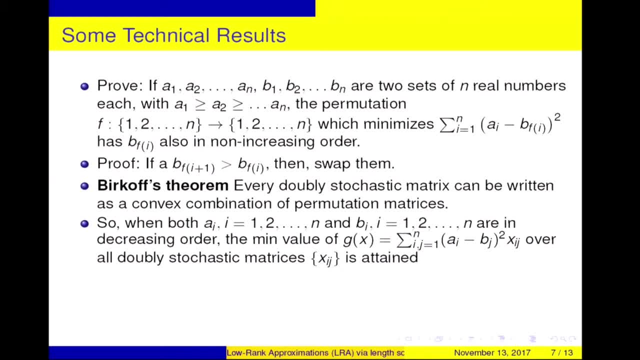 stochastic which form a W stochastic matrix right Is attained at a permutation matrix first. So why is that? Why is the minimum attained at a permutation matrix? Because of the convex combination right. So if the minimum is attained at some W stochastic matrix, 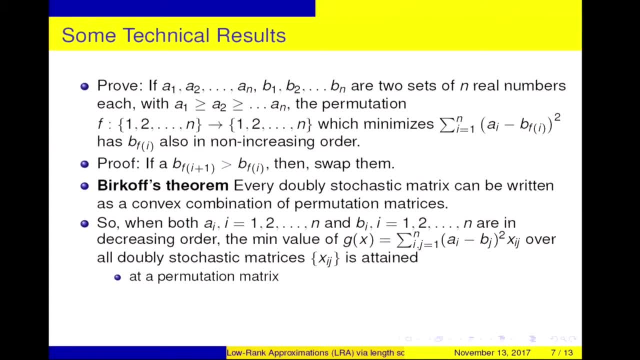 you can always write it as a convex combination of permutation matrices and there's a linear function in the xij, So it should be attained at one of the permutation matrices. And secondly, since the identity permutation is the min over all permutations, this is attained by the identity right. 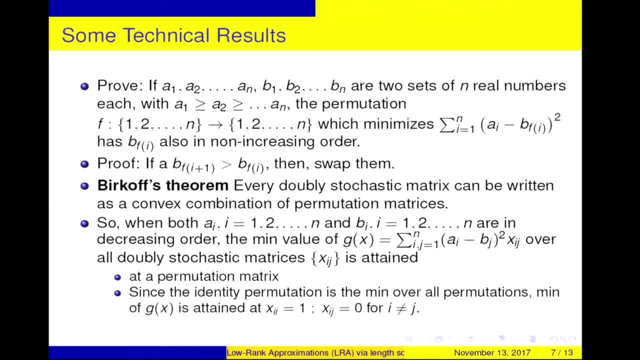 So we saw that the permutation that minimizes is the identity. that was this part, And this says that over all stochastic matrices, the minimum is attained at a permutation matrix must be the identity. okay, So we'll come back. we could use this in the next slide, but 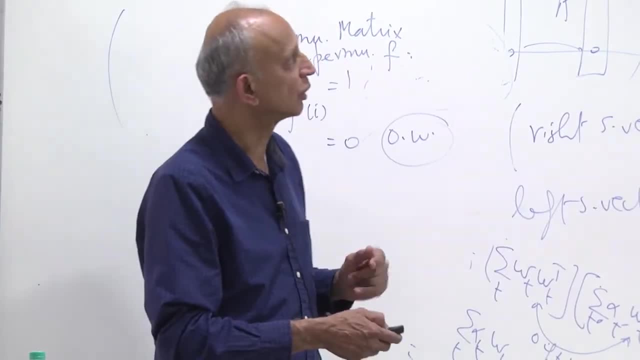 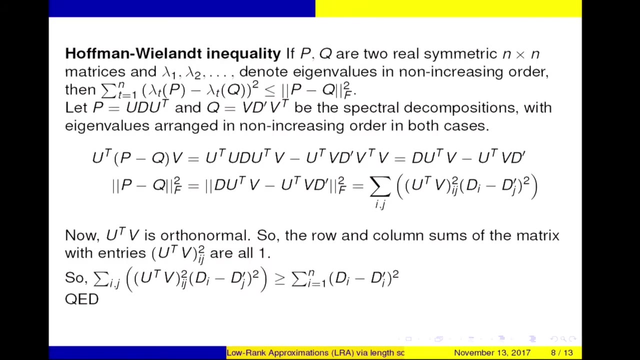 I may have to come back and recall this for you. So now Hoffman-Veland. I guess I don't have it. I have it all displayed one shot. This is the proof of Hoffman-Veland. now that we have all that, 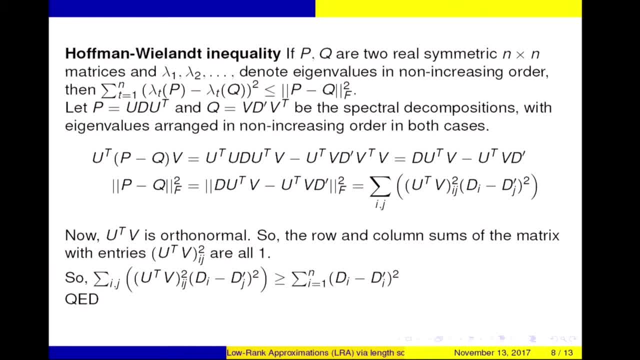 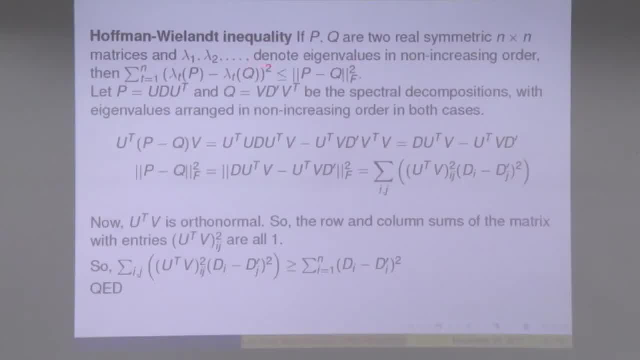 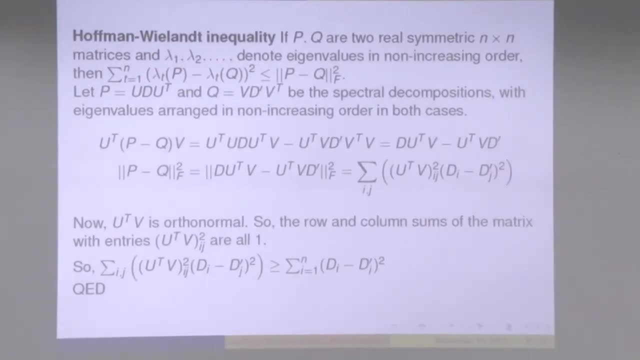 So if you have two real symmetric matrices with lambdas of the eigenvalues- I've arranged lambdas of both matrices in decreasing, in non-increasing order- Then the assertion is the lambdas are close, right Provided p and q are close. 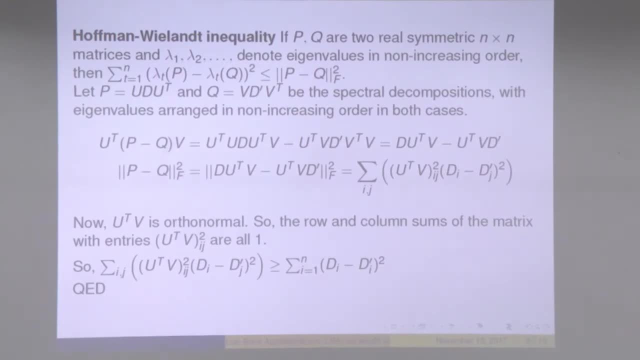 So if p and q are close, the lambdas are close, right, The eigenvalues are close Again. this is continuity of eigenvalues. Eigenvectors are not continuous right? So I'm going to come back to that. 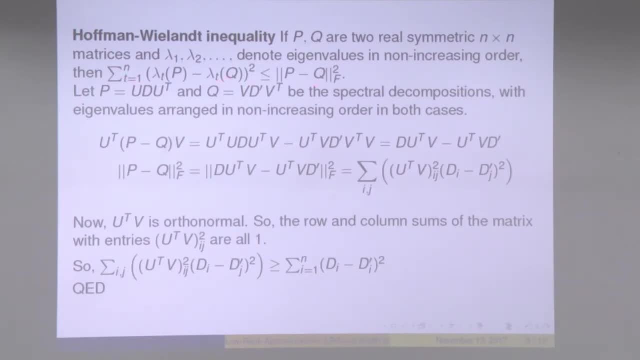 You take the sum of squares of all these things, That's less than or equal to the Frobenius norm of the difference between p and q. okay, So how do we prove that? So I'm going to go over- I mean while going over this, 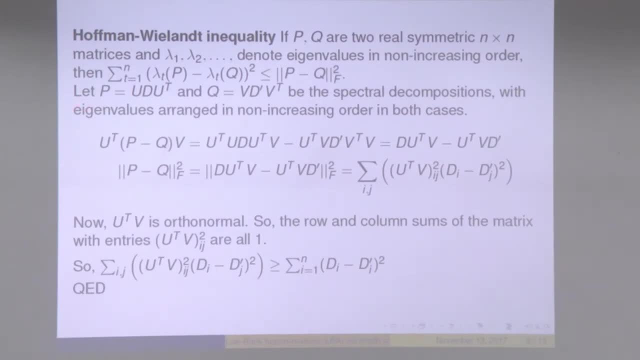 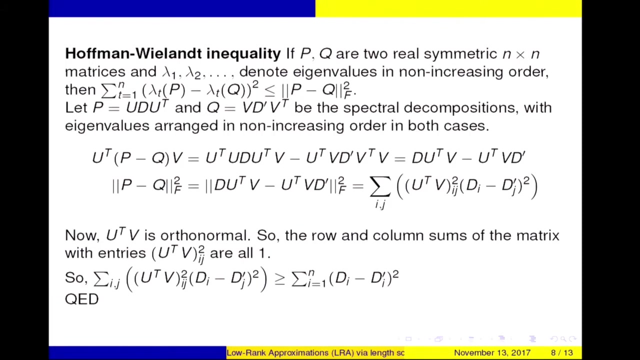 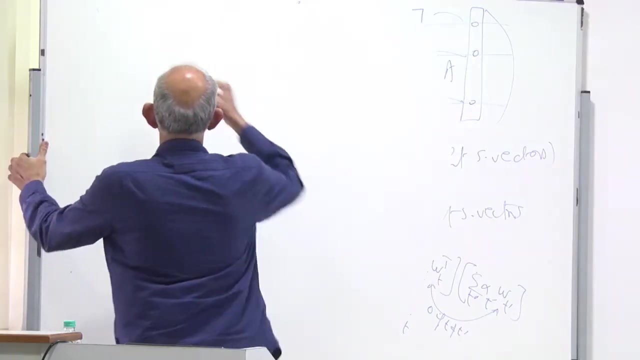 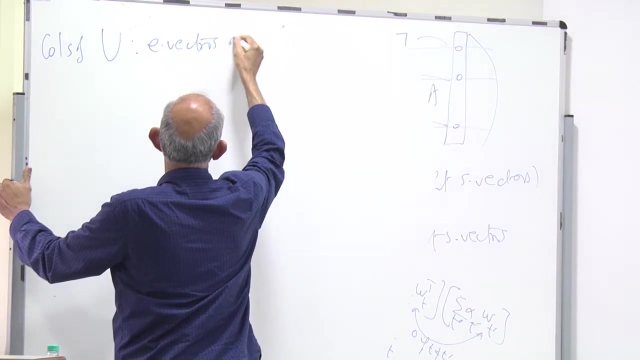 we'll recap some linear algebra as we go along. So I'm gonna write p as u du transpose, and this is v d prime, v transpose. These are spectral decompositions. And just to recall, So u columns of u are eigenvectors of p. 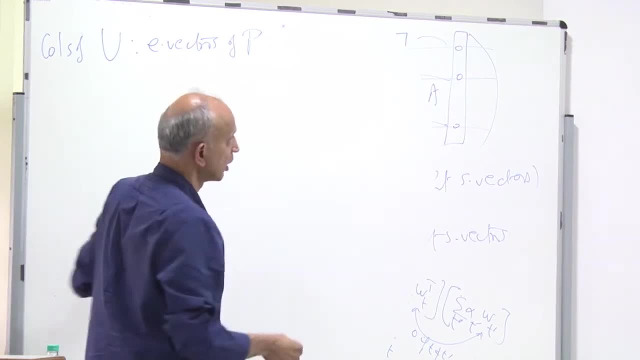 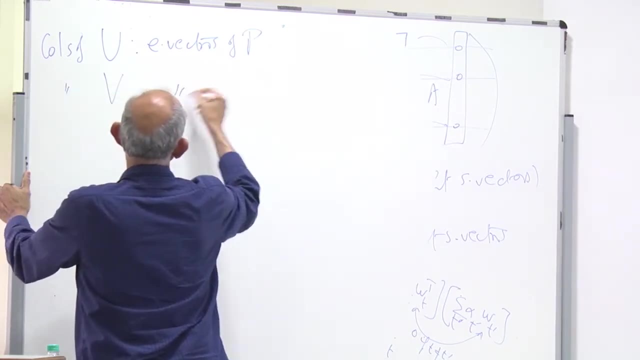 The p and q are symmetric right Eigenvectors of p, so they are spectral decompositions here, right. So and v is columns of v and v is columns of v And v is columns of p, or the eigenvectors of q and u. 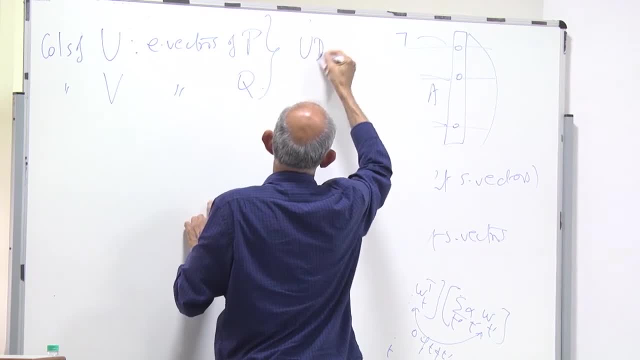 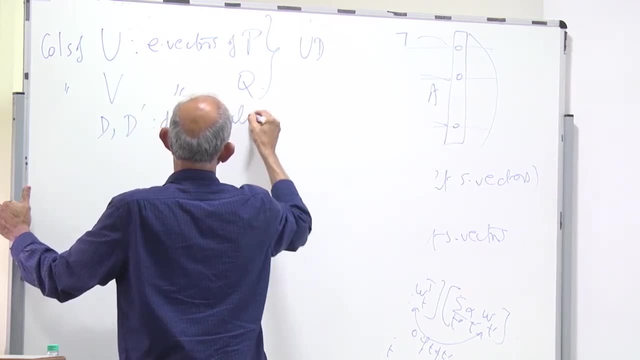 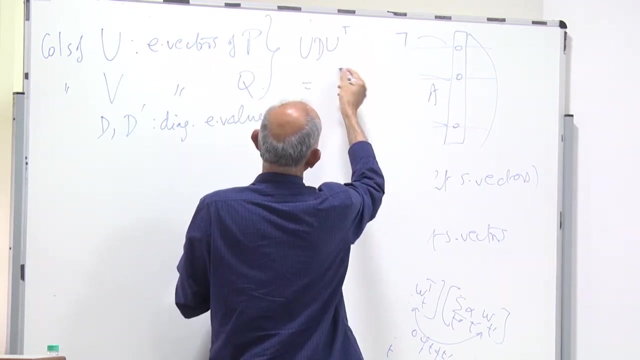 So we have been using a slightly different notation. But u d d is diagonal, d d prime are diagonal. They are the eigenvalues. So u du transpose, if you think about it, is the same as saying lambda i- this is for p, lambda i of p. 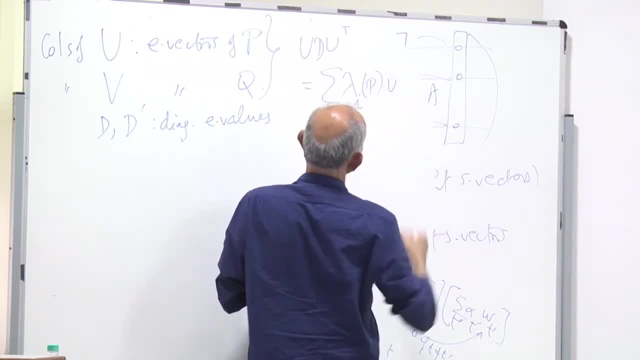 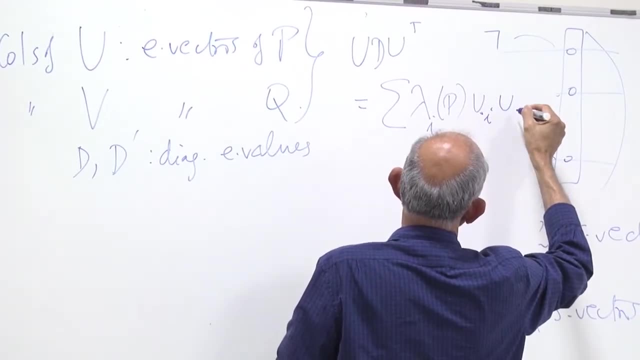 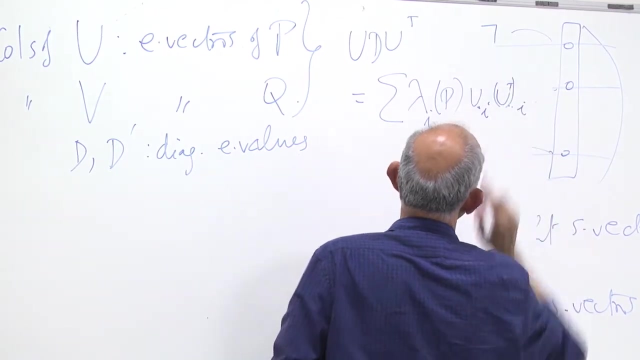 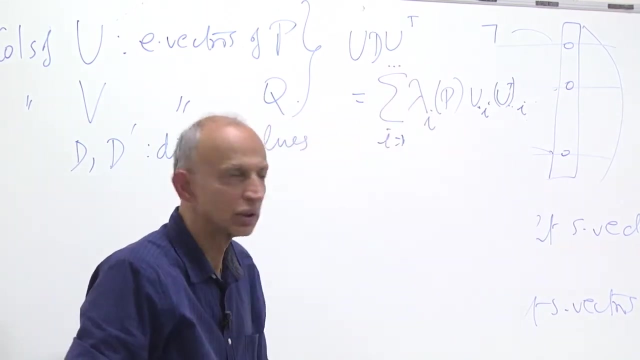 So that's u, column i of u. So column i of u. I wrote it this way before, so that's right there. And that is ui transpose, u transpose. i row i of u transpose. I'm just expanding the matrix. this is just the matrix notation, if you haven't used before. 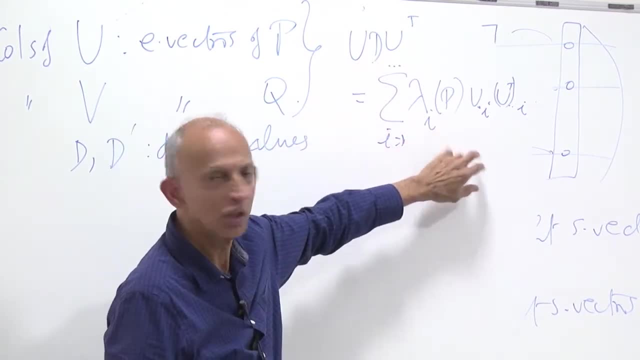 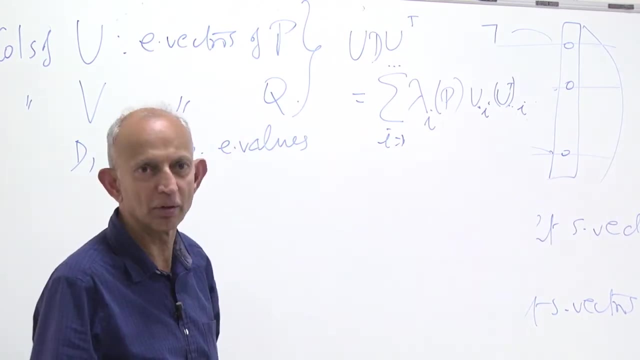 but more standard than the one notation we've been using, right, So this is just the outer product of columns and rows. They sum up. It's worth checking that these two are the same and these diagonal searches comes like that, okay. 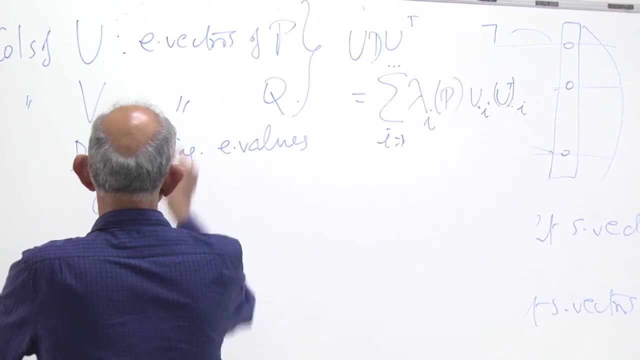 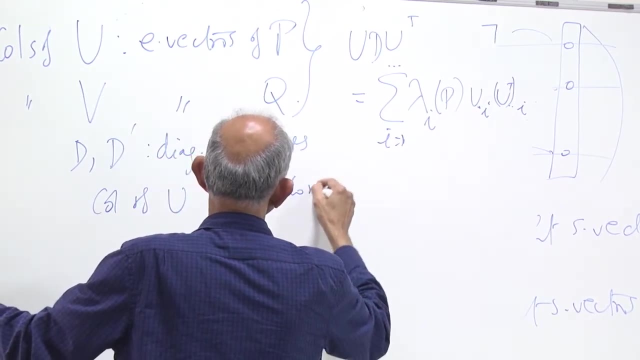 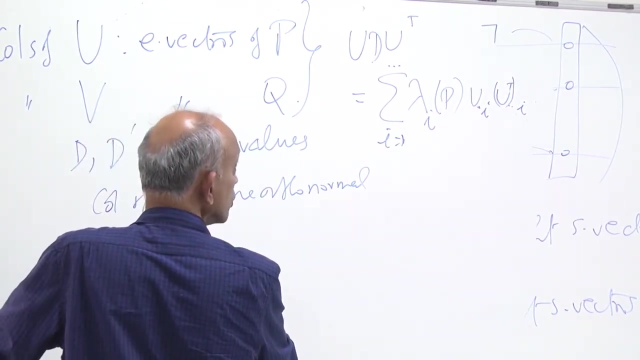 Now what we know is that the columns diagonal vectors are orthogonal, The columns of u and v, u are orthogonal or orthonormal, And in matrix notation that is just going to say that u, u transpose. no, sorry, I was going to say u transpose, u is the identity, and 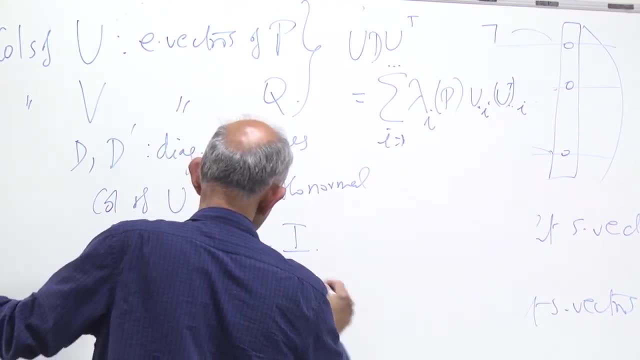 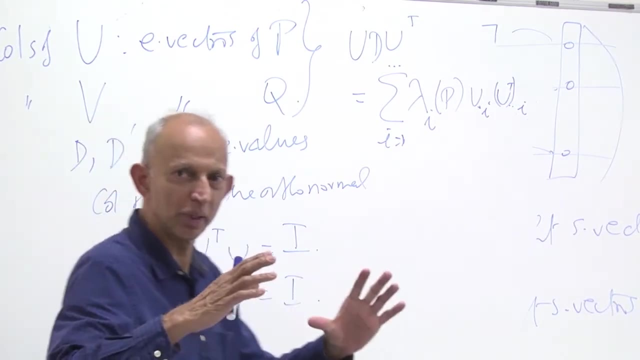 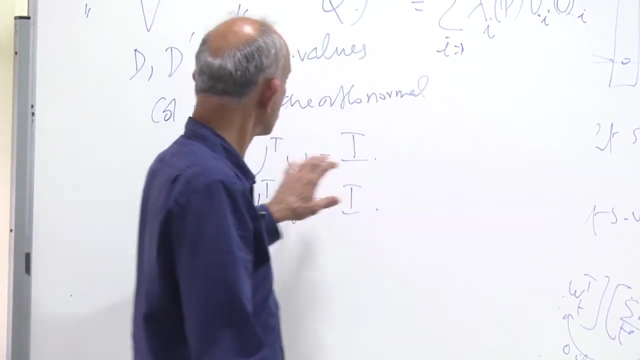 v transpose v is also the identity. Actually the other way as well, because if you have a full dimensional orthonormal matrix, then the rows are also orthogonal. So if you have in n space, you have n columns which are orthonormal. 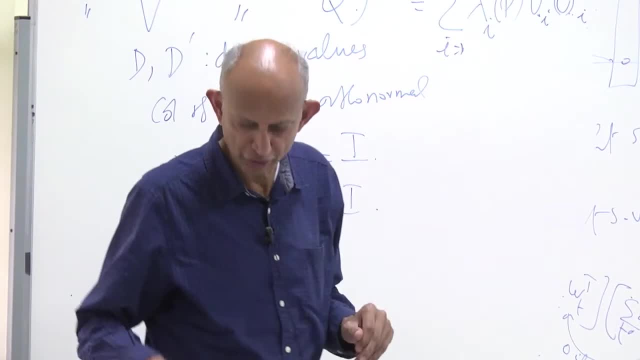 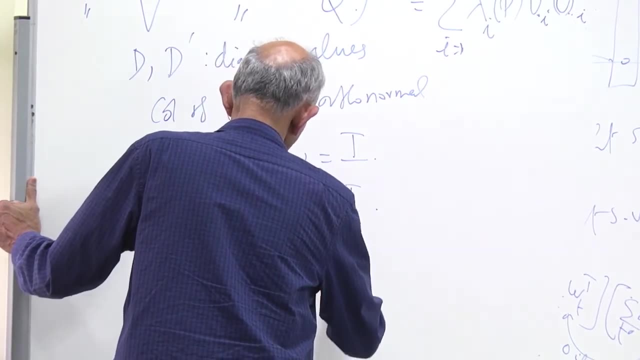 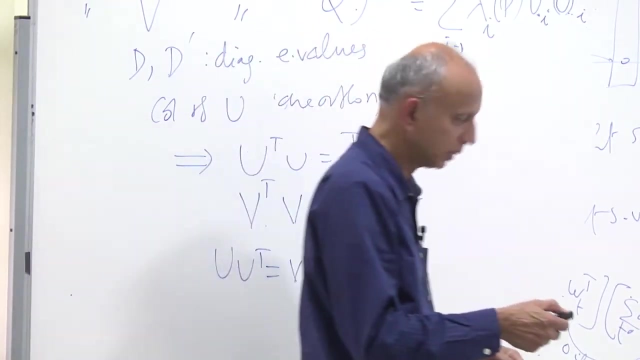 the matrix also have orthonormal rows. Not true if it's less than n, but if it's n, that's true. So in fact, u- u transpose is also equal to v, v transpose equal to i. okay, Bunch of linear algebra. we'll recap and we'll use that, okay. 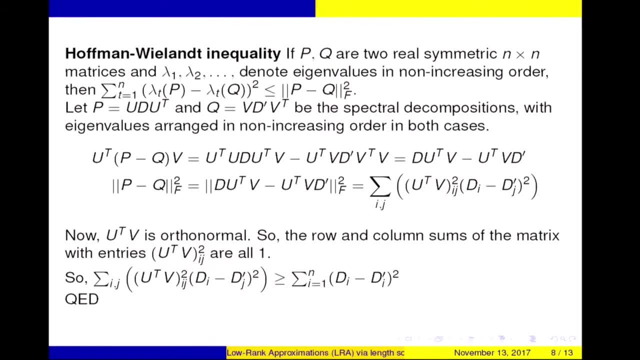 So these are spectral decompositions with eigenvalues arranged in non-decreasing order in both cases, And I'm going to do something, Something that it looks it's pulled out of the hat. So I'm going to take p minus q, multiply by u, transpose and v. 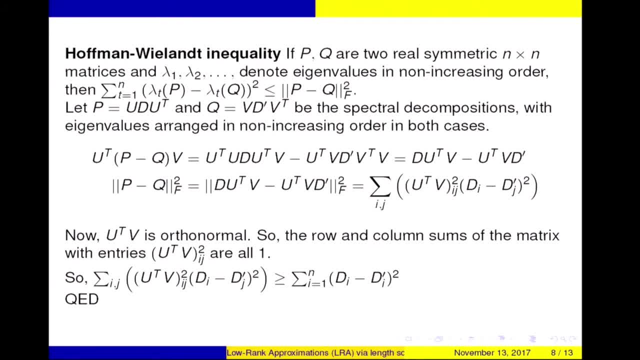 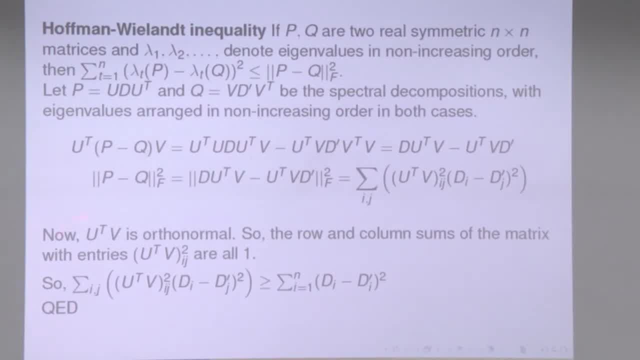 On the two sides. I'm just expanding this out. U transpose u d and so on and so forth, and I get that. Now, u transpose u is the identity, right? It's one of these things, So that goes away. I get d times u transpose v. 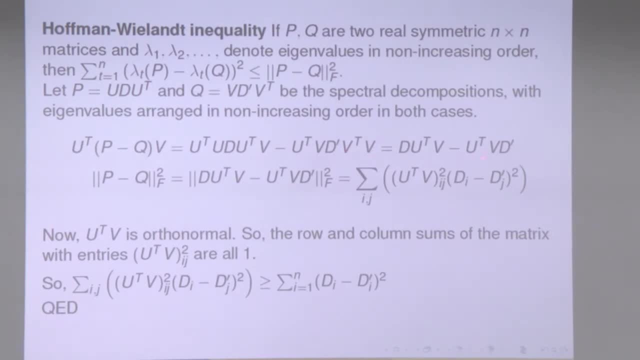 And again, v transpose. v is the identity. That goes away. you get that Now. these are all the normal things, so they are all length preserving. They don't change the Frobenius norm. okay, It's invariant Frobenius norm under these transformations. 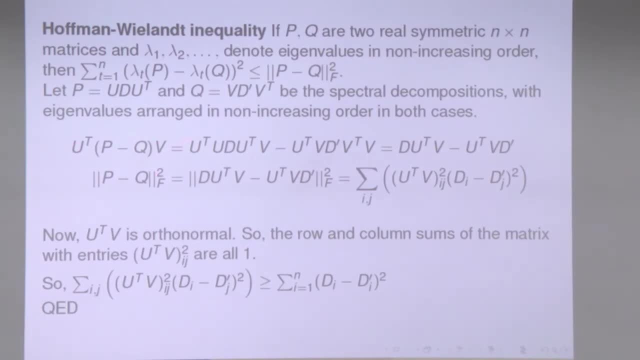 So I get. this is just: I'm taking the Frobenius norm of the whole thing here squared, that's the same as p minus q squared And that's the same as that Frobenius norm squared. And that's the expanded version of this. 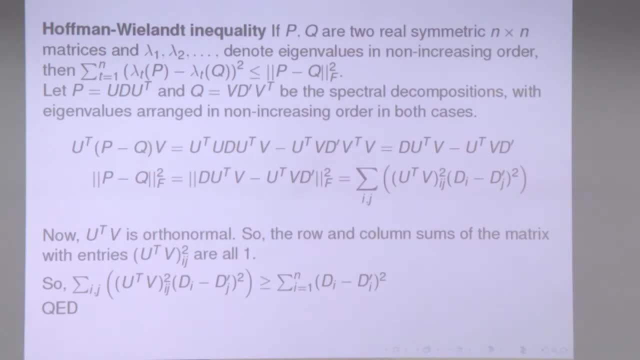 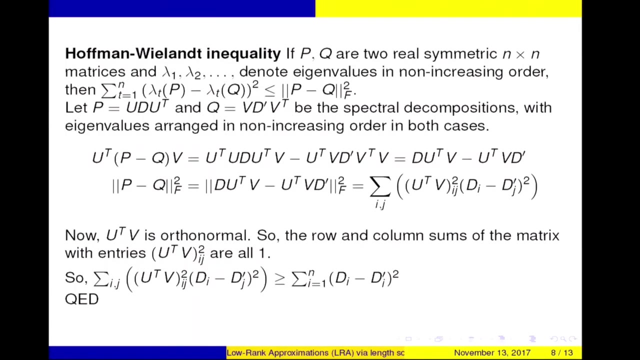 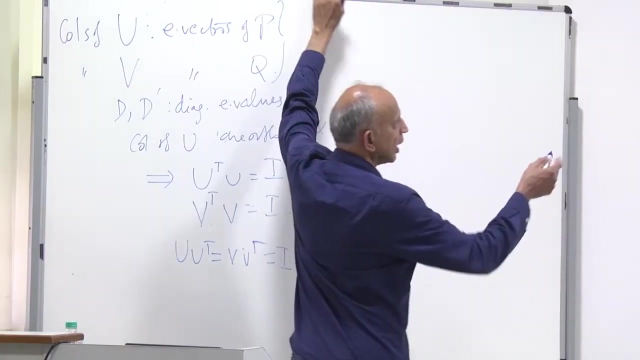 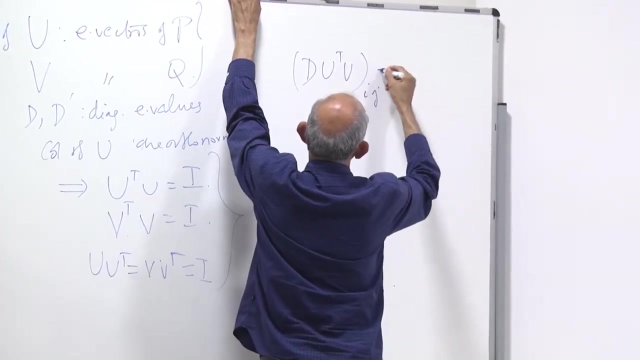 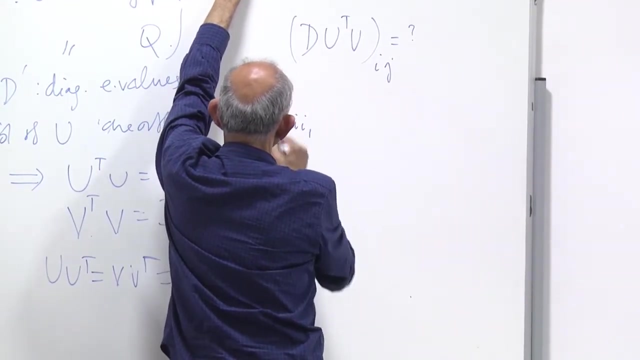 Now why is just quick check that that is correct. That's just algebra, but let's check. So I want to know what the ijth entry of this is right. Well, ijth entry of this is: di i1, sum over i1, u transpose i1, i2.. 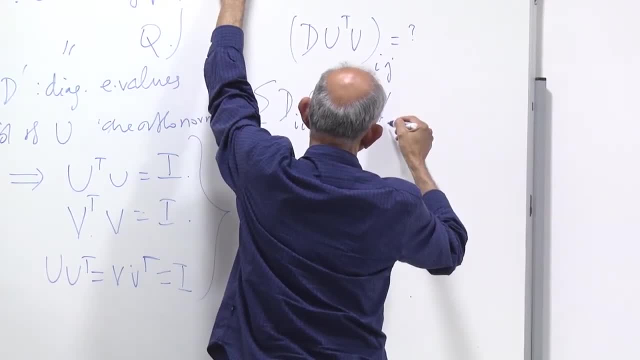 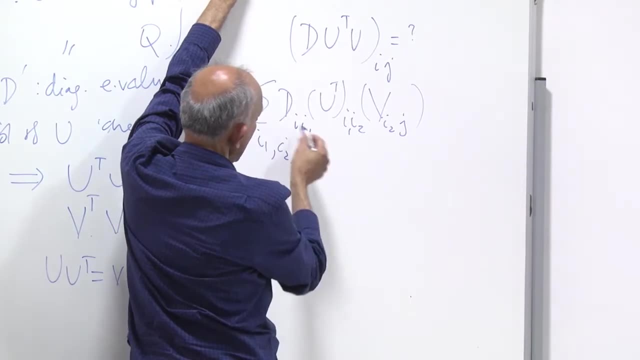 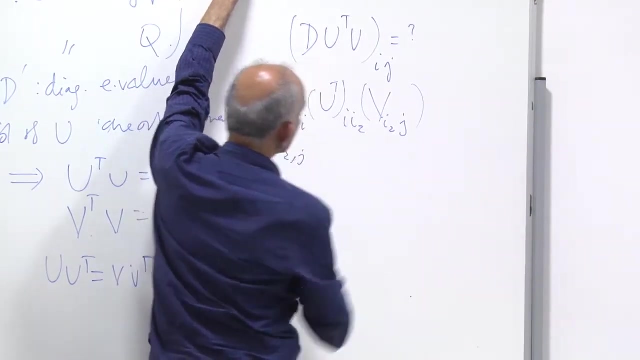 I'm just writing them down: And v- i2, j right Sum over i1, i2, and j- i1 better be equal to i, otherwise it's 0, so this goes away. This is i, okay. 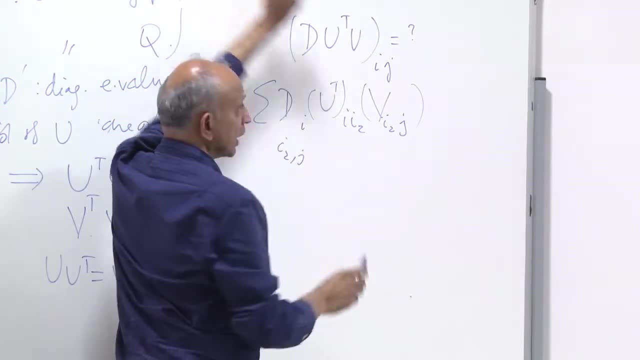 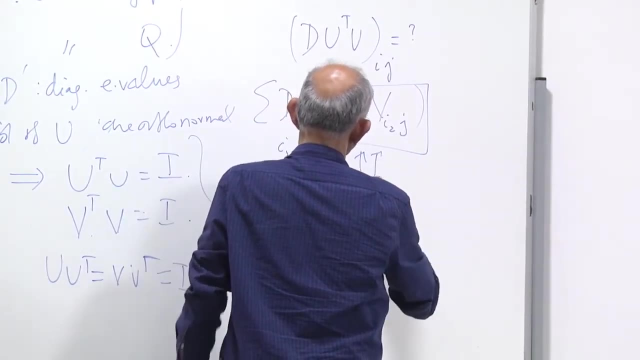 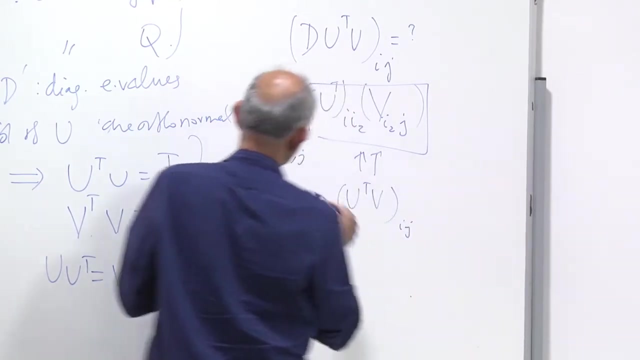 And so you get dii is just I call it di. okay, And this is just U transpose v's ijth entry because I sum over i2.. This sum over i2 goes in there and I get that. 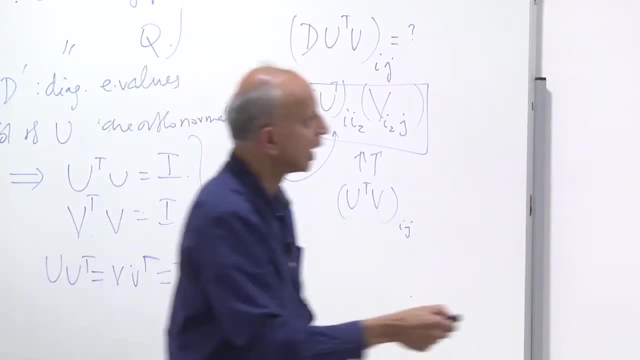 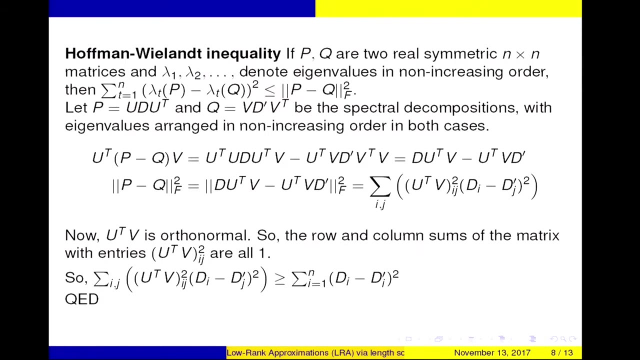 So then I've just done the algebra for the first one, right, And this is similar, just u transpose same, u transpose v, So anyway, so you get that Now. u transpose v is also orthonormal, because u and v are. 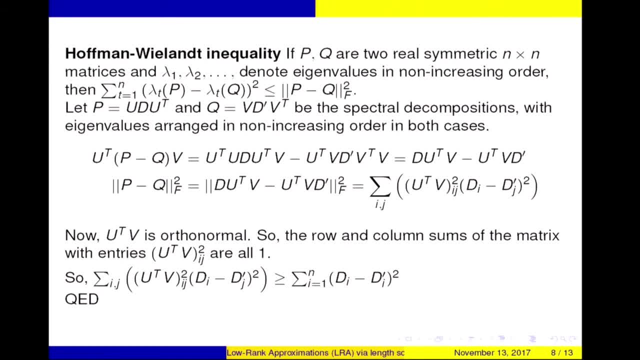 You have to check that Another linear algebra, in fact maybe I won't check that. They are orthonormal. and so the rows and columns, column sums of the matrix, rows and column sums, column lengths, are one. That means the sum of squares is one. 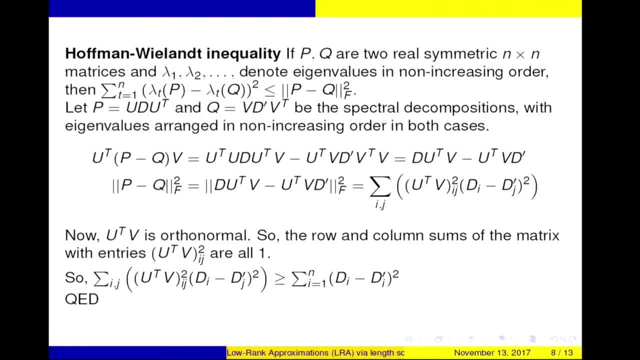 So if I take this matrix, that is doubly stochastic, right? So I put this. Then I use the theorem from the last slide, right? So this: so di minus di prime squared, these eigenvalue differences squared. it's something that I want. 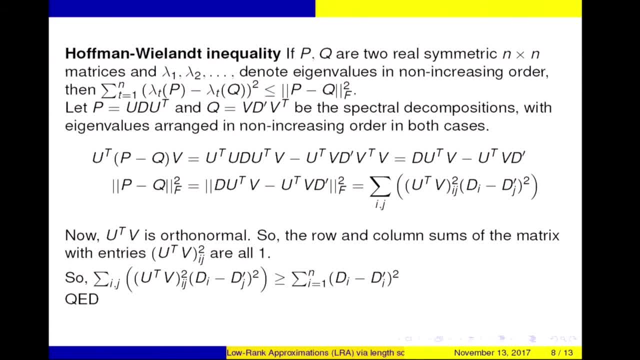 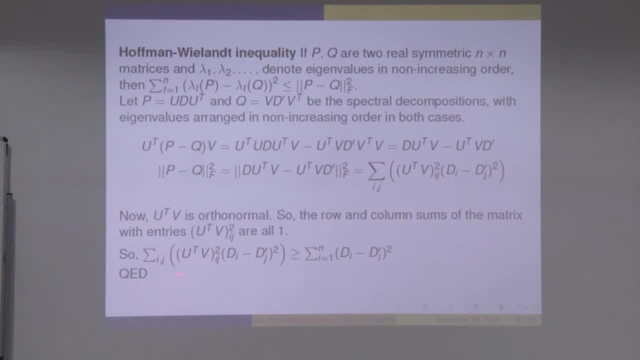 Okay, That's what I want, right? Those are weighted by a doubly stochastic matrix and the minimum is attained when I put the identity there. That's what I showed in the last slide, right? So I put the identity, so the cross terms go away. 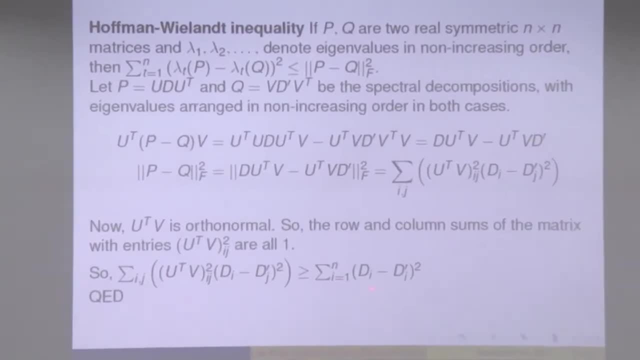 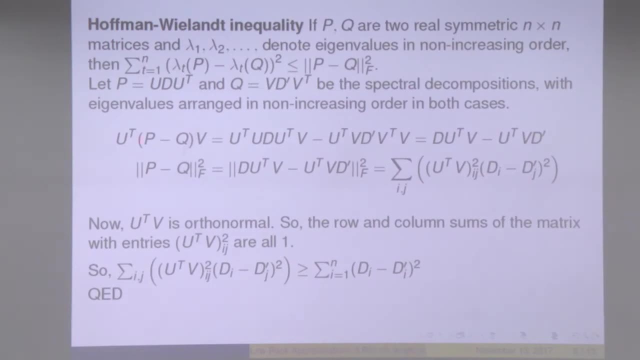 i and j not equal, go away. so you just said i and i for both d and d prime and you get that. okay, You do have to check all the intermediate steps. So this is that quantity Right And I started from that. I started from that sign. 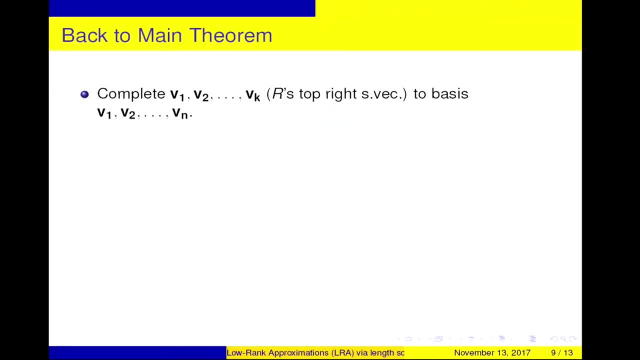 Okay, so that's Hoffman-Wiener and let's go on to our theorem. Okay, so V1 to Vk. so now we have to do a little bit of algebraic manipulation, unfortunately, to get to the theorem, But it's not too bad, I hope. 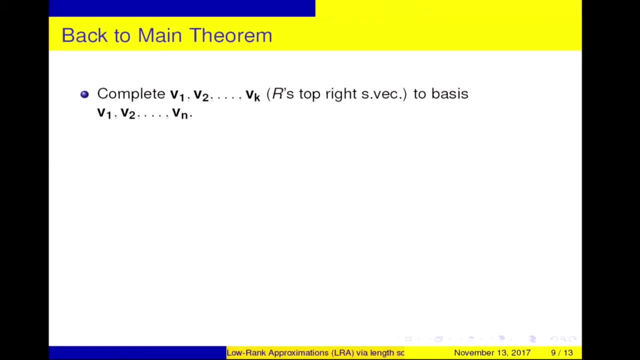 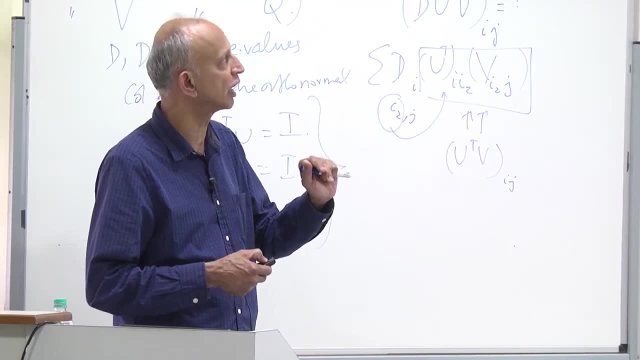 So we compute, we take V1 to Vk. So the theorem said: I'm going to restrict A to the space spanned by a and by the top k singular vectors of r. So these are the top k singular vectors. I'm gonna make a full basis out of it, right? 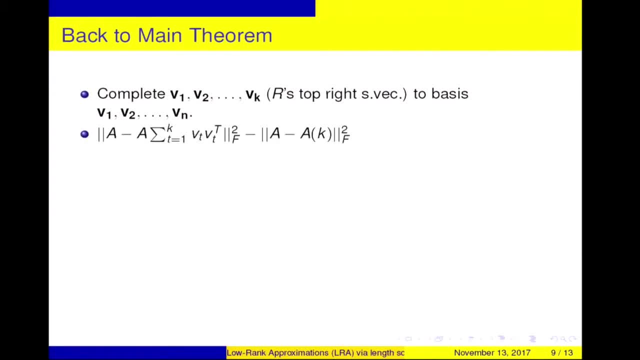 You can always complete a basis normal set. So I would like to prove this is small. So this is A's restriction to this. I like to prove this is small And I'm gonna pull something out of the hat. I'm gonna pull this out of the hat and subtract. 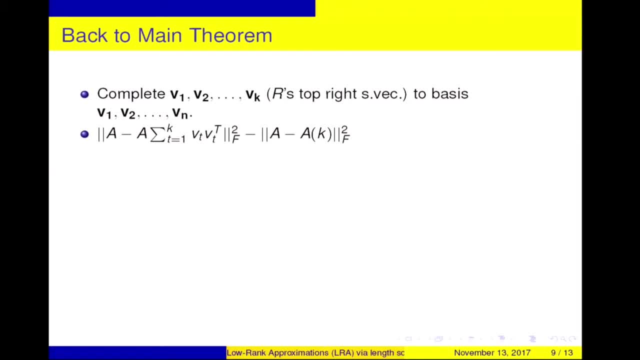 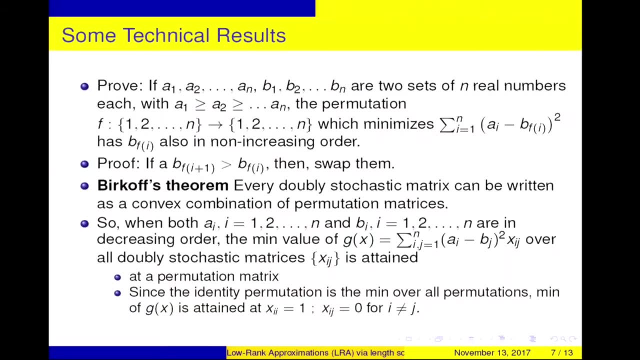 So again, unfortunately this, you'll have to go through some manipulation here. In fact, I wanted to prove this expression to you. I wanted to prove this is small with respect to this right, So maybe I should go back to the theorem for a minute. 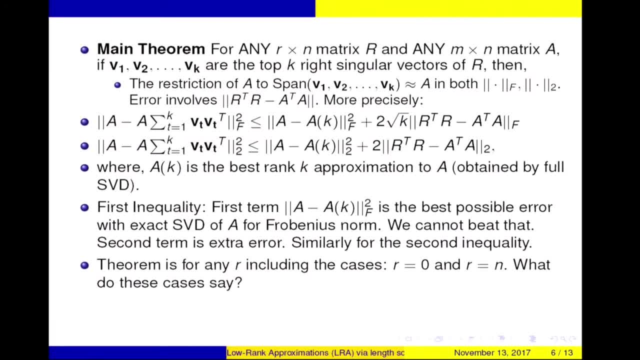 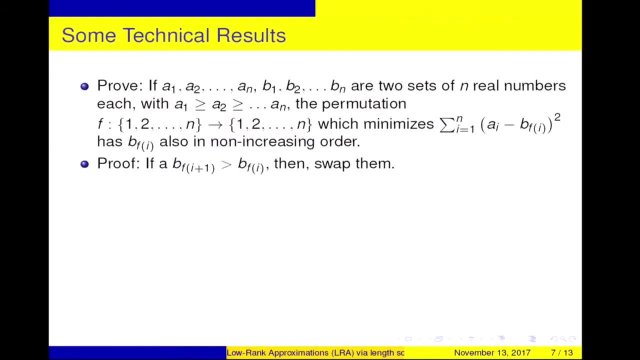 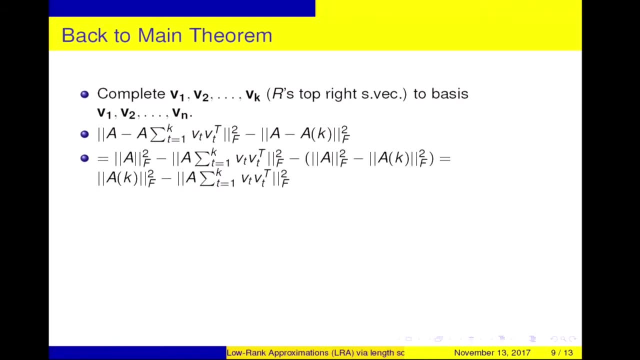 Yeah, so I want to prove this is small comparison to that. I just brought this over to this side, So I've taken this minus that I want to show that's small. So I have that and I'm gonna expand that. Okay, so this a few more lines of proof. so this is A. 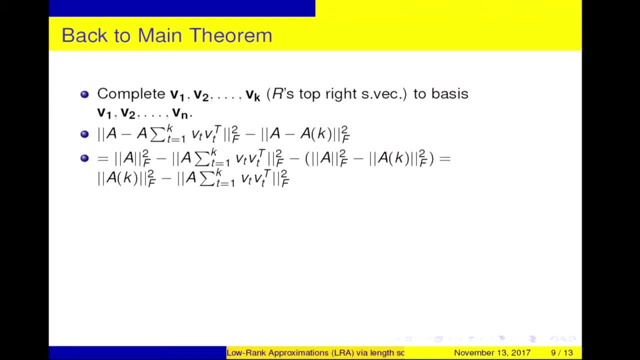 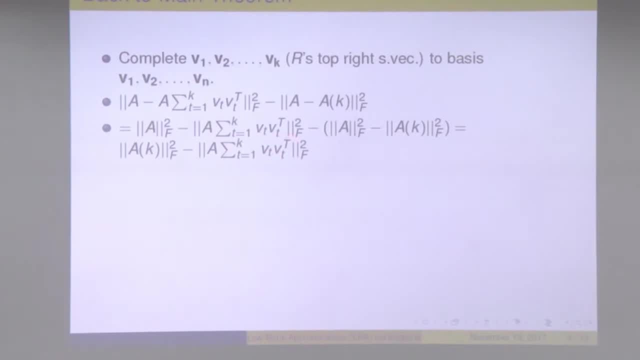 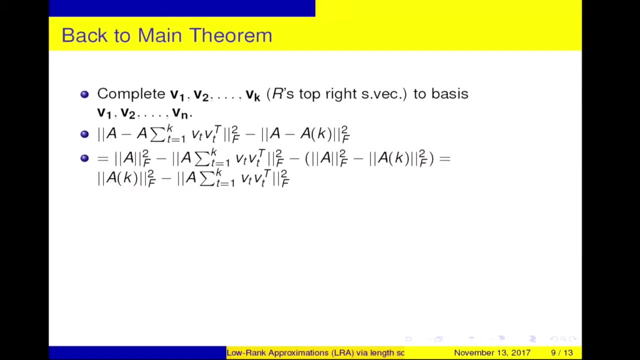 This is A restricted to a particular subspace. okay, And that's always. the provenance of that Difference is A minus that You have to prove that right, But I mean a simple proof of that Is just by the completion. 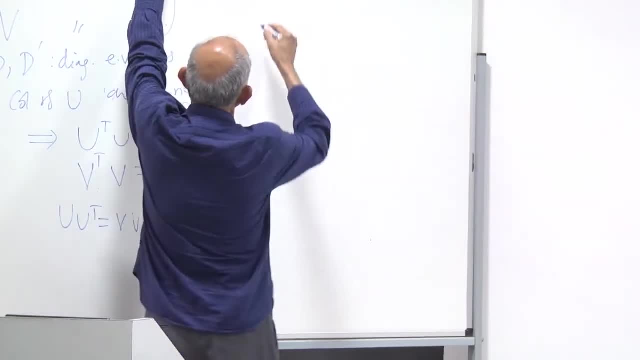 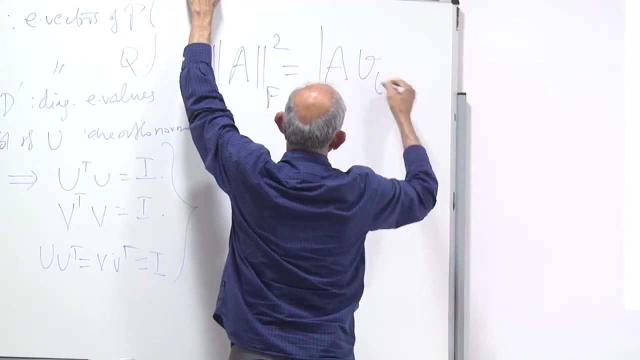 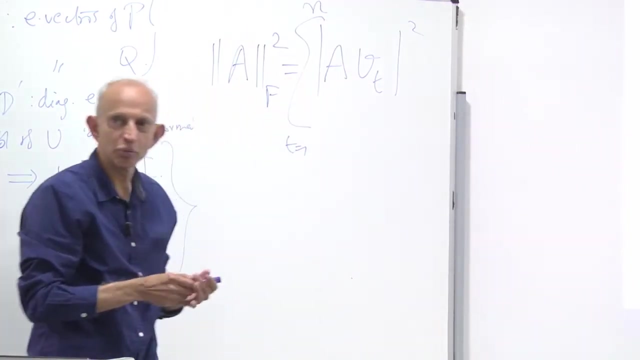 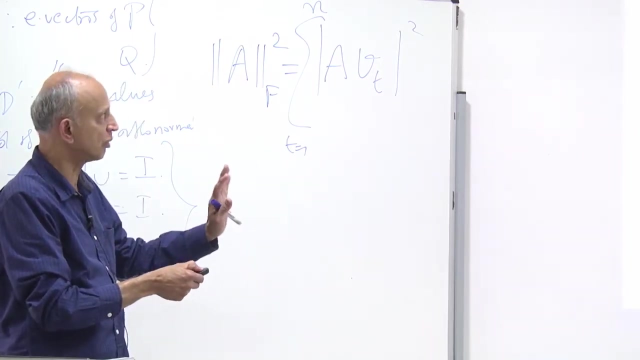 Of the basis. so Okay, maybe I should write that. So AF squared is just equal to A times VT squared right. So the provenance from squared is the sum of the rows squared length, and you can write the matrix Norms. nice norms are always invariant, whatever the basis. 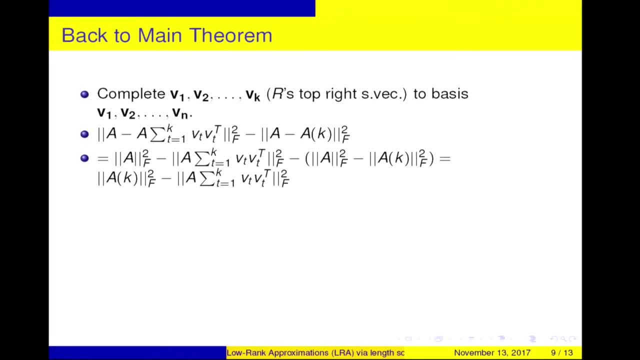 So I choose VT as the basis, then you'll get this, And I subtracted out the first case so you get only k plus 1 to what's left right, So that minus that, You also have to prove that that is equal to that. 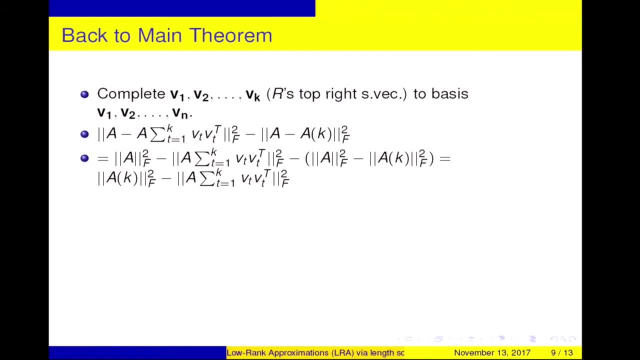 Again, similar proof. I won't do that. These two cancel out And you get that minus. that okay, So that I have to prove is small. A few more tricks. So a k is the best rank k approximation. so that came from SVD. 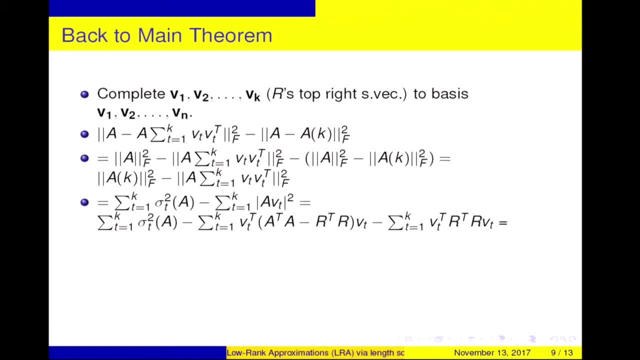 So that's, that's okay. That's just the SVD theorem, we proved. We proved that SVD is the best approximation, so you get that. What about this? You can see that that's just equal to A VT squared right. 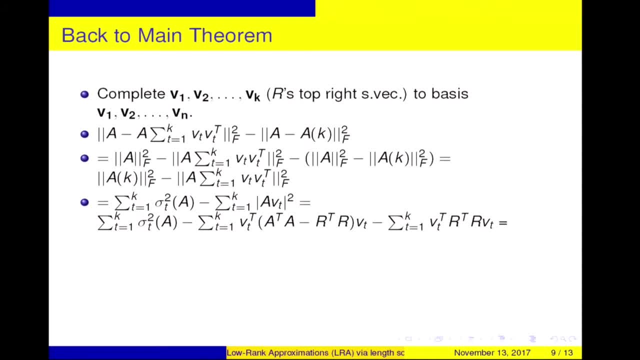 See, all of this is not true if it's not autonormal. Everything uses all these facts, so that's true. So now I want to write that as equal to. this is the same as what I had before. Here's another trick. 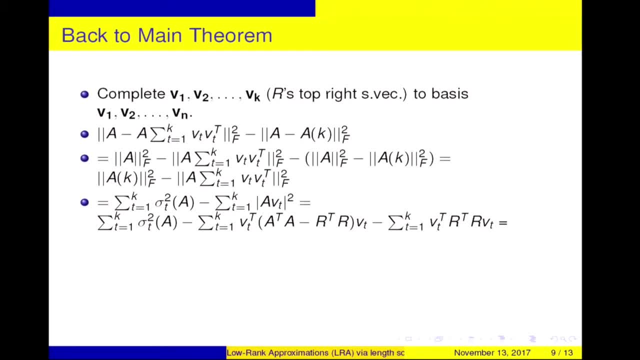 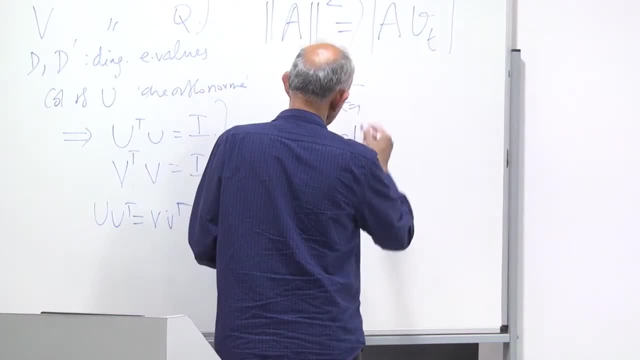 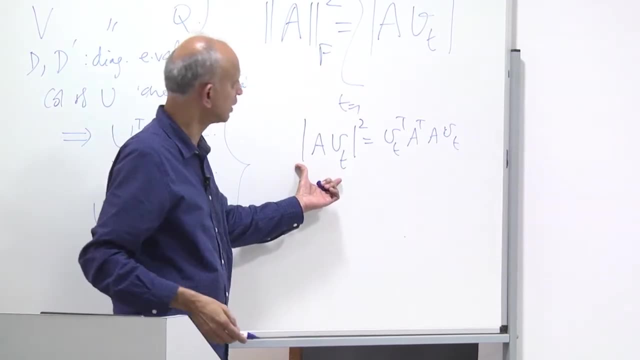 I'm going to take A VT squared, That is, I mean, the first. here's not a trick, it's just simple. That's just equal to VT. transpose A, transpose A VT. right, There's a length squared of a vector that's equal to its dot. 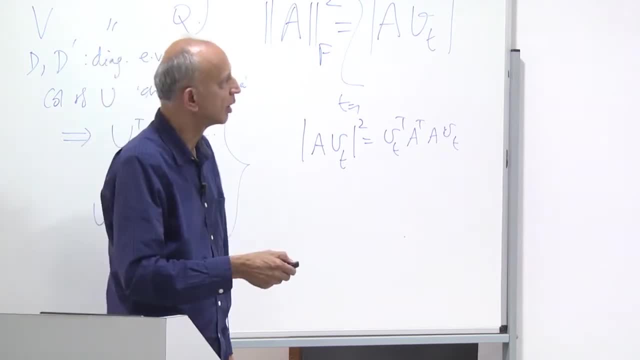 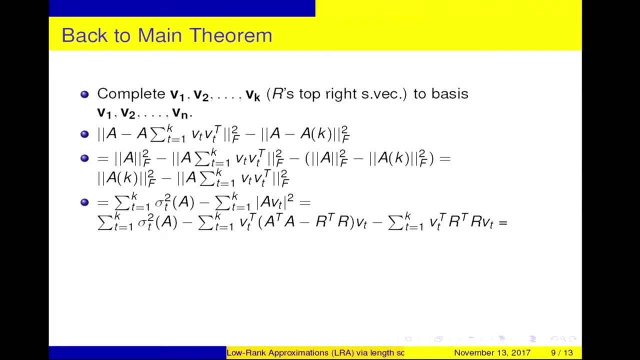 product with itself. Again, that's not a trick, But I'm going to add R, transpose R and subtract it. okay, That's okay, I'm adding and subtracting. I've done this several times. I did it last time too. 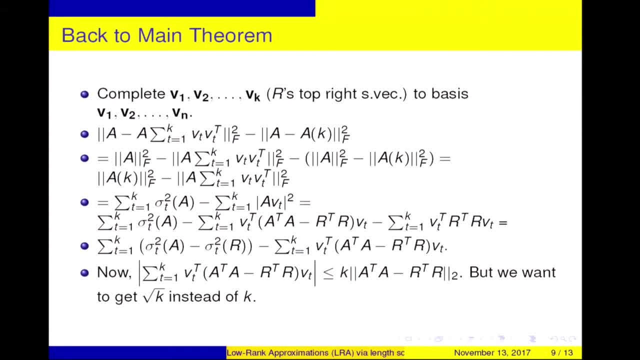 And now what do we get? Now we get this, is this squared Here: VT are the singular vectors of R, so those are just the singular values of R, So that's a difference. Okay, so I'm going to use this difference and 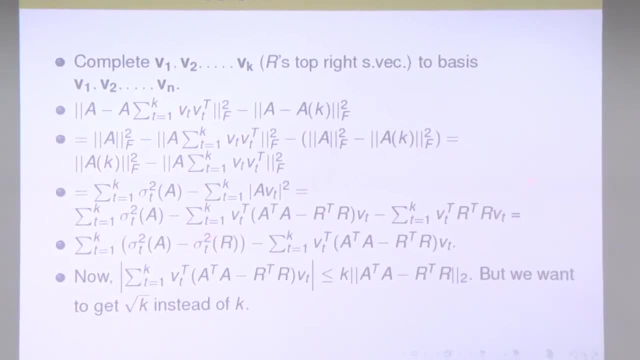 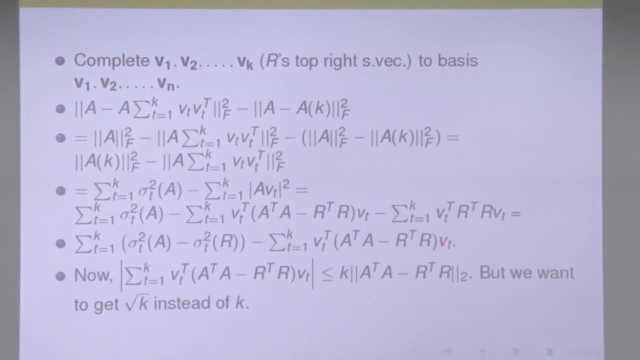 bound it using Hoffman-Wieland. I'm coming to that, But that's this term and this term. I still have to deal with this term. I've rewritten that I've not dealt with it yet. So now this is less than or. 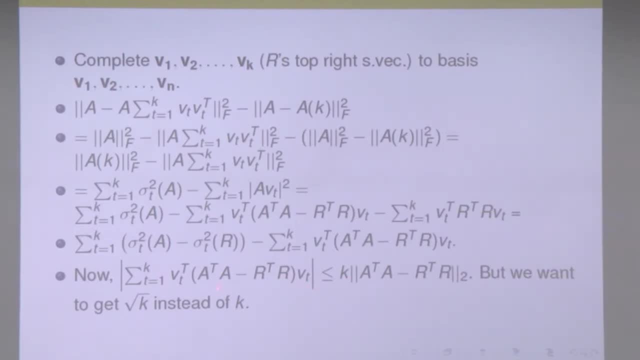 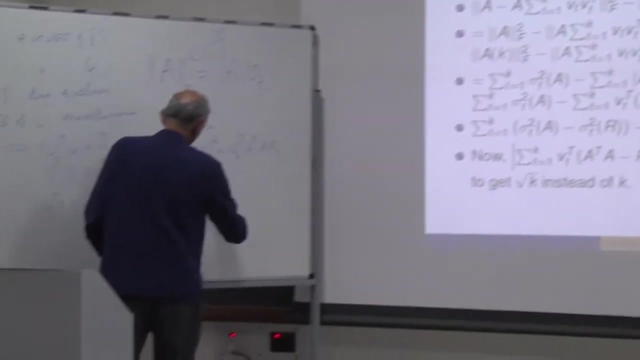 equal to k times That, because for each vector V, this quantity is at most the spectral norm of that. okay, Now we define spectral norm slightly differently, but yet we define spectral norm of A as the max over all V of A V. 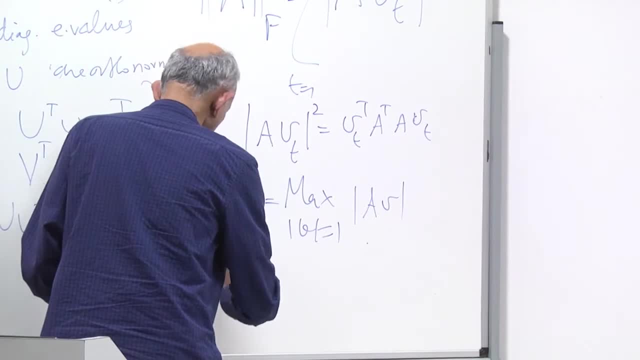 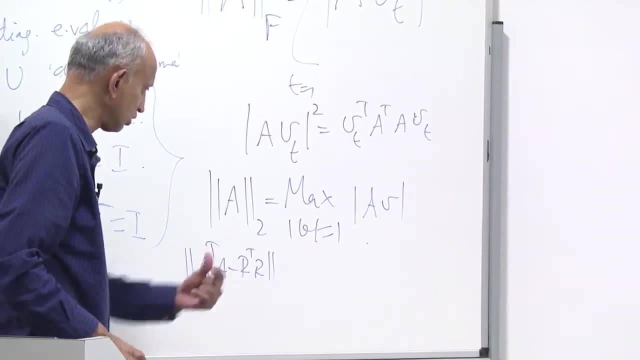 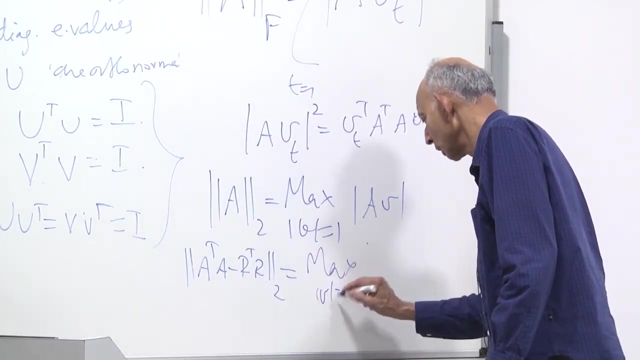 But it's also true that the spectral norm of A of a symmetric matrix- A transpose A, minus R transpose R. this is symmetric, they're both, so the difference is symmetric. For a symmetric matrix, a spectral norm is the max over all V of V transpose times. 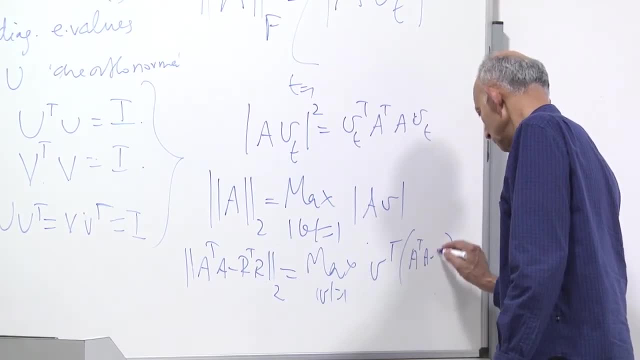 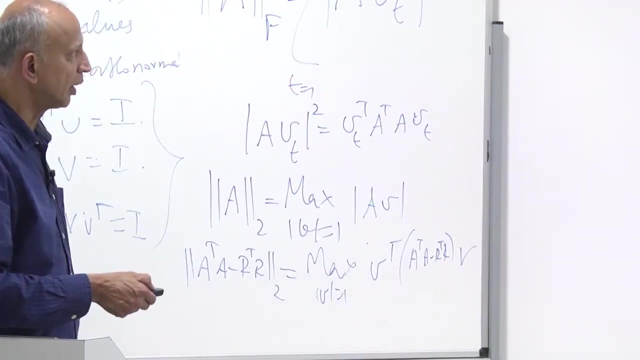 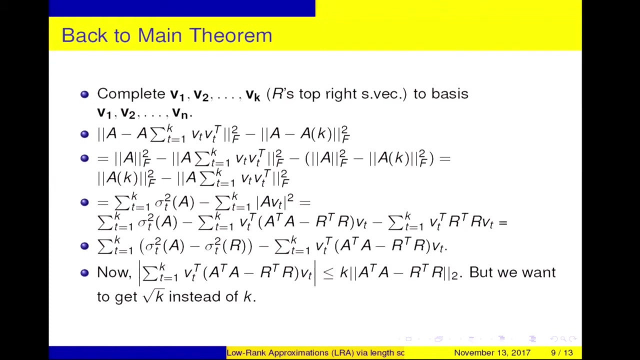 the matrix times V. Okay, this all at the end of this day. this gave me a k, but I want to get a root k. If you're happy with k, you're done. So I'm going to work a little little, little, little little. 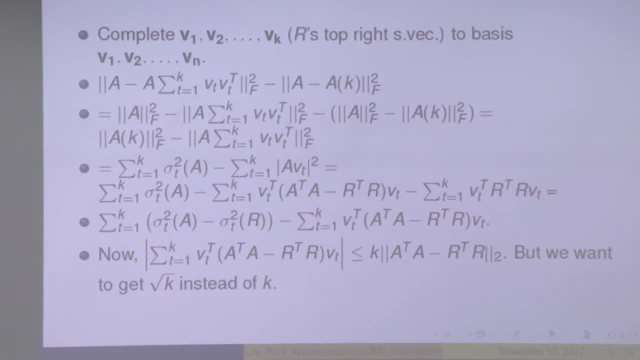 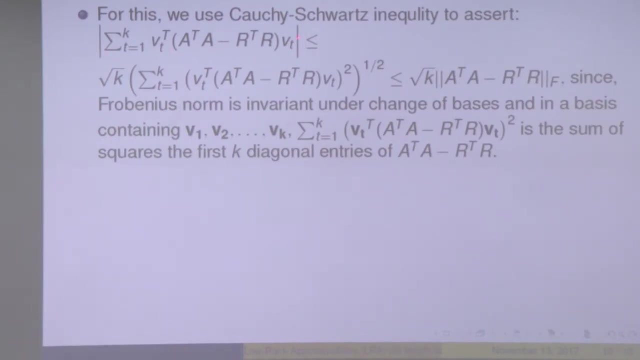 little bit. one more slide of work to get a root k. So for this we have to use Cauchy-Schwarz. so we take that The reason I'm doing this proof is partly it's. algebra is uninteresting, but hopefully it'll jog your. 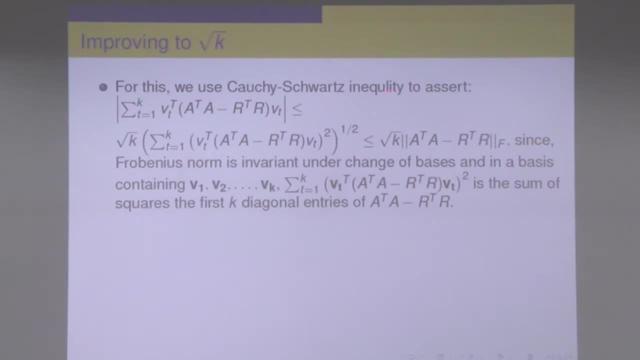 memory on the linear algebra that you might have forgotten. So for this we use Cauchy-Schwarz to assert that that is less than or equal to that. That's just the sum of k real numbers. these are real numbers, So that's less than or equal to that. 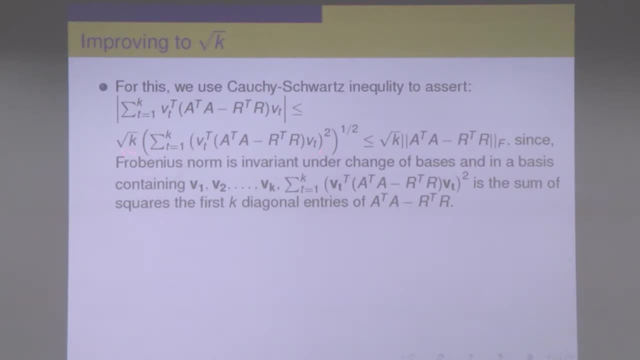 Okay, Okay, So that's the sum of square, then square root and then a root k at the top. Now, what is this? so this is it's all. I claim that that's, at most, a Frobenius norm. why is that? 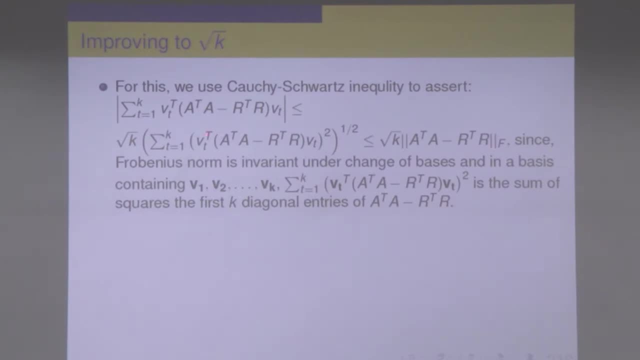 The Frobenius norm is invariant in the change of basis. So in the Vt basis right These entries are the diagonal entries of that matrix. So we have matrix A transpose A minus R transpose R. If diagonal entries in that basis are just this, then the 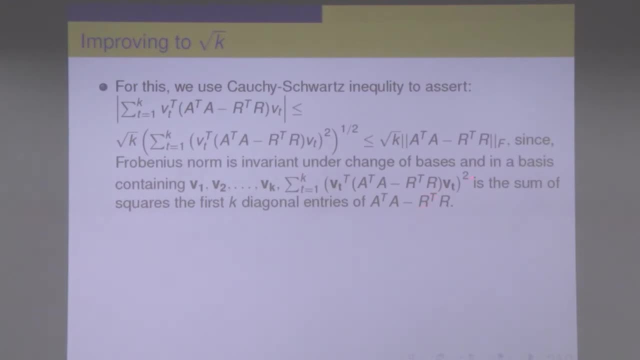 I'm taking the sum of squares of the diagonal entries, which is at most a Frobenius norm. I'm throwing away something cuz off. diagonal is not being counted, so that you get that okay. Okay, we are still to bound that. for that we use Hoffman-Wieland. 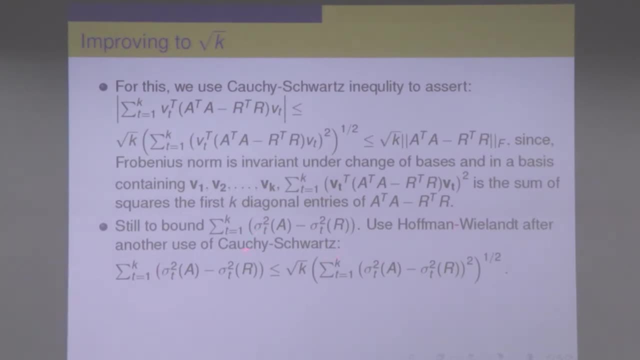 So, by the way, Hoffman-Wieland is only for symmetric matrices, as stated, So I had to do some of these machinations to get to the proper symmetric matrix. So we use another Cauchy-Schwarz, and then plugging all this in. 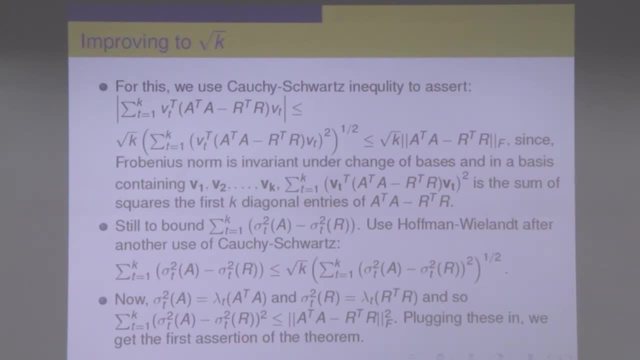 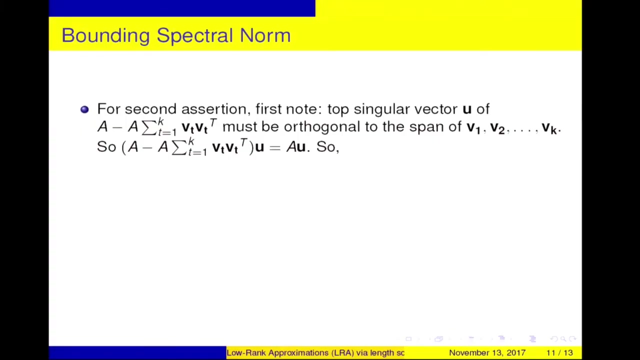 you get the first, you get the Frobenius norm. assertion Turns out, the spectral norm proof is not much harder in this case. Yesterday it was harder, but today it's not so bad Bounding the spectral norm. So we have only a couple more things. 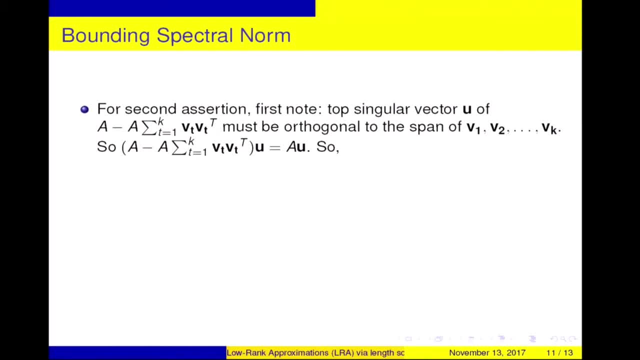 Bounding a spectral norm. For the second assertion, that's a spectral norm assertion. That's all. The top singular value u of this must be orthogonal to the span of this. So for this I have to write at the end. 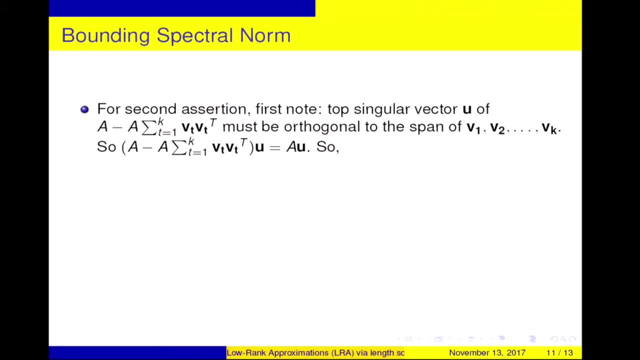 V1 through VK. so because I subtract out the action of V1 through VK, if you had a component along this it would make just 0, alright, So that's not interesting. So u might as well be assumed to be orthogonal to this. so 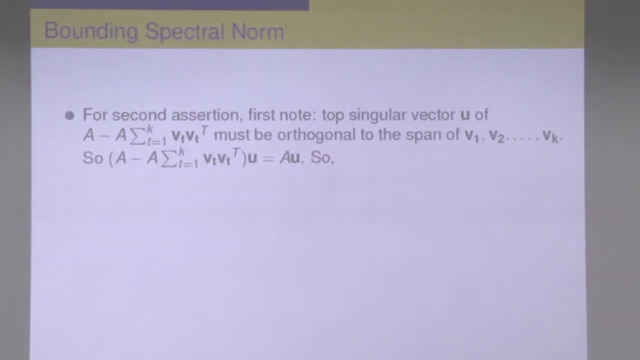 this product goes away and you're just left with au. So, again, we do have to do some work. So this is what I wanted to bound. so again, this is a. this is a restriction of a to that subspace. I want to say the difference is small. 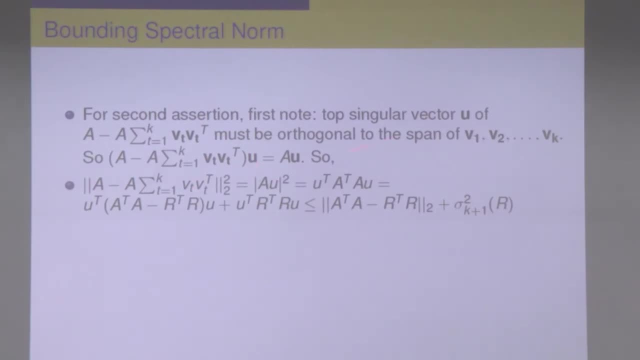 And since the top singular value is u, singular vector is u, so I get that. I get that. Now, this trick again. I have A, transpose A. I'm gonna add and subtract R, transpose R. It's same trick, And that's because I know how to bound this. that's this. 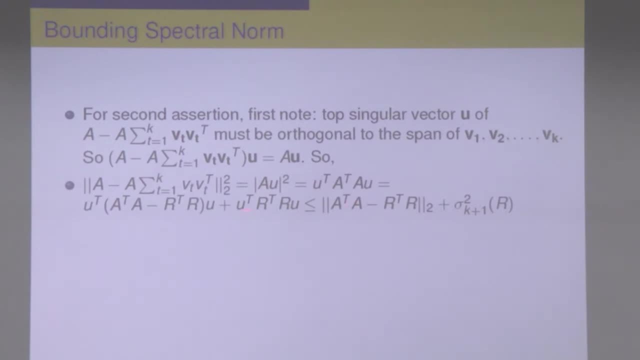 And this quantity, u, was orthogonal to the top k. singular vectors of R. These are the exact singular vectors of R. it's the top k, So this is at most k plus 1.. So we again saw that. So it lives in the space of the k plus 1, and 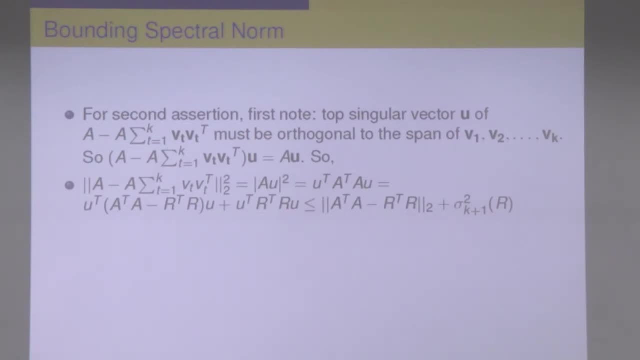 later singular vectors. therefore, you get the best of that. Okay, so we're not done yet. so that same written like that. Now I have that. I'm adding and subtracting Sigma k plus 1 squared A. this is, we know what this is. 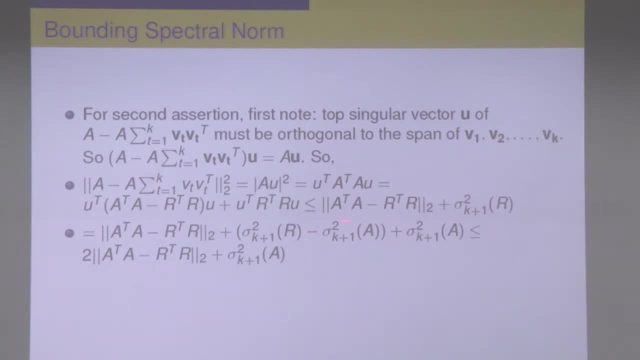 How about this? So I'm going to say that's also at most this Okay, and that is using Weyl's inequality. So let's remember that again. I'll write a short proof of this. This is one of the many inequalities in any algebra. 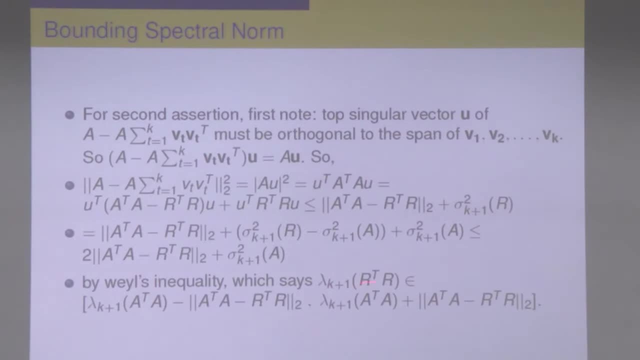 But so it says: for a symmetric matrix like R, transpose R. is I take the k plus first or any eigenvalue in decreasing order? Eigenvalues are in decreasing order. That is at most. I've written in a particular way. Let's write as inequality here. 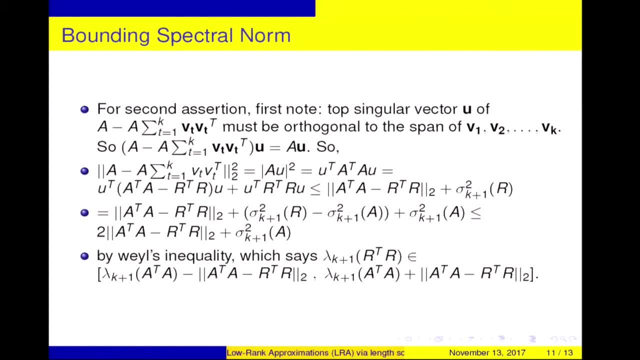 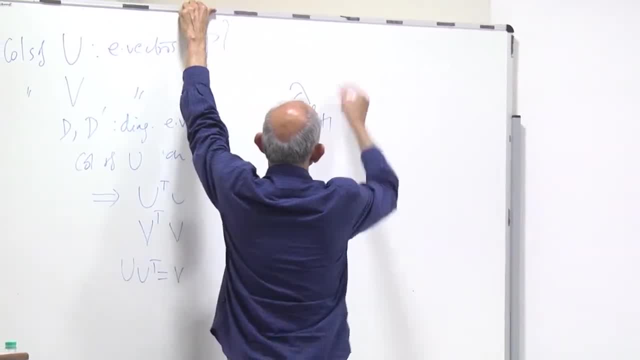 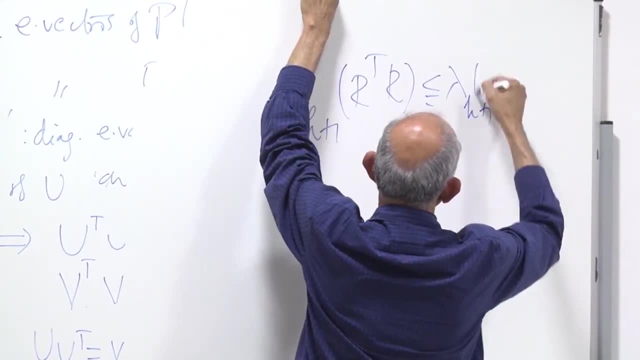 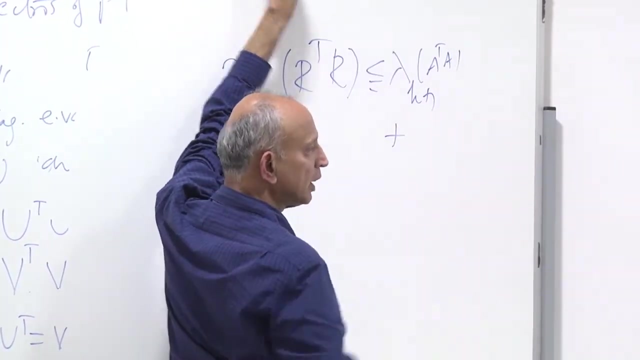 So it's saying: lambda k plus 1. R transpose R. For instance, less than or equal to lambda k plus 1 of a different matrix, A transpose A plus. I've written that, So that's I'd like to say. this is a term, but I'm not sure why. 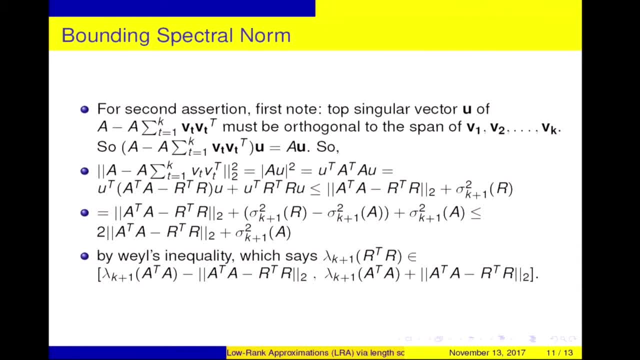 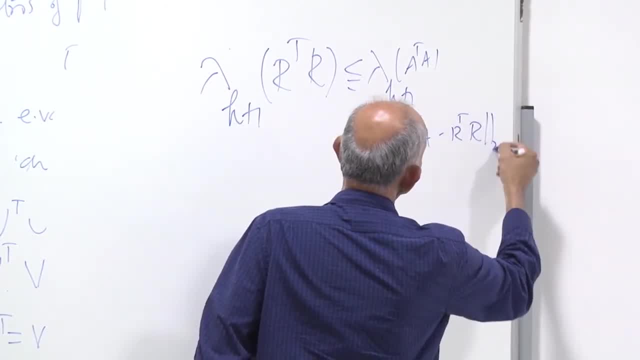 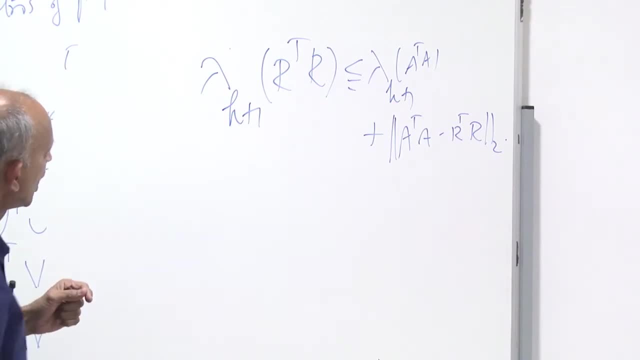 I'd like to say: this is a top eigenvalue of that, But it's a top eigenvalue and absolute value, right? So? So that is that side, and there's a symmetric inequality. How do you prove something like this? So we prove it by taking well. 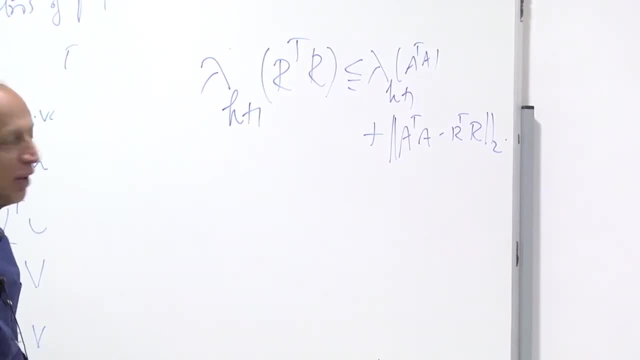 we have to use min-max theorems. I guess I didn't write Okay, so we don't prove it. You can look up a proof To prove this. I have to use- Let's prove this- I have to use min-max theorems. 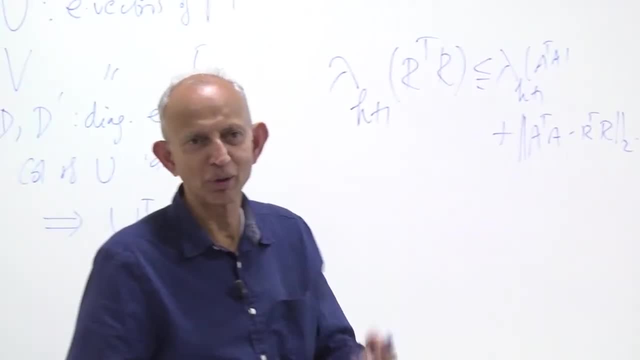 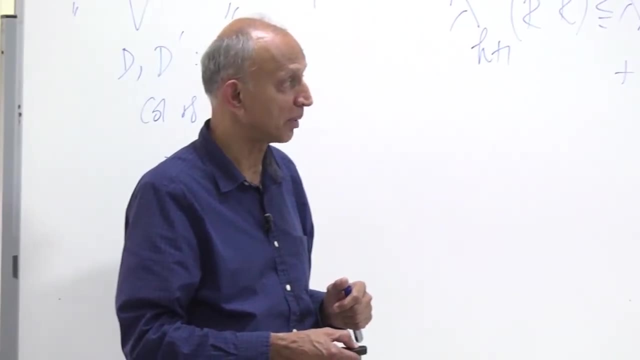 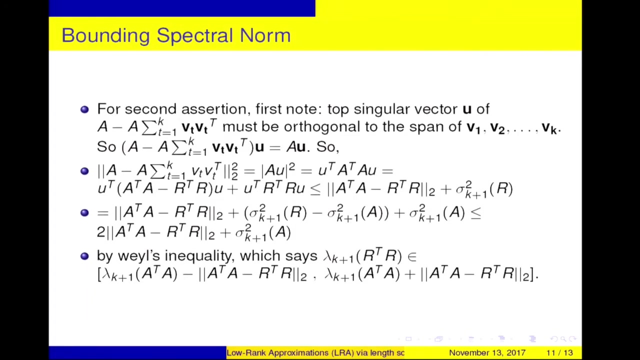 which I just realized. I didn't prove, But you can look up any standard book and you'll have this inequality. I do have to have symmetric matrices right, Otherwise I'd be a little more careful, But here we do, And that is telling us that this difference. 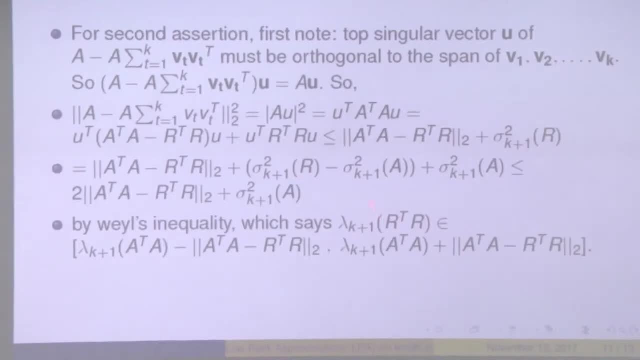 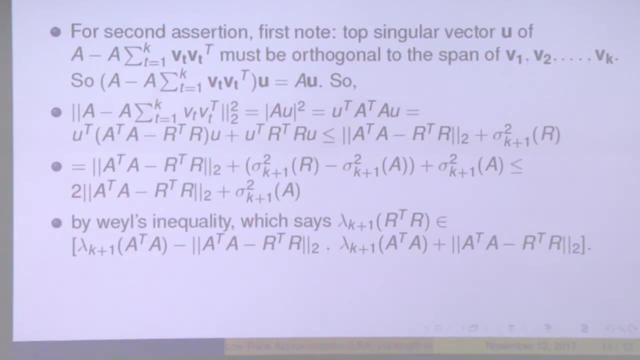 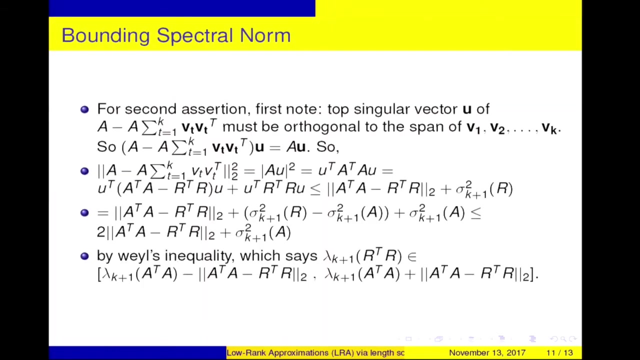 that's this minus that right, This minus that, This minus that Right. The difference between these two is bounded by this at most. So that's got the factor of two plus sigma k squared, The sigma k plus one squared. Okay, so that's the end of that story. for. 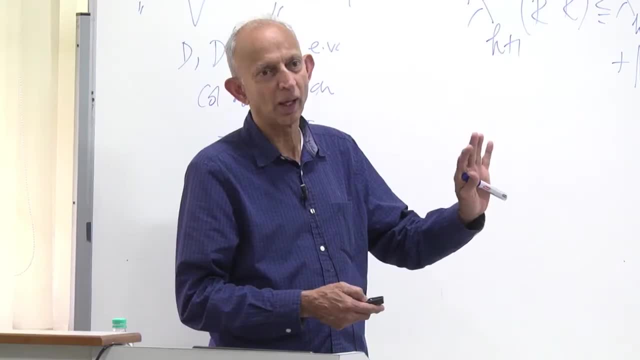 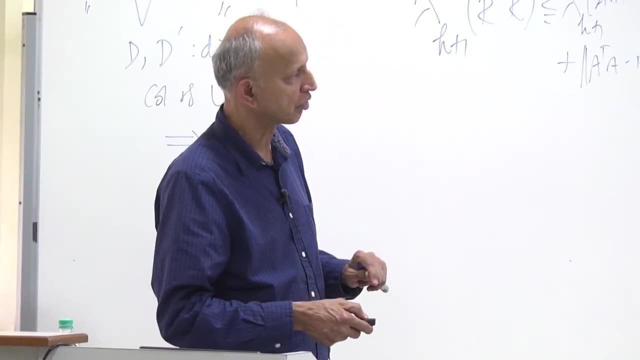 proving the main theorem. okay, And by length squared sampling, we can get an R. We can get it by any other means, right, As long as this is small, for which it's enough for us. Okay, Okay, It's enough to do SVD on that. R transpose R. 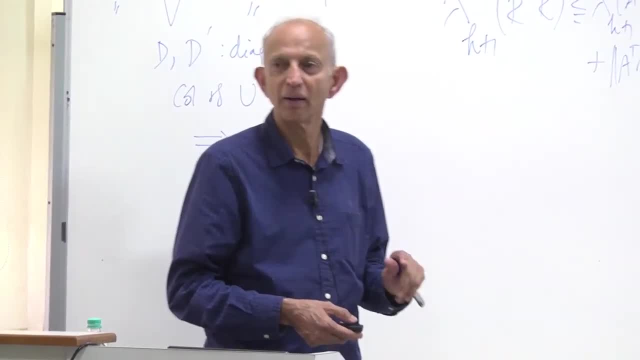 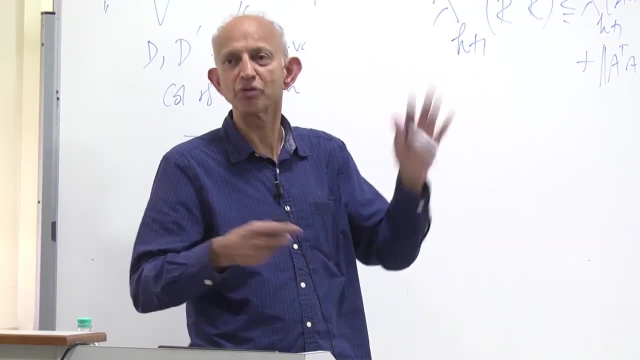 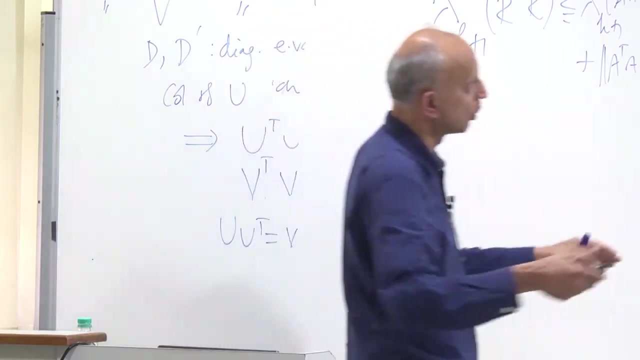 And now I want to take a step back and figure out what we have done in terms of time, How much we have saved, right? Okay, so this will also recap the overall proof and sort of the algorithm behind it. So what we needed was the right singular vectors of a smaller 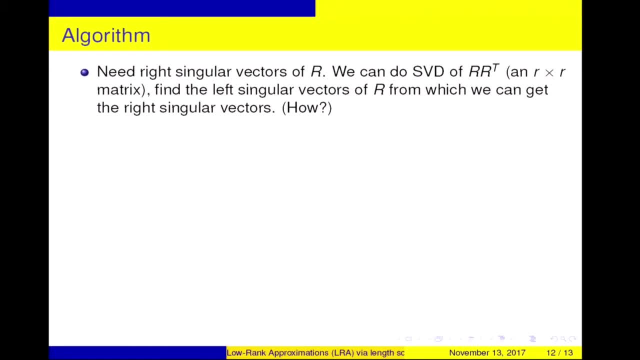 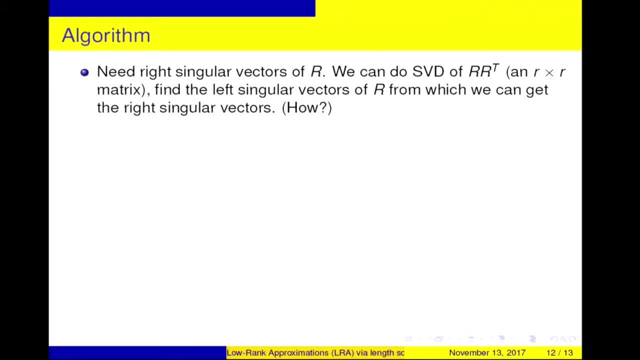 we'll analyze the running time. We can do SVD of R, R transpose, which is a small matrix, R over R matrix and that gives us the left singular vectors of R. So the eigenvalues of this are the left singular vectors of R. 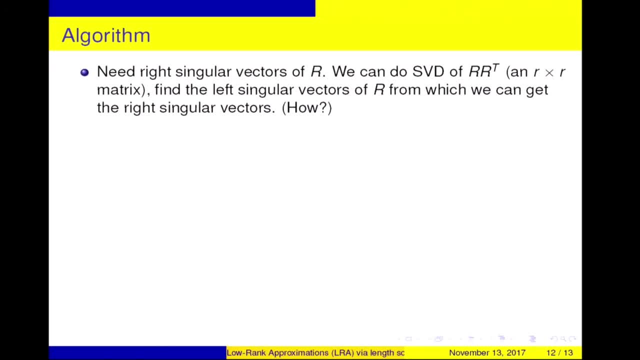 Because it goes on the left of R or the right of R, transpose, which is same as left of R, R, from which we get the right singular vectors. by just multiplying once by R, I'm going to figure out how much time all this is going to take. 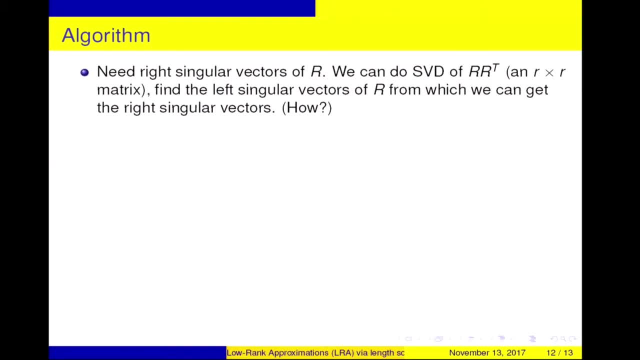 right, that's the story. So this how just meant multiplying left singular vectors by R to get the right singular vectors algorithm. So we pick R rows. Now I'm going to give you a length squared sampling version. You could do it by other means again. 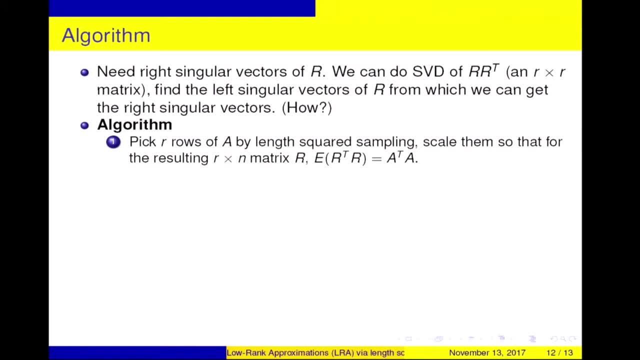 Pick R rows of A by length squared sampling. Scale them so that for the resulting matrix expected value of R, transpose R is A, transpose A. Remember this is going back to the beginning. When we did length squared sampling we said to make it unbiased you have to scale it. 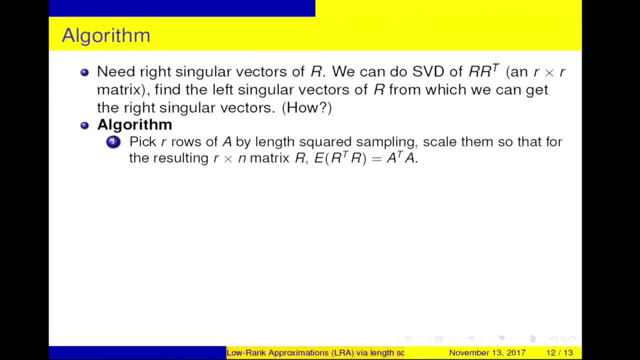 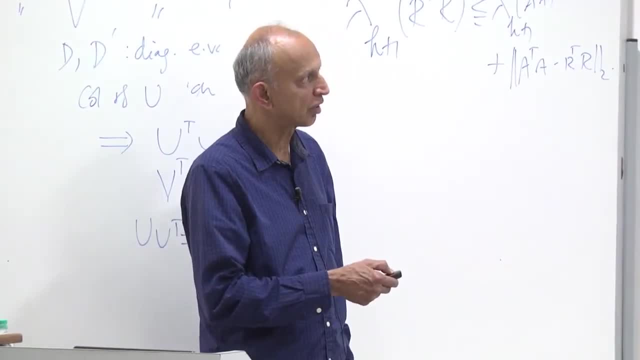 So you pick these rows right And to make the estimator unbiased you have to scale it. You have to scale down by the probability you picked. okay, So unbiased just means the expected value is right. okay, We already did this in the beginning. 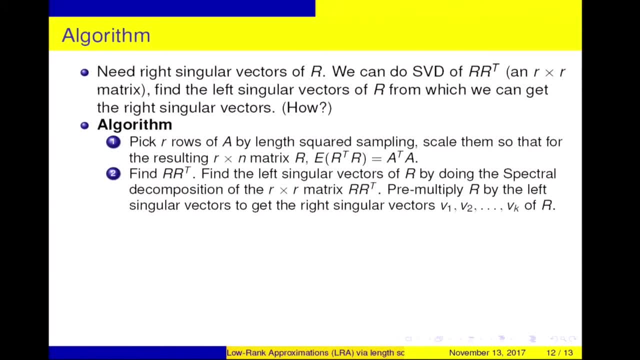 Now find R, R transpose. so I picked R. The expected value of R transpose R is A, transpose A. But I find R trans. but I find the other thing: R, R transpose. Find the left singular vector by specular decomposition. Pre-multiply R by the left singular vector to get the right. 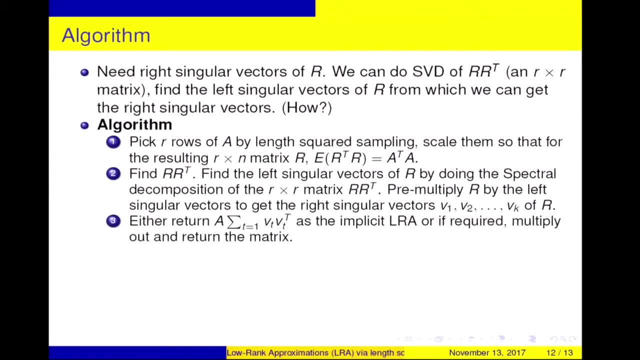 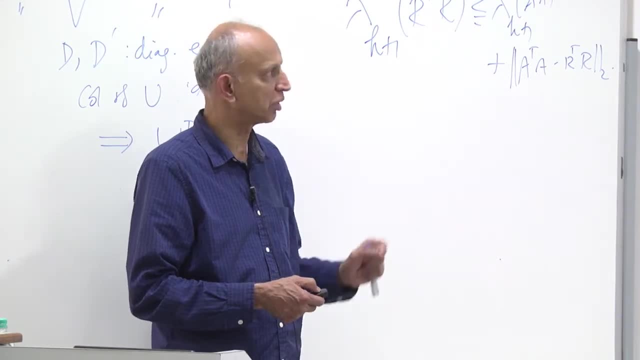 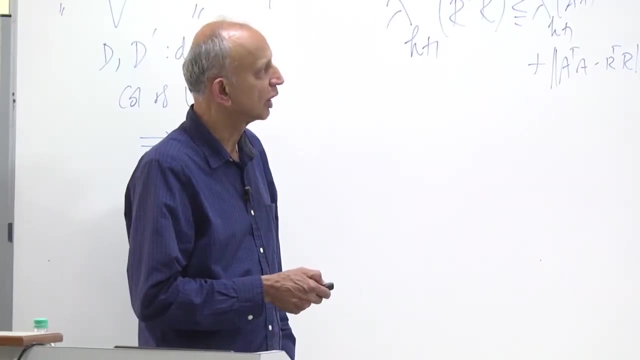 singular vectors of R. okay, all that is routine. And then you return A times this as the implicit LRA Meaning. If I don't really want explicitly what the low rank approximation is and that is useful sometimes, I'll try to show you one instance where it's useful. 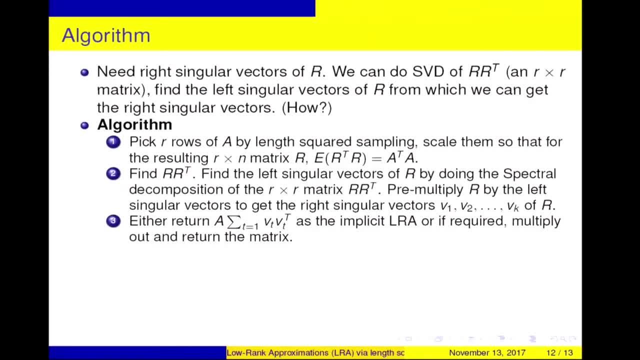 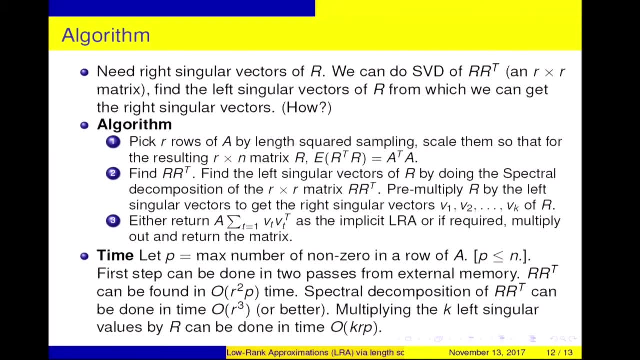 You do A times VT, VT transpose, Or, if you want an explicit one, multiply out and return At the time required, if you okay. I should mention one thing. We didn't do many algorithms here, But if a matrix is sparse, lots of big matrices have very few. 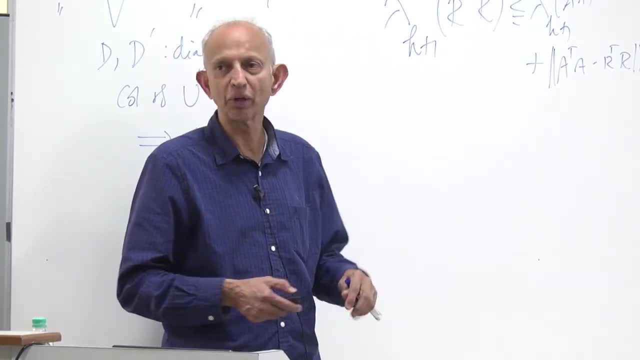 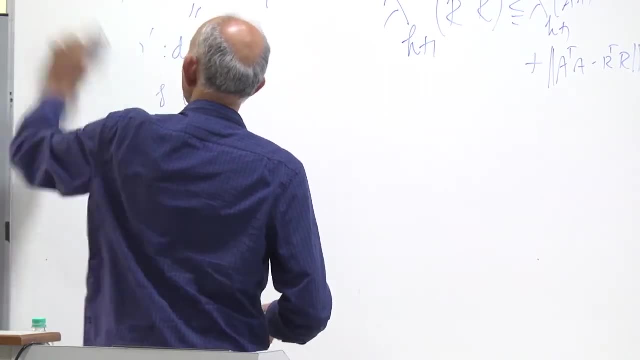 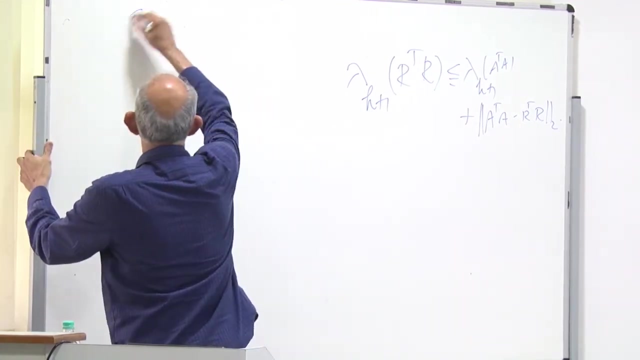 non-zeros and you don't write down all the entries of the matrix. you only write down a linked list of non-zeros. So that's a general trick. maybe I should write that So: a sparse matrix. We have few non-zeros. 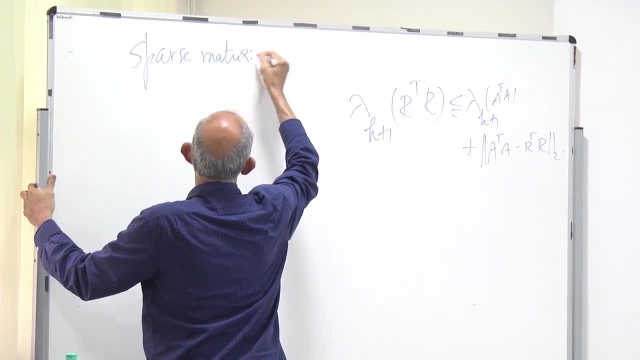 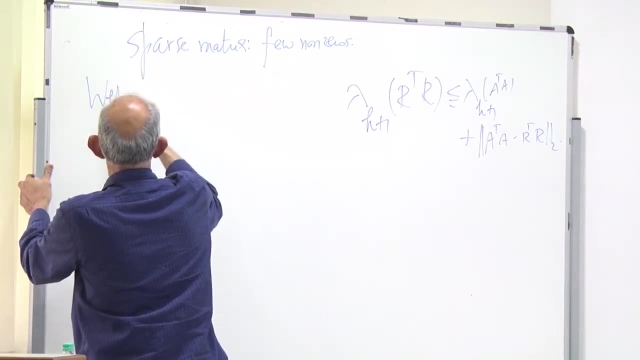 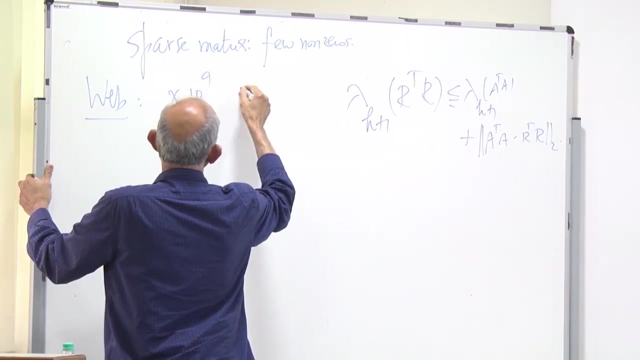 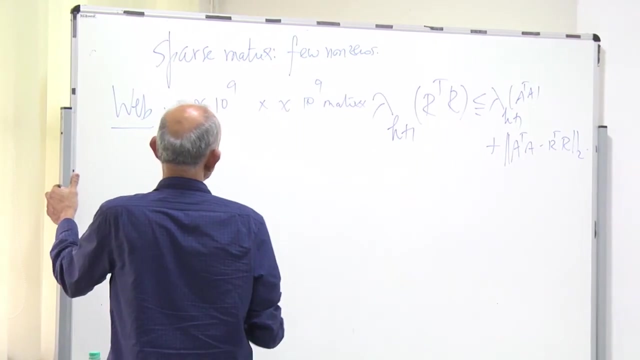 So a sparse matrix. we have few non-zeros and we only write down a linked list of non-zeros. One example is the hypertext link matrix of the web, So it has X billion right Matrix right, But each row has only about ten non-zeros. 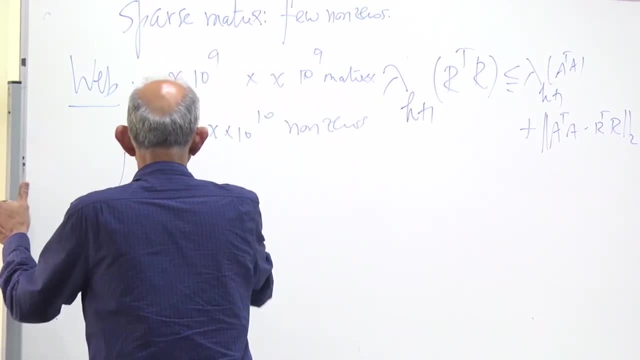 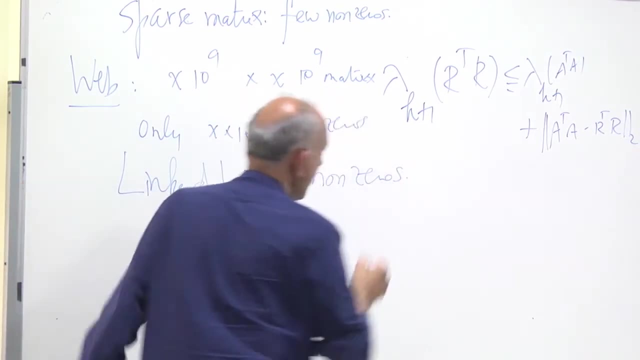 So you write it down. So you write it down by having basically a linked list of non-zeros, Linked list of non-zero entries, It just tells you where the next entry is, and so on. So you don't write down the zeros. 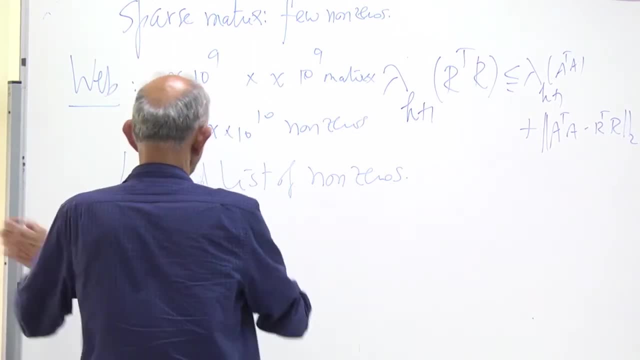 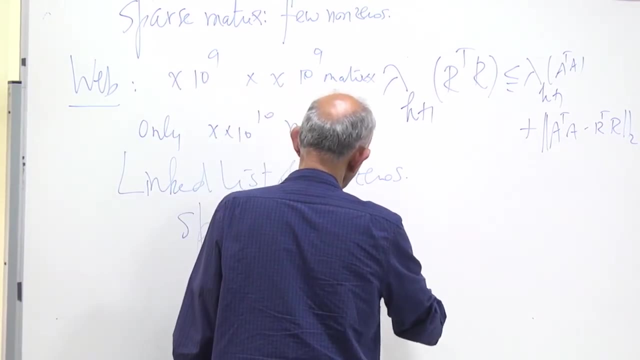 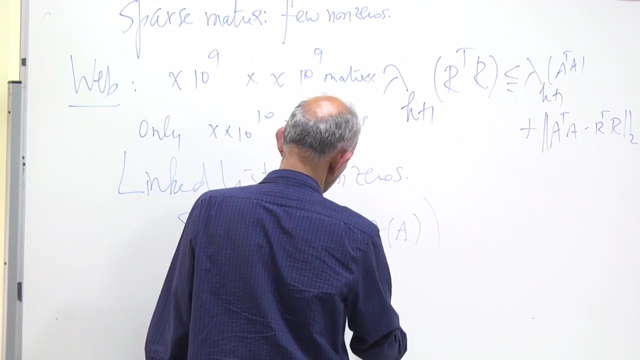 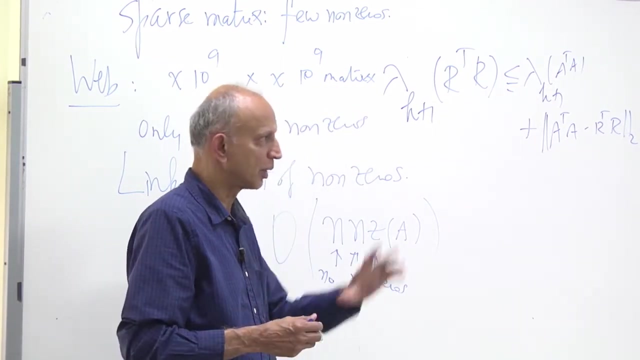 You basically have space proportional. You have space which is order. Here's a piece of notation that's now become standard: N and Z of A, which is the number of non-zeros, of A Number of non-zeros, In fact several. I didn't mention many algorithms, but 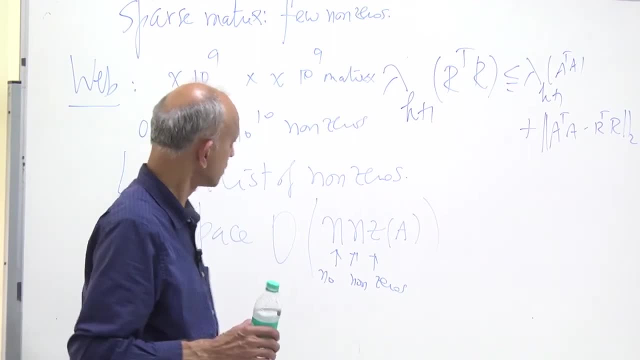 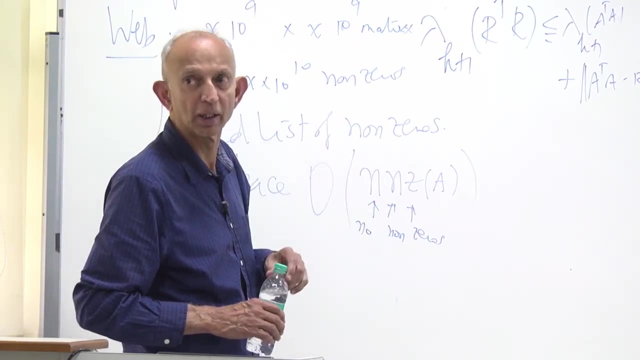 there's been some effort and people have now made many of these algorithms depend fairly benignly linear, quite often on the number of non-zeros only. So in the case of the web matrix, right if you, I don't know. 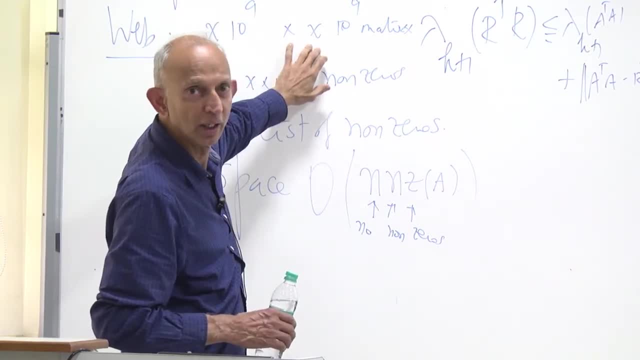 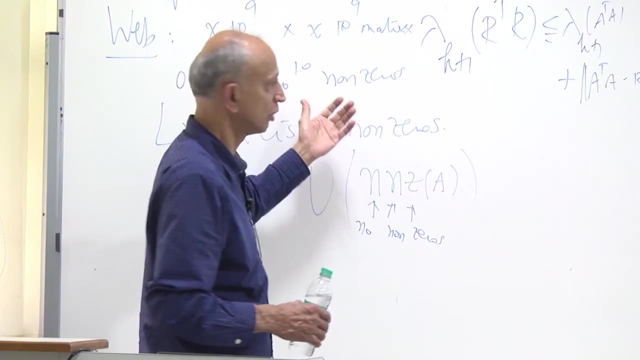 if you had an N squared algorithm, that would be pretty bad, But there aren't N squared entries to be read, So the argument is that this can all be done in time proportional to the number of non-zeros, provided the R and all are constant. 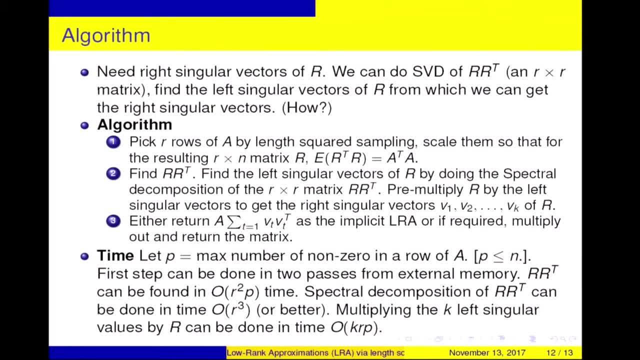 So one way to see that. so this is an advantage of sampling algorithms, by the way, over iterative methods or any of these methods. Standard numerical algebra, which is, I think, the best way to do that. Standard numerical algebra, which is, I think, the best way to do that. 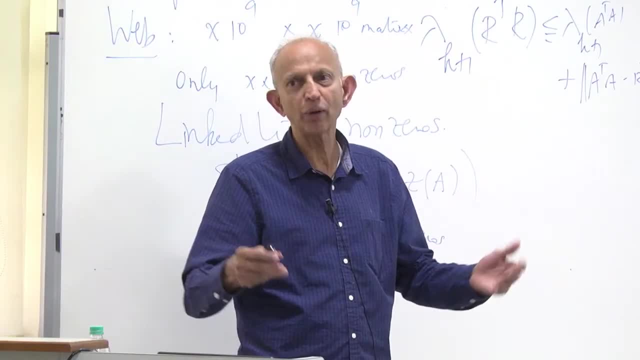 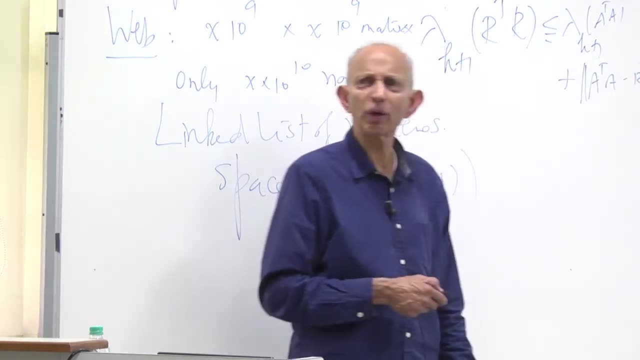 The algebra methods, unless you're careful, will fill out non-zeros, the matrix will become dense And then after a few iterations and then you're in trouble. So these don't happen with these kinds of sampling-based algorithms. just because you work only on a sample of the matrix. 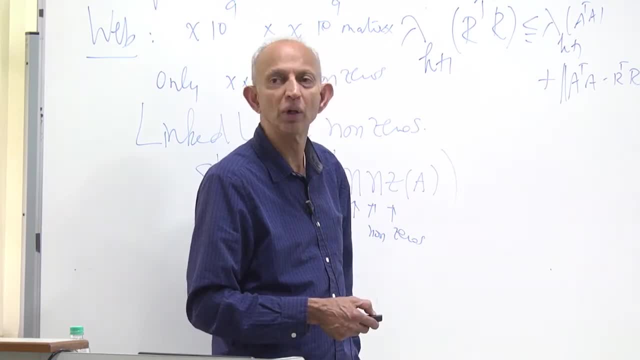 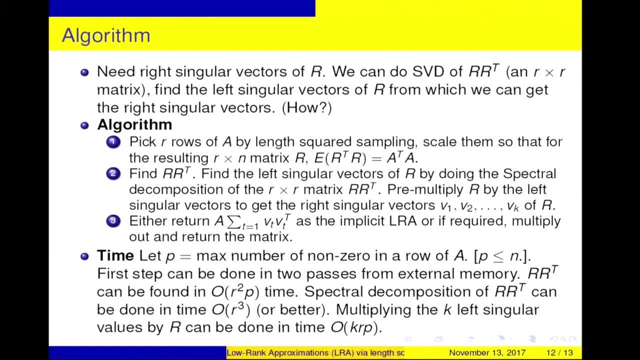 So if p is the maximum number of non-zero entries in any row, in this case p is 10.. Now, it's not true that the maximum number is 10, but pretend that it was the average, then it would be 10.. 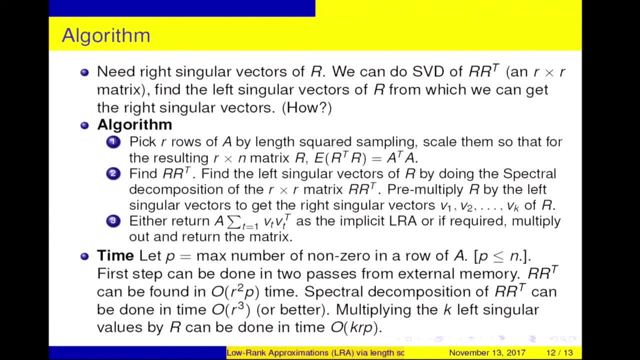 So the first step is to make sure that the maximum number of entries is 10.. So the first step is to make sure that the maximum number of entries is 10.. The first step can be done in two passes from external memory. So we saw that how to sample going through the matrix twice. 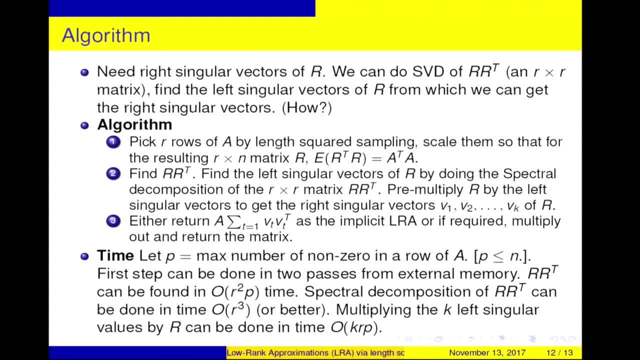 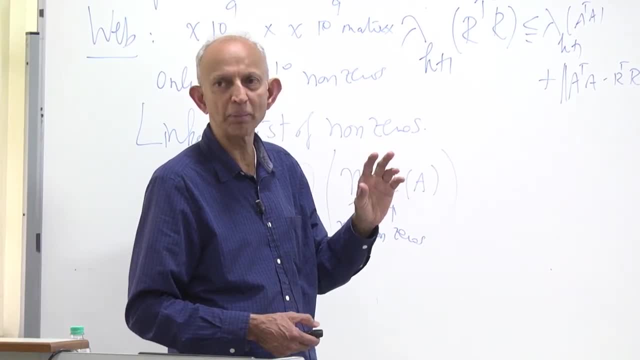 from external memory, right? You compute the probabilities one step and the next step You pick them out. Then you find RR transpose. Now RR transpose is R rows multiplied by R rows, So R squared multiplications, but each only p time, right? 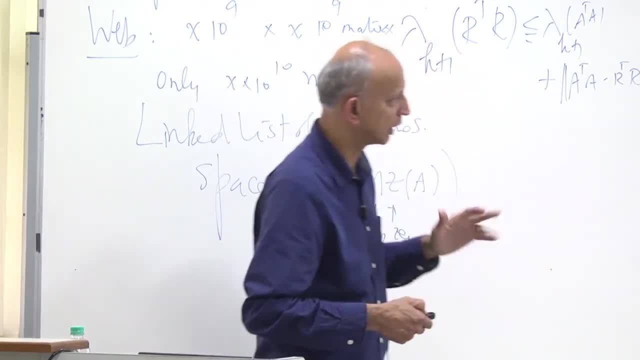 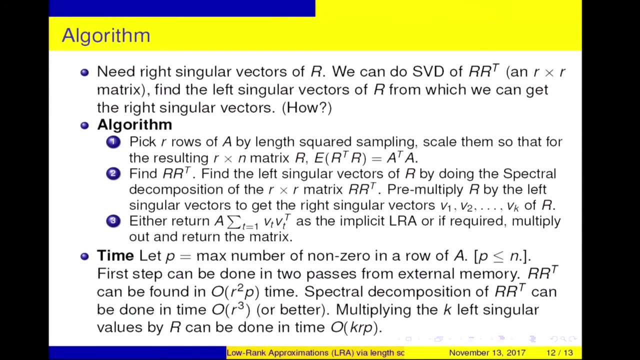 They're only p non-zeros. Dot product of two vectors with p non-zeros only takes p time. Spectral decomposition can be done in R, cubed time or better. R is to be thought of as a constant right, And p as well. 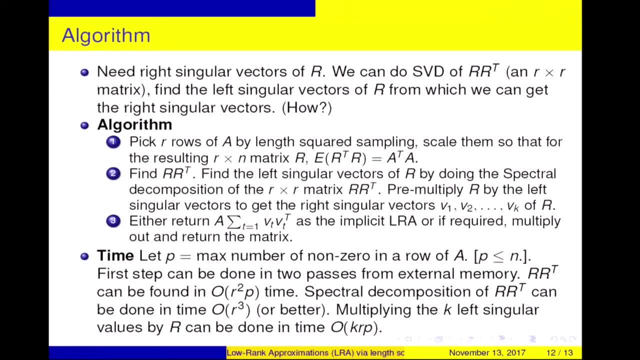 So multiplying the k left singular vectors of R. So this gives you the left singular vectors of R. The right singular vectors can be found in time k times, R times p. okay, So you do take time, dependent on n, for reading through the entire matrix. 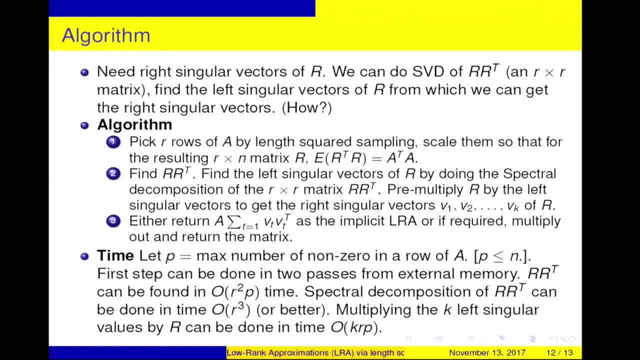 But after that the times are not right. Unless you want to do this multiplication, then you have to go through the whole matrix once more. okay, So roughly, the time is linear in the number of non-zeros, And that's typical. we didn't do this kind of analysis before. 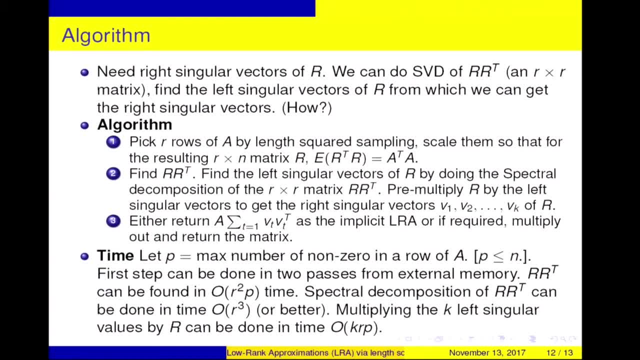 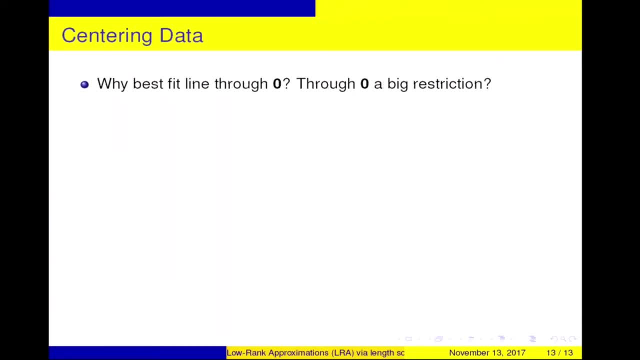 but it's typical of these sampling methods. okay, Now I want to do one more slide and then tell you something which I didn't put on the slide, So I mentioned in passing earlier. on right, SVD requires only finds the best fit line through the origin, right. 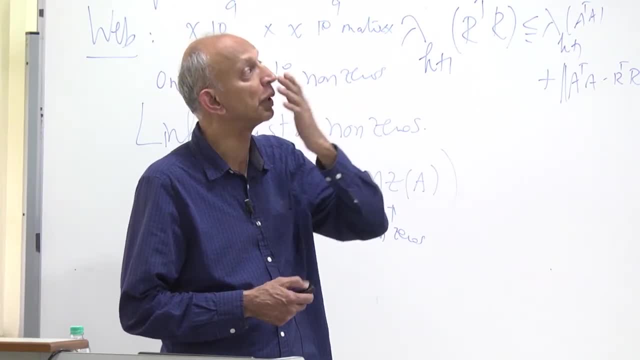 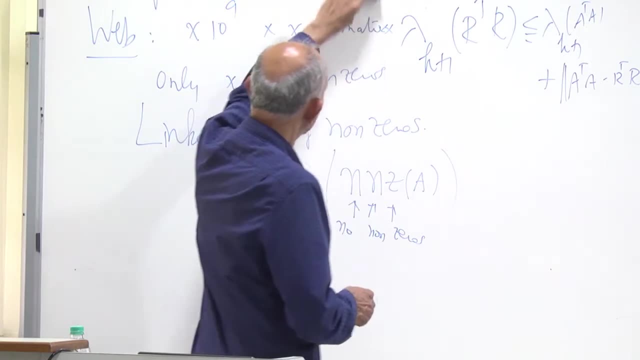 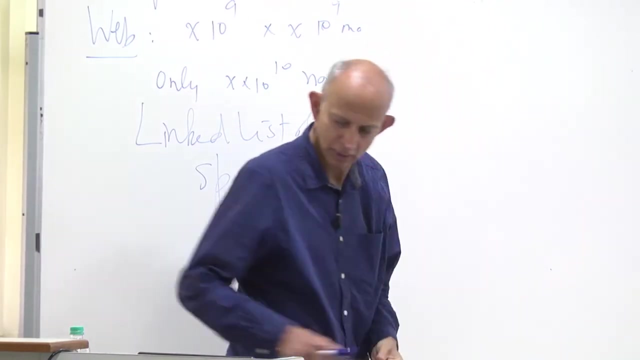 Subspace is always passed through the origin. It only finds subspaces through the origin. okay, Now you could have data which is nowhere near the origin, And then this is a big restriction. So here's the origin and all your data could be here, and 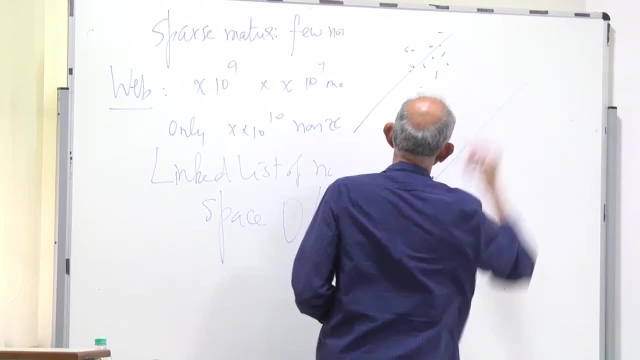 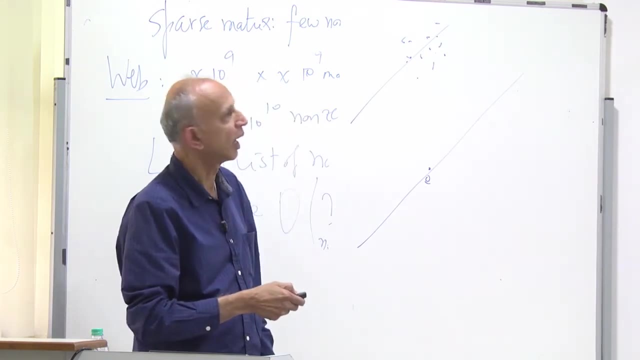 the best fit line. The best fit line might be like this, but you might end up finding this all right, So you don't want to do that. How do you avoid doing that? So first, the definition of line: space of dimension k. 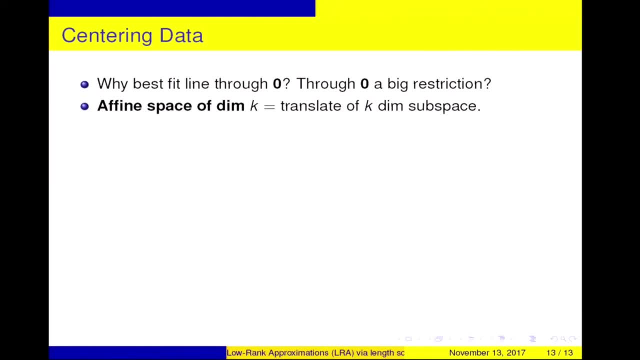 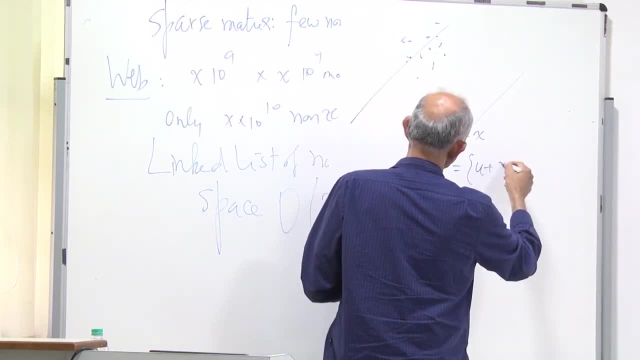 is just a translation of a k-dimensional space. Translation just means: so, this is a vector space. v, v plus x. translation just means the set of u plus x, u belongs to v. Okay, I mean, it's just moving like that. 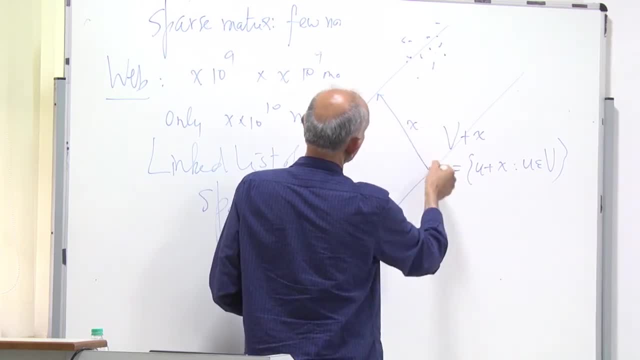 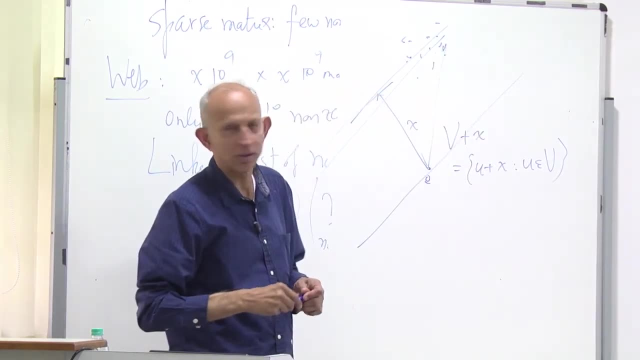 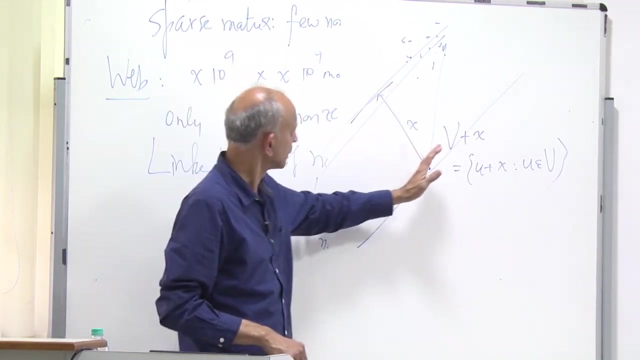 If it's a perpendicular translation, this is an x. It just moves up that space. It's also true that this x also is a good right. You can translate this by this vector or this vector. you get the same thing. All that matters is what the perpendicular component is. 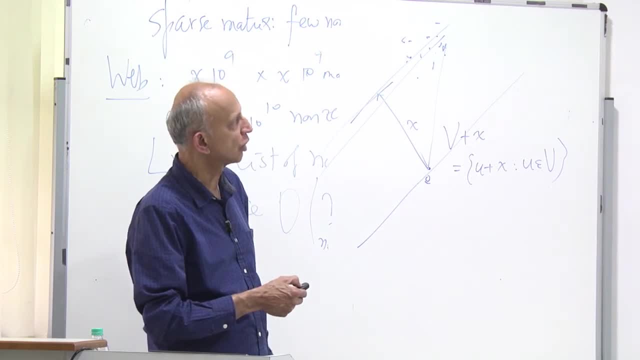 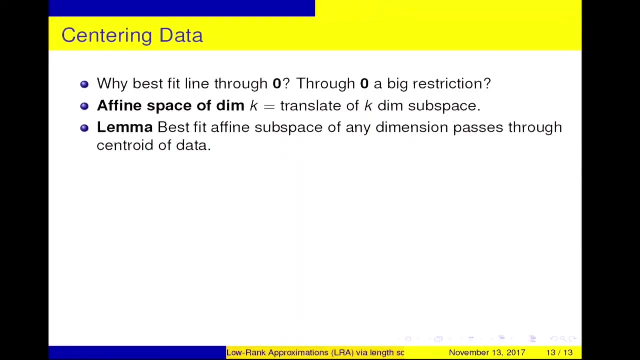 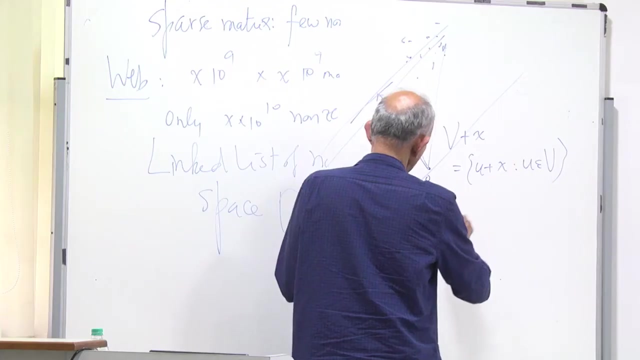 Okay, that's just a definition. right, That's called a fine space. So the lemma I want to prove is fairly simple: is the best fit of fine space? Okay, any dimension passes through the centroid of the data, The centroid of the data. you have data points a1 through an 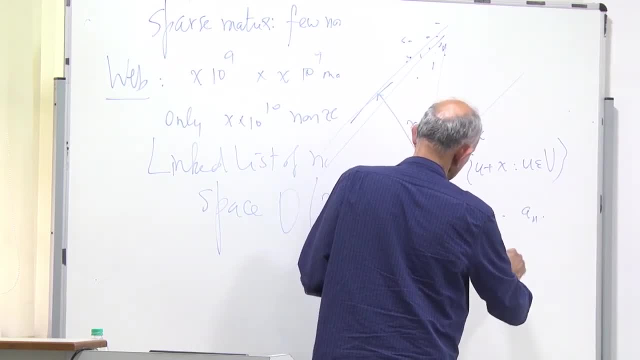 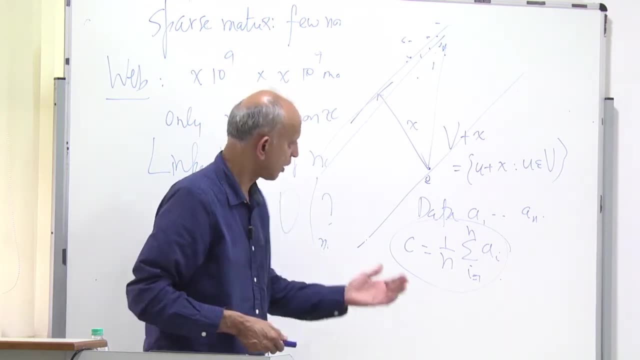 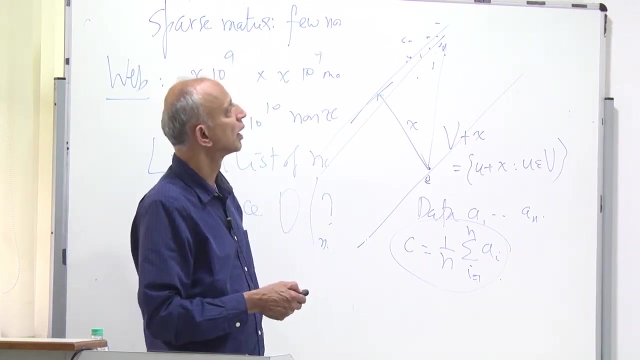 Centroid. c is just what you think it is. These are vectors. It's just average. right Average is going to mean component-wise average. Just add them up as vectors and divide by the total number. Okay, so the proof is that. if it's not the case, 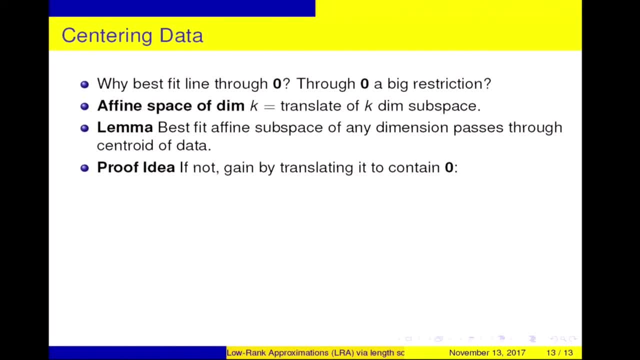 if you had a best-fit subspace which didn't pass through the origin. it's a contradiction. You're going to gain by translating it to contain 0.. So first let's prove this. So suppose you have real numbers: a1 through an, and. 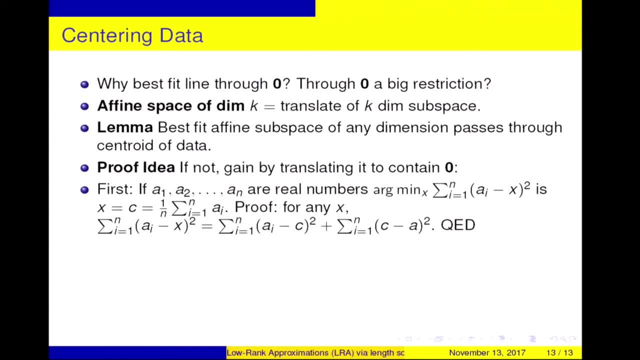 I want to choose an x to minimize sum of squared distances of ai. It's not difficult to see that the centroid is the right thing. I mean this also comes up in defining variance from mean and so on. right, So proof okay. so let's quickly go over the proof. 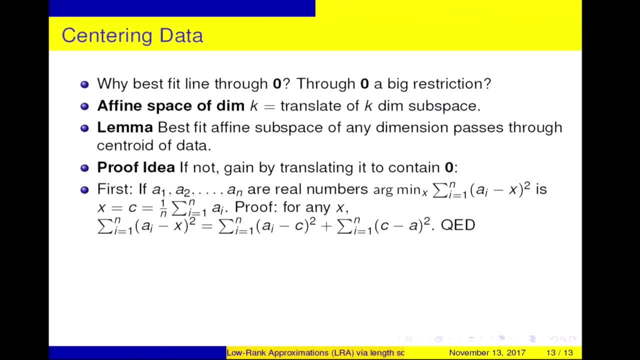 because this is typical proof that's used in many places. So I'm going to expand: ai minus x, whole squared. So I write it as ai minus c plus c minus a. I'm sorry that's not a, that's c. No c, sorry, that's all right. c minus x, that's x. 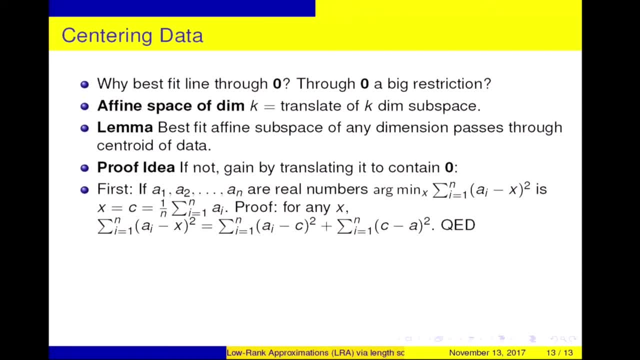 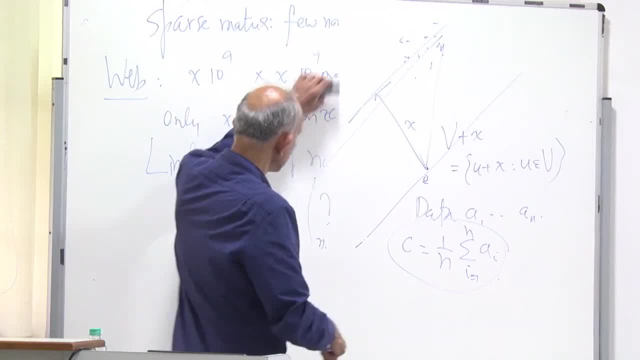 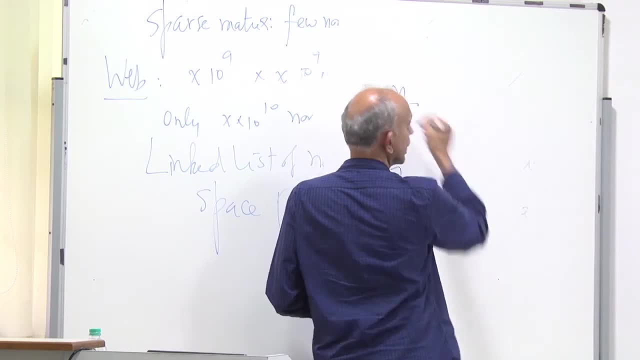 Okay, that should be an x. There's a cross term that I omitted because it's 0, right, So there's a term. so there'll be three terms when I expand the whole square, So I'll also get a term. sum over i equals 1 to n. 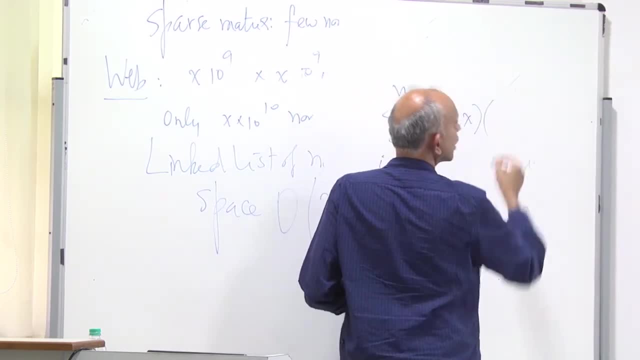 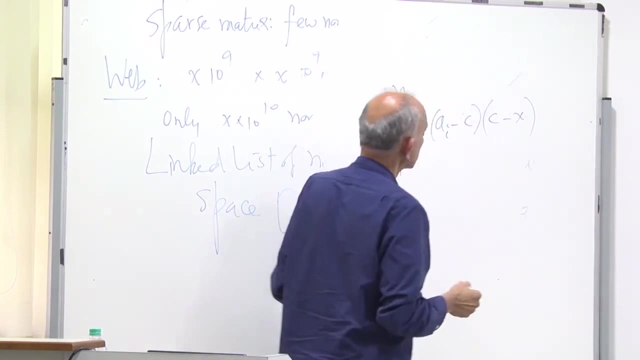 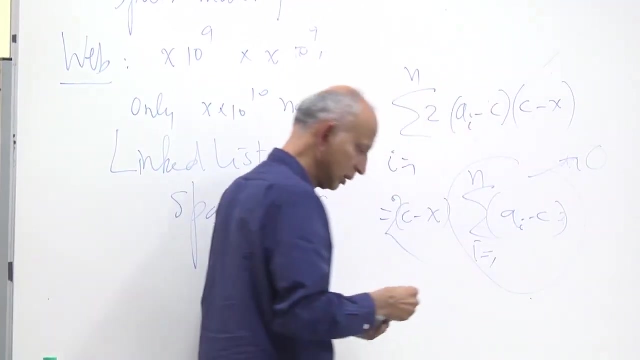 The twice ai minus x, times no ai minus c, times c minus x. This is 0. because c minus x comes out, is a constant, is independent of the ai. 2 also comes out. Sum over i equals 1 to n ai minus c. this is 0, right. 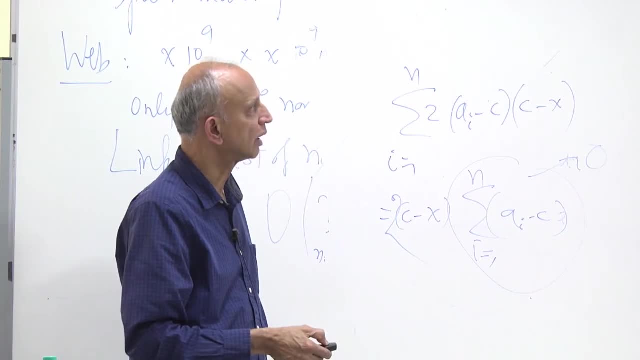 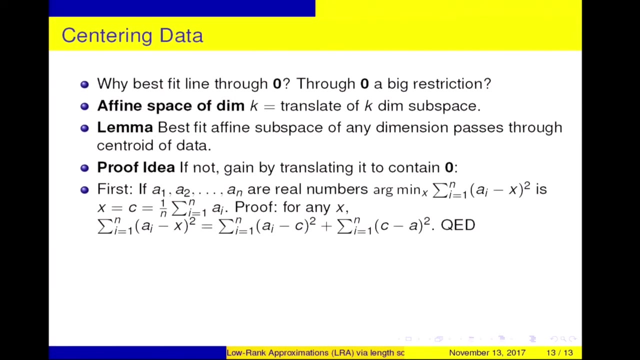 So that goes away. so you get that. That proves that for the case of real numbers, right? Because this is a non-negative quantity and the best value you can have for it is 0, and 0 means x equals c. 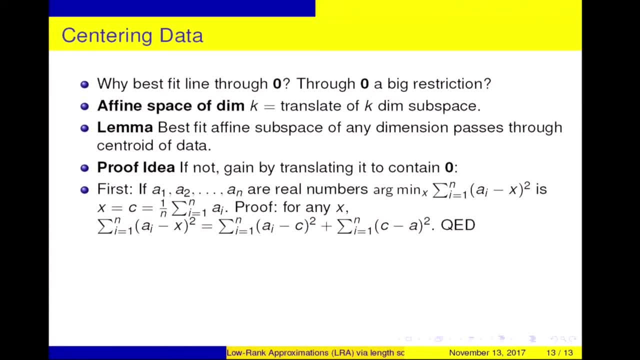 Okay, that's the lowest value: x equals c. That's the lowest value: x equals c. That's what we wanted to prove. Same thing is true for vectors. Okay, so I want to prove this for vectors. actually. So, ai minus x, I want to minimize the sum of squared distances. 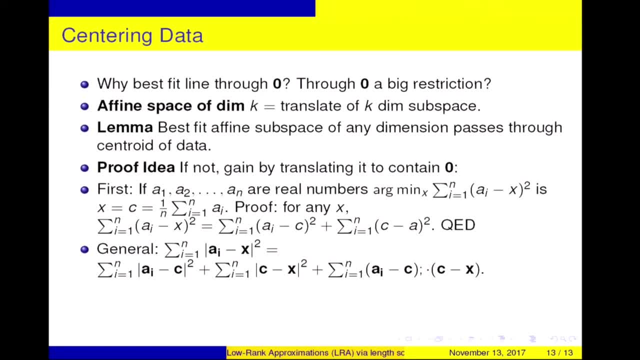 I'll come back to how you apply this really. So I write it as ai minus c plus c minus x plus. I also put the cross term here. Cross term is: what is the value of c? What's the value of c? 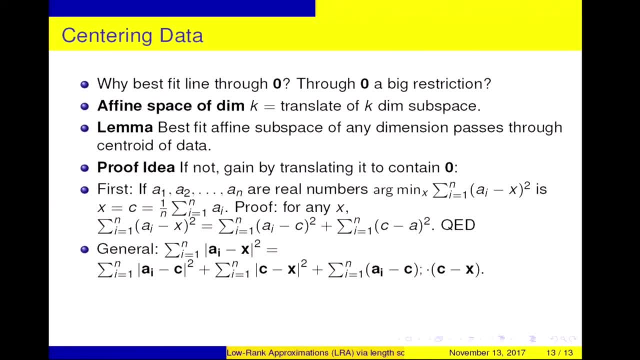 term is ai minus c, dot product with c minus x, right, That's dot product. I'm just using the fact that length squared of a vector is dot product with itself and it's the sum of two vectors. If you expand it, this is what you get and that term is zero. 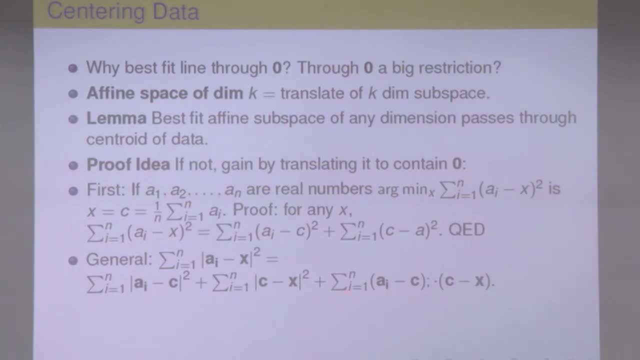 Again, c minus x comes out. even though it's a vector, the sum of these is zero, because sum of ai equals c. C is the centroid, okay, Like it was for the real numbers, Okay. so how is this used for the SVD? 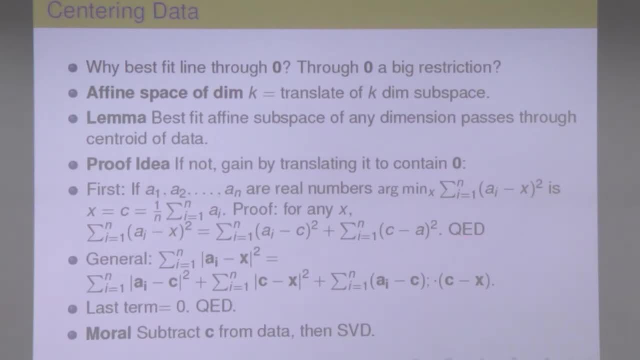 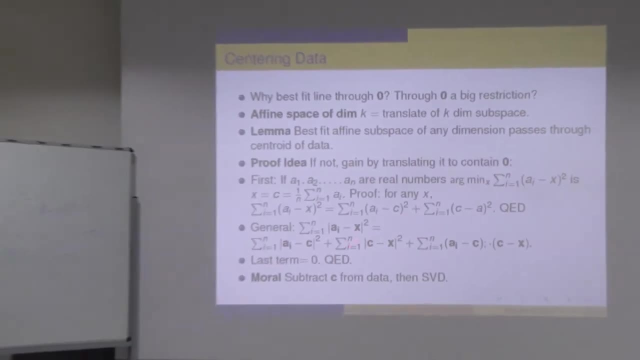 So if you want to find the best line that fits the data, rather than the one going to the origin, you could just as well find the centroid. okay, That's simple enough to do. Add all the data points and divide, take the average and. 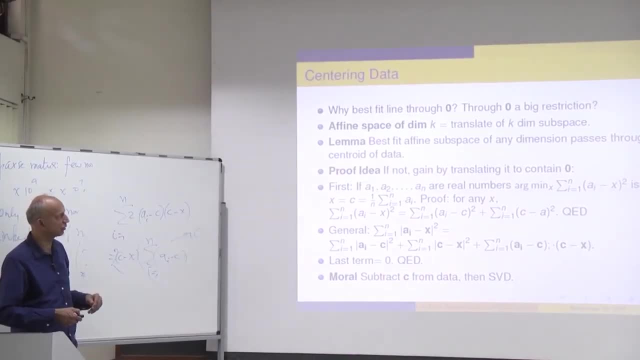 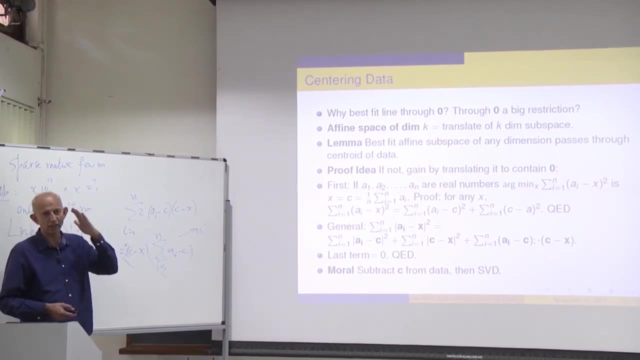 then subtract that from each data point, Subtract the centroid from each data point. Now the centroid becomes the origin. So there's no restriction in assuming that your subspace has to pass through the origin. okay, So SVD will find the best affine space if you did this. 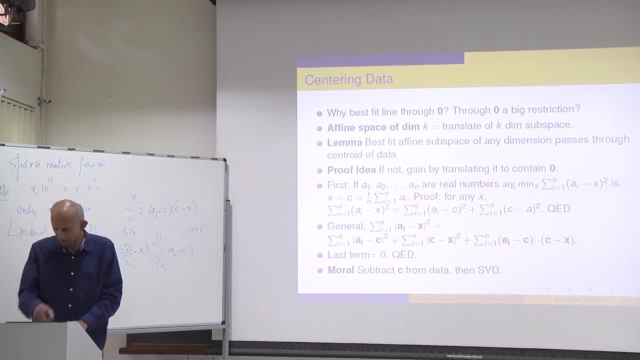 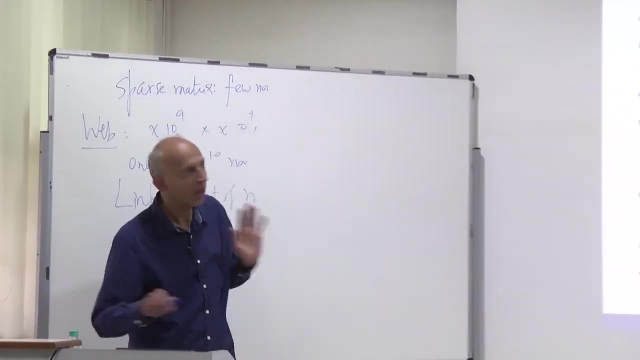 So for a bunch of applications you do that, So okay, so I think that's all I have on the slides, but I want to close by take a few more minutes to say two more things. Okay, so so far what we saw. 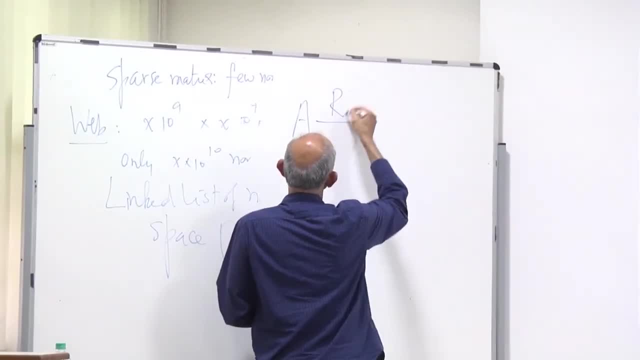 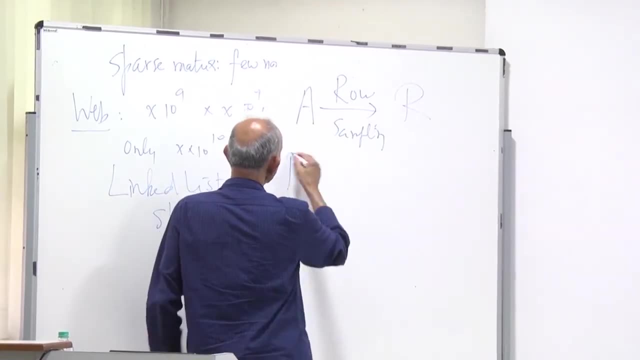 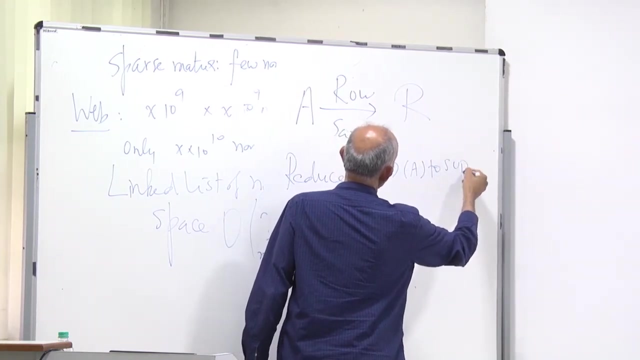 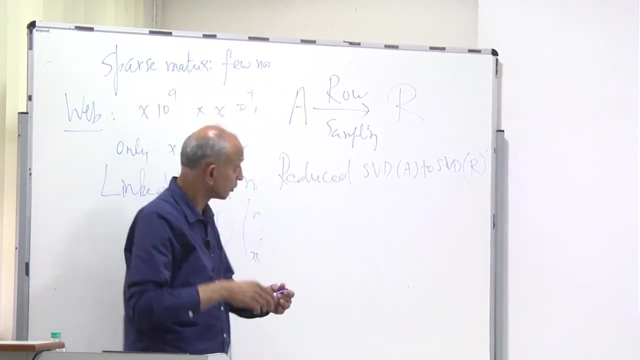 was that we had a matrix A- we do row sampling to get R- And we reduced by this process finding SVD of A to basically SVD of R. We could we further reduced it to RR transpose, but this is in spirit what we did. 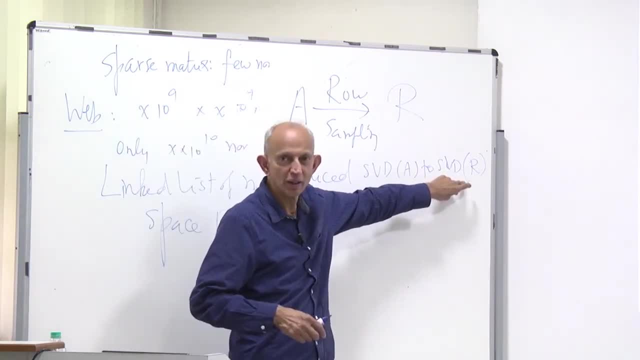 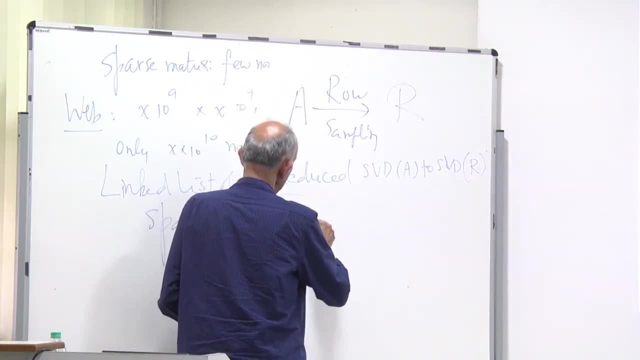 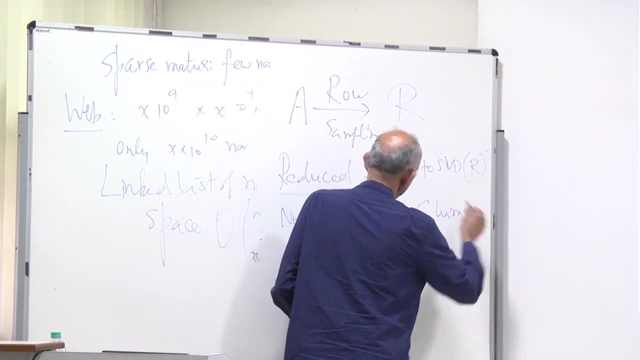 So you can ask now: I can now take R, do column sampling on R and reduce it to a really small matrix. Now can repeat, That is, I do column sampling On R to get an R by R matrix and reduce it to a really small matrix. 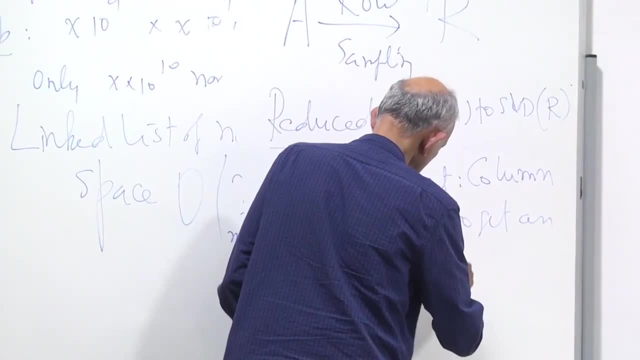 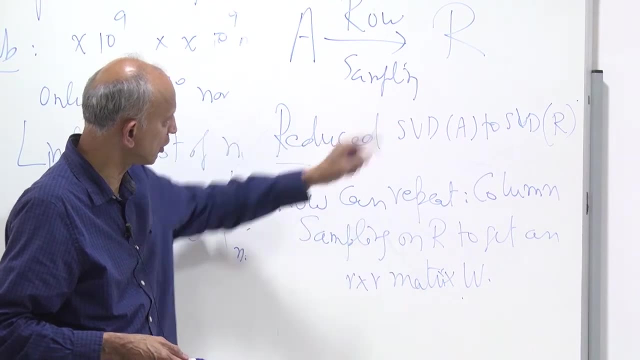 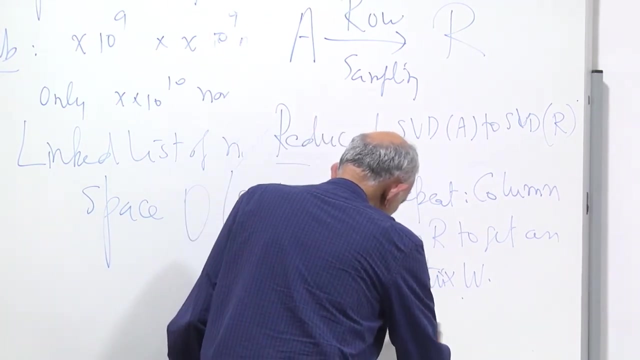 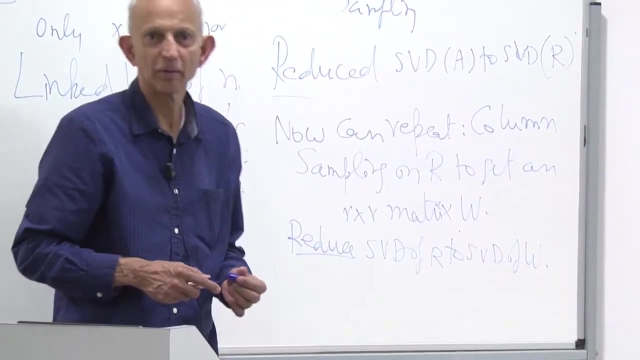 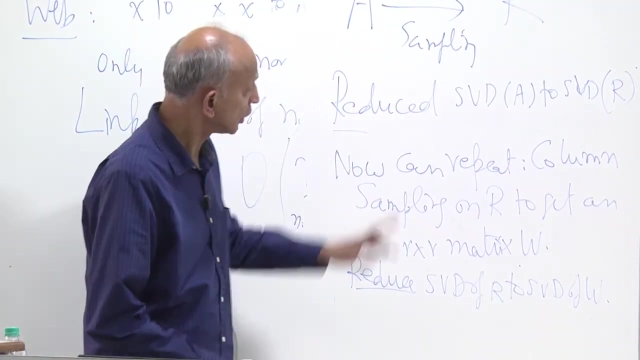 R matrix W. Okay, and intuitively I should be able to reduce SVD of R to finding SVD of W, Right, I mean, it's just a symmetric version of that problem, except columns and rows. So this is true, but the proof is much more complicated. 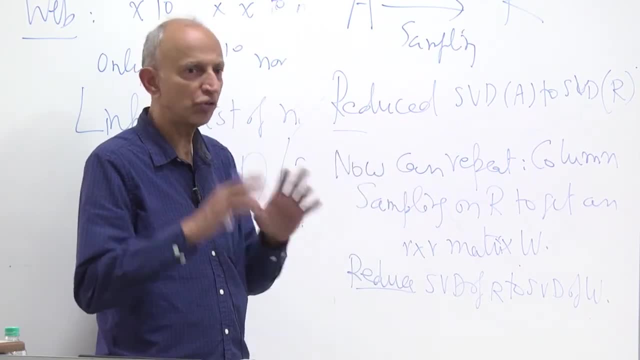 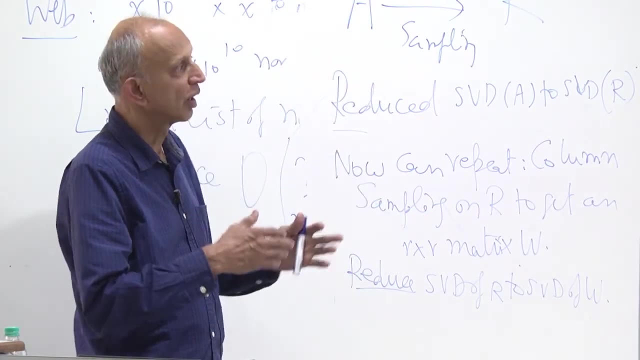 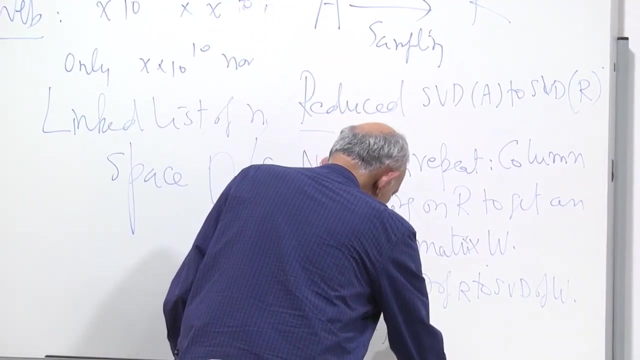 And the trouble happens because things go wrong when singular values are close to zero. So in some areas of this process we have to worry about singular values that are close to zero. So this is true, but complicated, I would say actually much more complicated. so 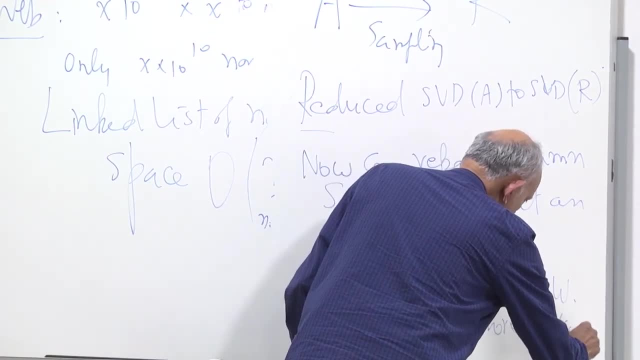 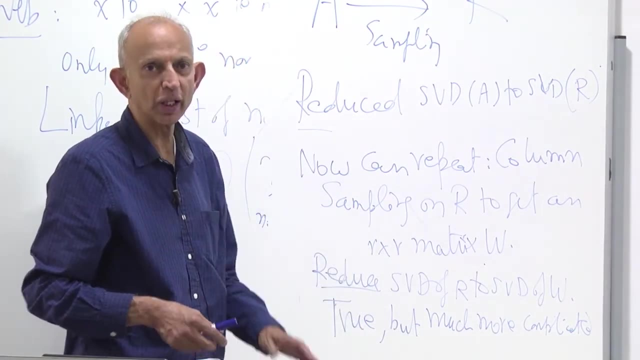 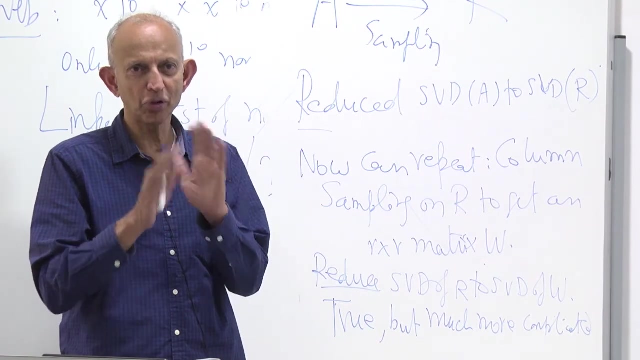 it's not simple at all, But the moral of the story is, by doing the sampling twice, you're finally left with a constant size matrix, Both rows and columns, constant number, and that's all that you need to worry about. okay, in some sense. 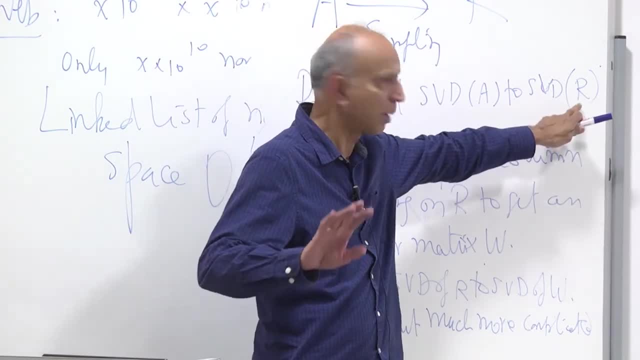 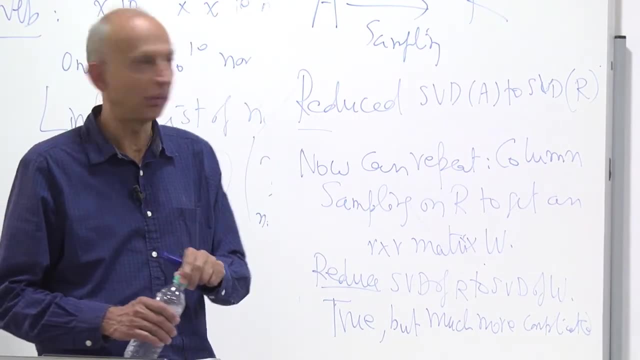 I mean that was true when we do RR transpose the small matrix. but we'd have to find RR transpose for that. So we don't have to do any computation on big matrices except to sample. That's what this is going to tell you. 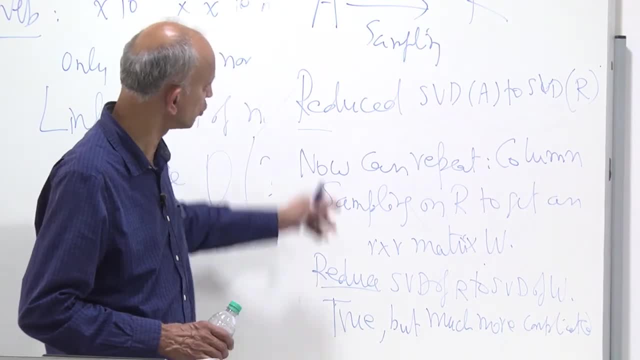 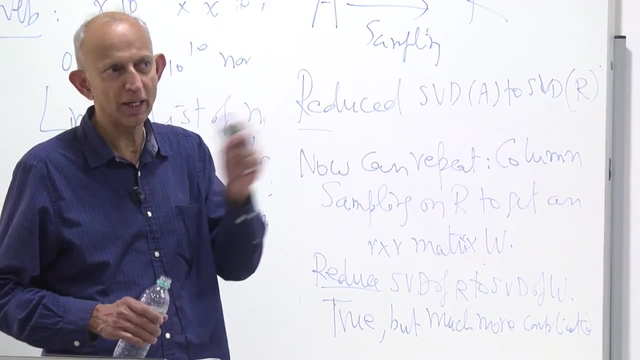 Now in practice, however, I'm not sure this has been used as much as row sampling has been used quite a bit, But both sides. I think it's too expensive still, although I'm not current on the state of the art, but 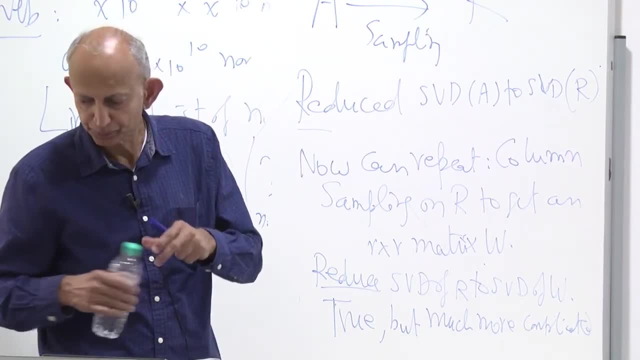 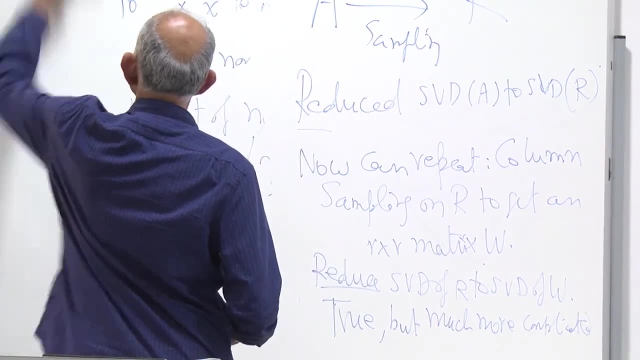 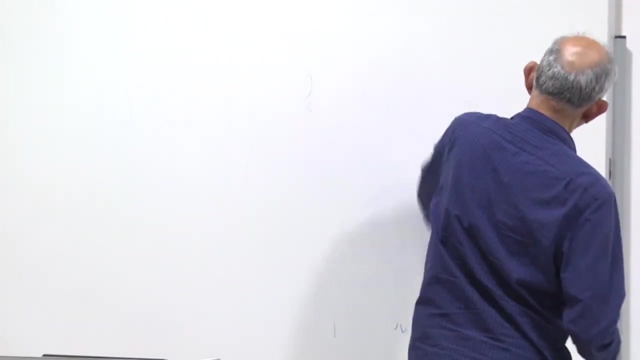 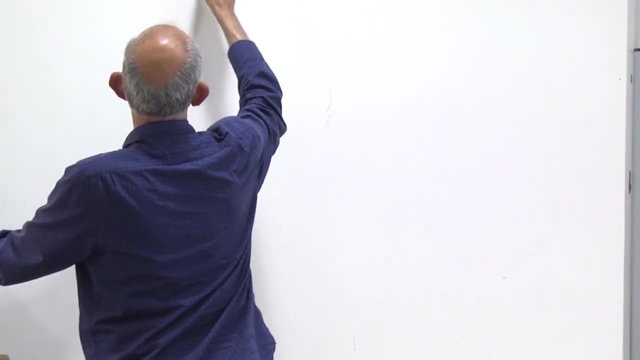 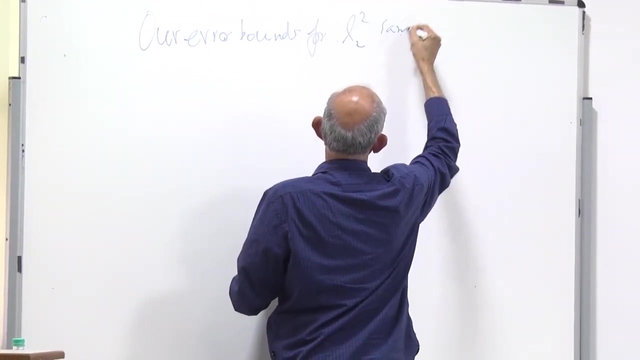 How do you do that? Okay, that's one thing I wanted to say. The other thing also, I should have put up on the slide. I'll just say that. So our error bounds for length. squared sampling always had, or? 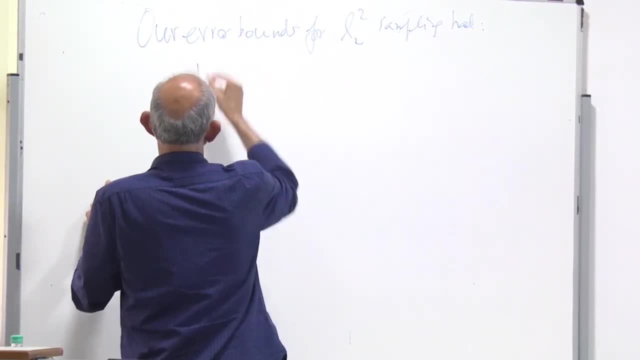 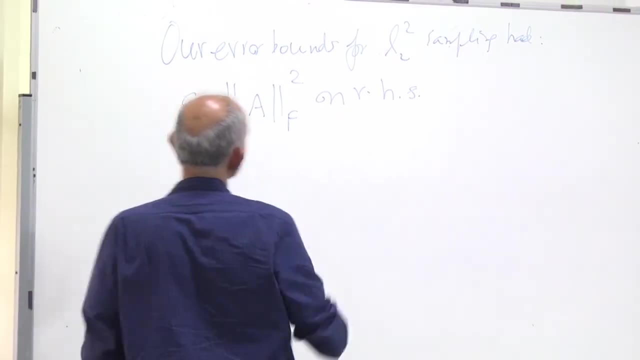 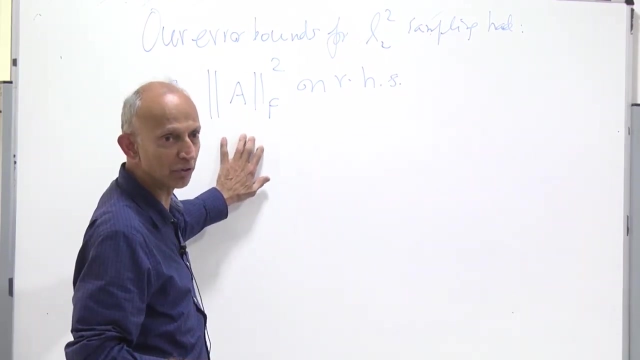 generally had on the right-hand side, not every one of them. There was one today where I had only the spectral norm, but this is what I generally had on the right-hand side, right, And I told you that I cannot replace this by spectral norm. 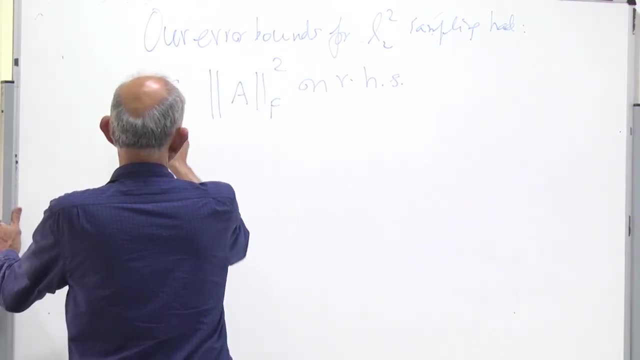 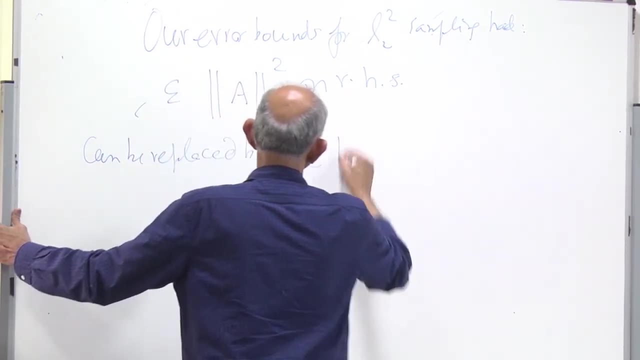 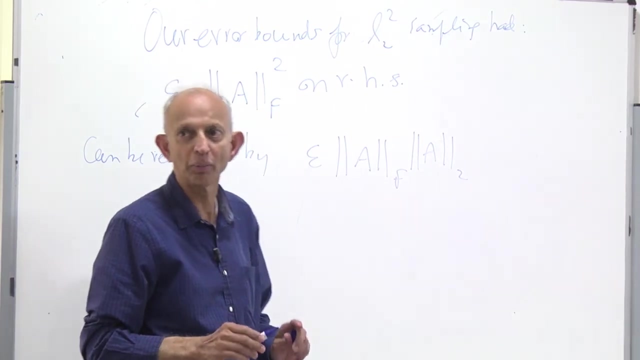 That's correct. but what's true is that can be replaced by Epsilon times, Frobenius norm times the spectral norm. So one of the Frobenius norms can be replaced by spectral norm. Now this looks just like an improvement going to another. 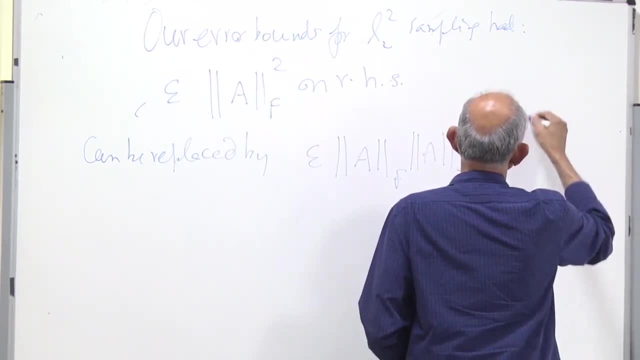 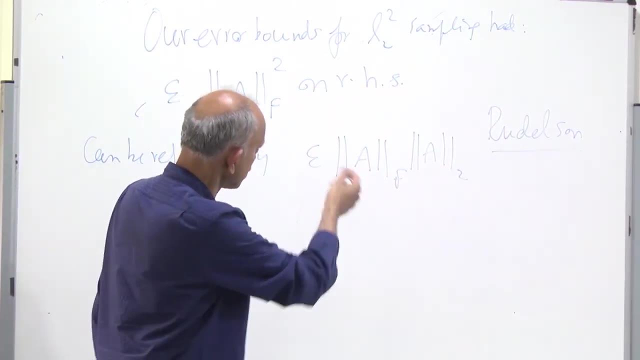 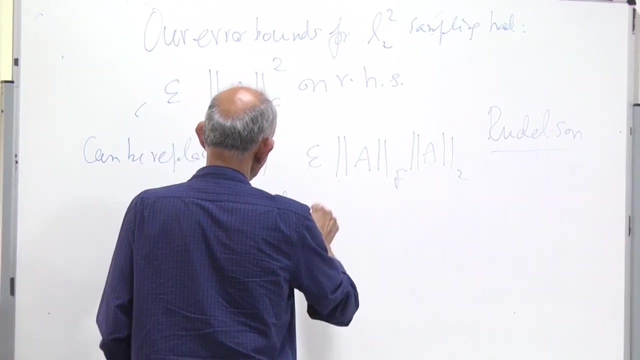 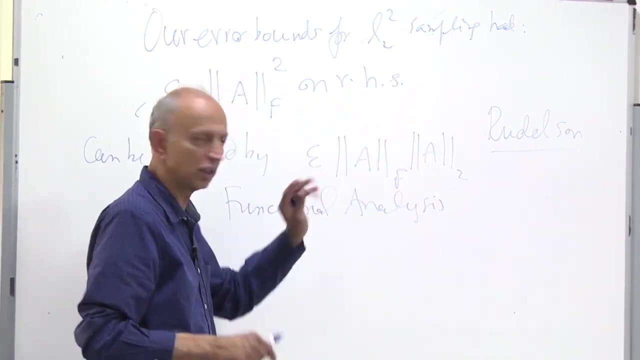 norm? it's not. This is a theorem due to Rudelson, Which came about maybe five, six years after the original paper, then after our paper. But this uses a nice bit of functional analysis. It's not simple. There's slightly simple proof of it, but it's still not simple. 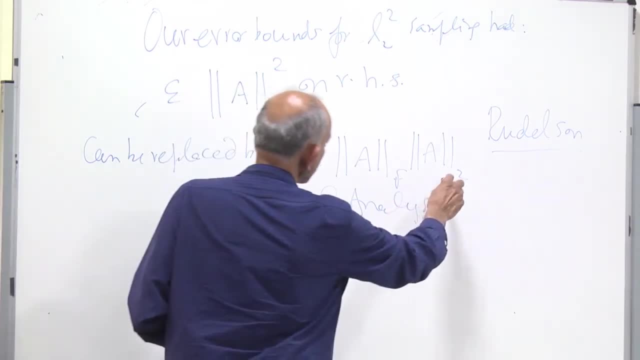 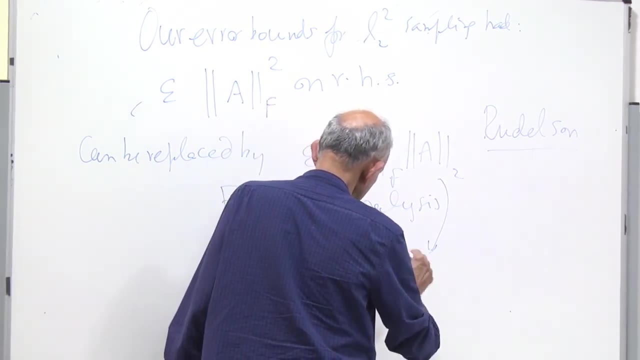 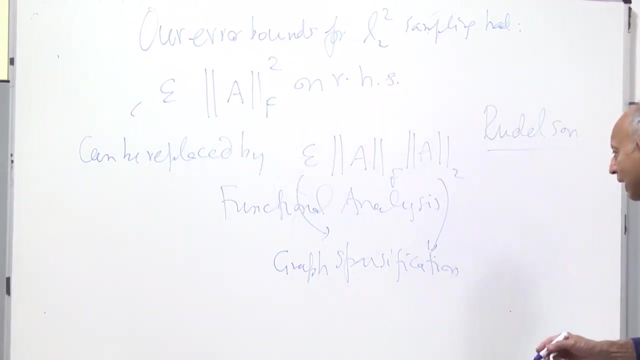 Now this turns out to lead to a bunch of things. Probably the most important thing is graph sparsification, And I'll tell you the result, but not prove anything. This is due to Spielman and Srivastava. So you need- you need the fact that one of the Frobenius norms 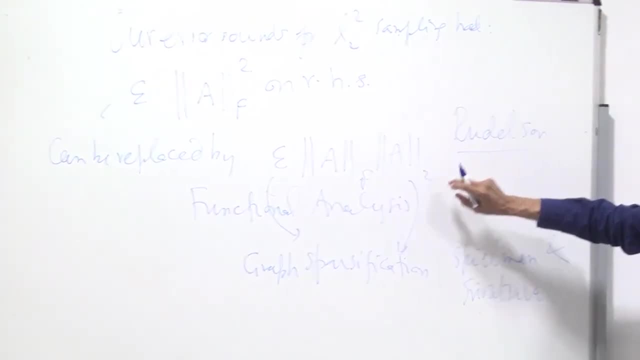 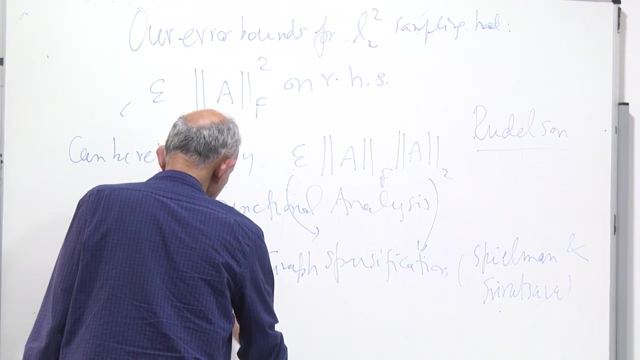 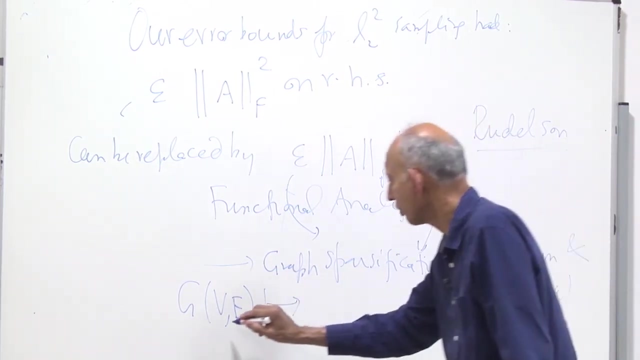 has gone to spectral norm to get graph sparsification. So graph sparsification says the following: I give you any graph Gve From that I can produce a graph. This is N vertices. I can produce a graph G, H. 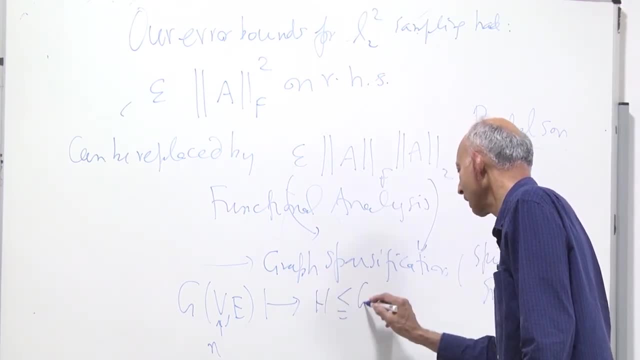 Which is a sub sqrt. This is a sub sqrt. This is an excess. this is an excess. the subgraph of G. I'll write it like this, So H is on n log n vertices. sorry, n log n edges. 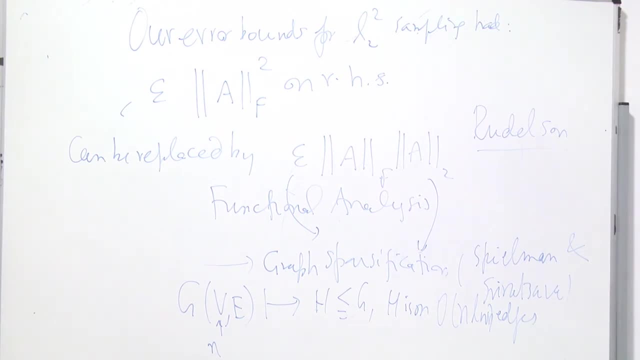 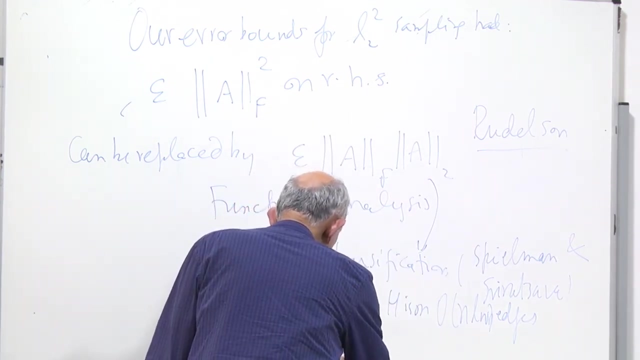 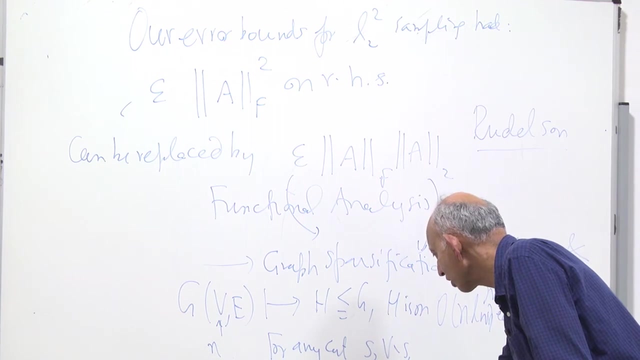 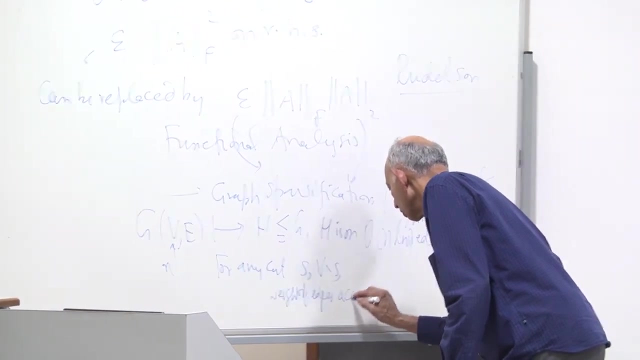 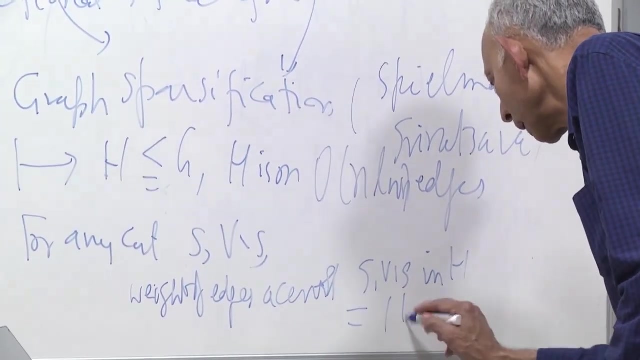 And has the property that every cut in H is roughly same as every cut in G. So for any cut S V S, the weight of edges across the cut in H- Weight of edges across S V minus S in H is within one plus or. 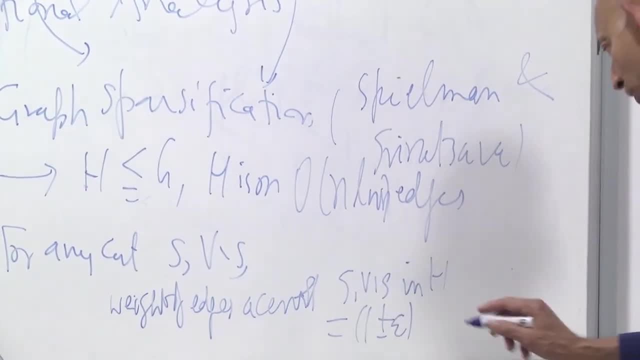 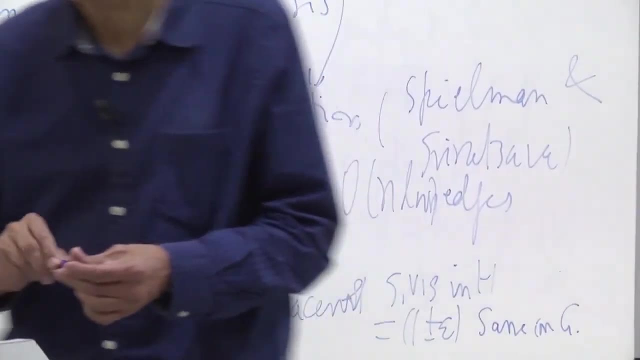 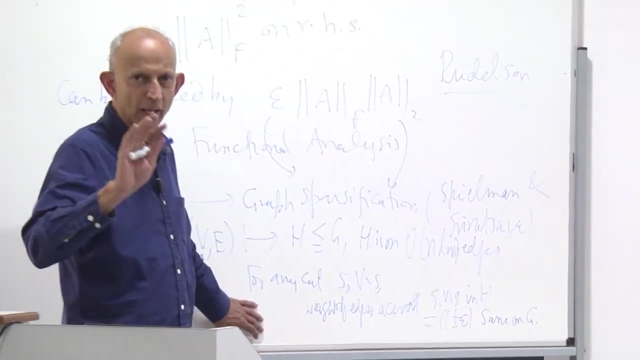 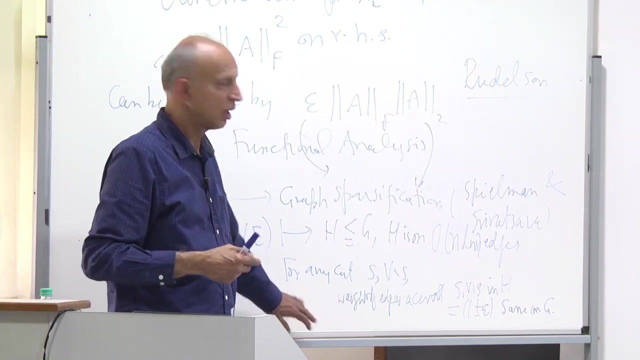 minus epsilon of the same thing in G. So it's a purely graph theory result. So what it's saying is: I can produce a much smaller graph so that there are exponentially many possible ways of cutting the graph into two parts. right, Any subset of vertices. any subset of vertices. 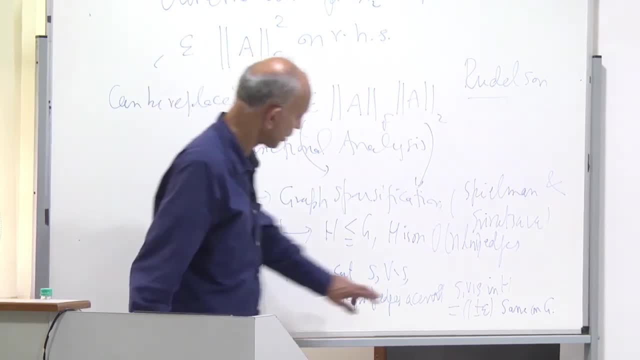 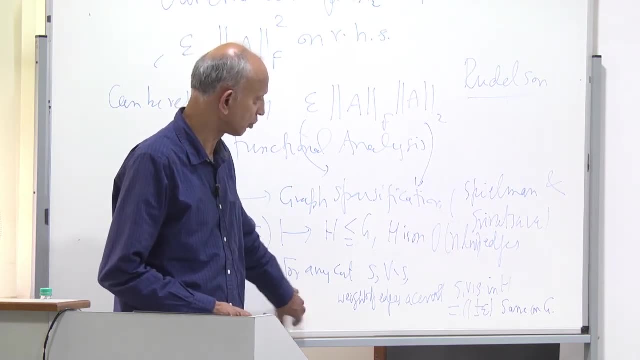 H without fail, for every cut has about the right number of edges, as G does. I mean that's completely non-trivial, I mean it requires quite a lot of work. But central to that is Rudelson's theorem about 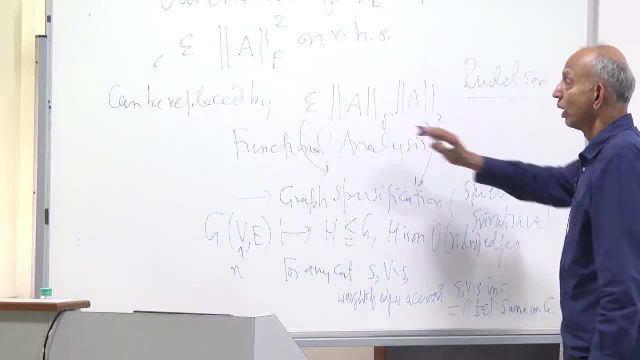 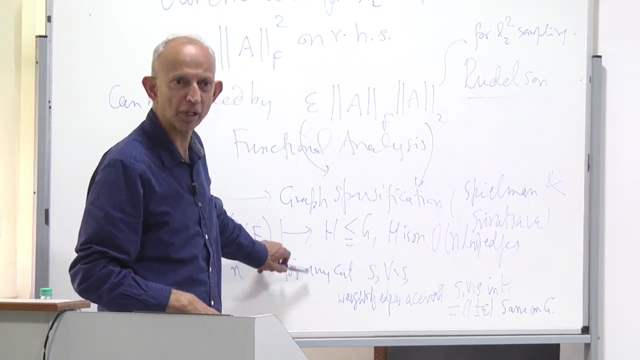 Rudelson's theorem is also about length squared sampling. So can we replace this for just length squared sampling? So I won't be able to prove that, but hopefully I've stated the result well enough for you to see. So what is interesting is, of course, that there's a purely 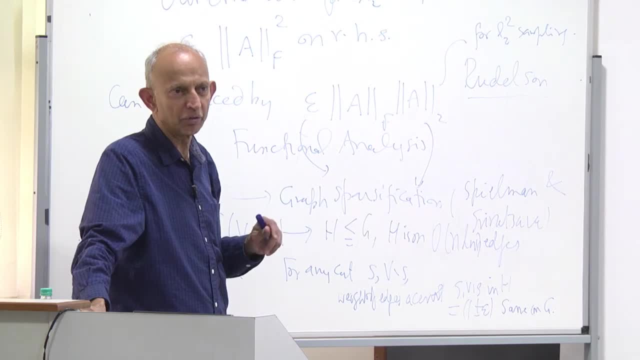 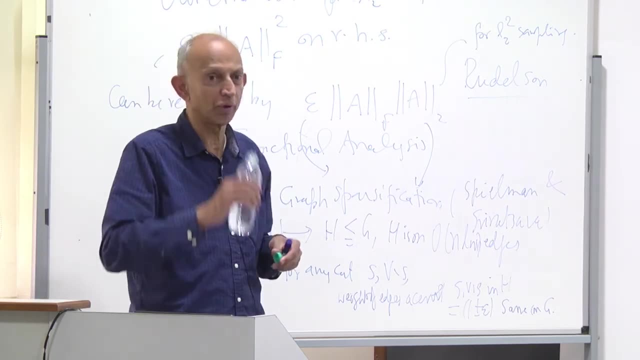 combinatorial result follows from this matrix kind of stuff, Right? Not terribly surprising, Yeah, And what's not surprising is that you're going to get these two. I think a lot of graph problems are related to matrices, but it does follow from that. 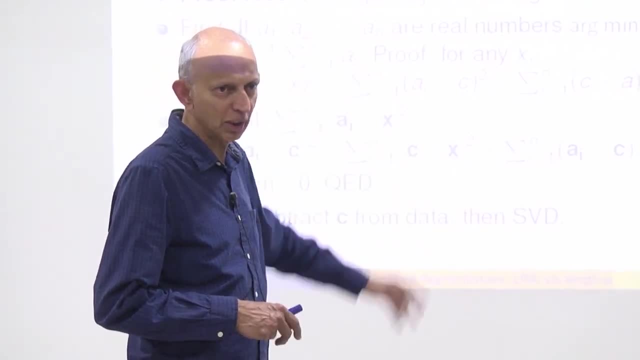 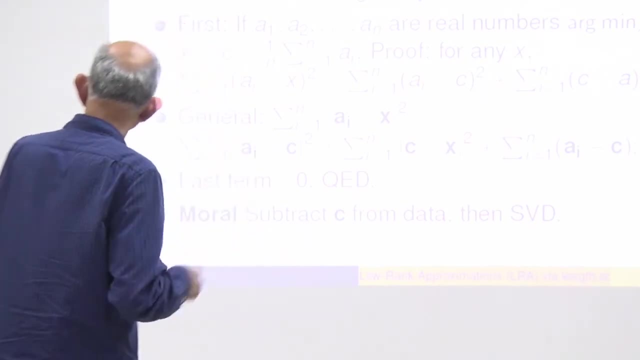 The bound today I showed is also what spectral norm on the right side. but the matrix multiplication bound, for instance, had only the Frobenius norm That can be replaced. So okay, so maybe I should say more specifically: we wanted to multiply two matrices, A and B. 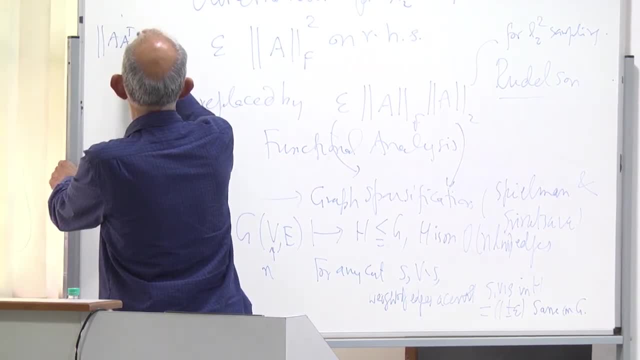 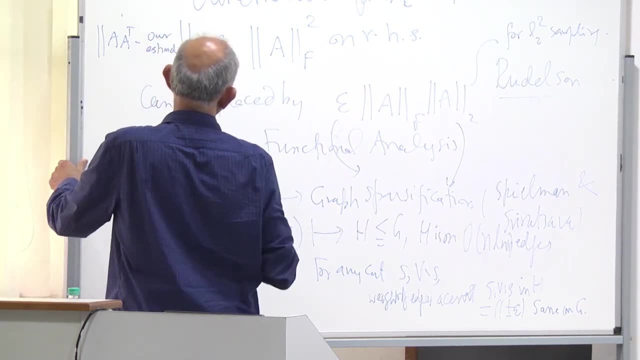 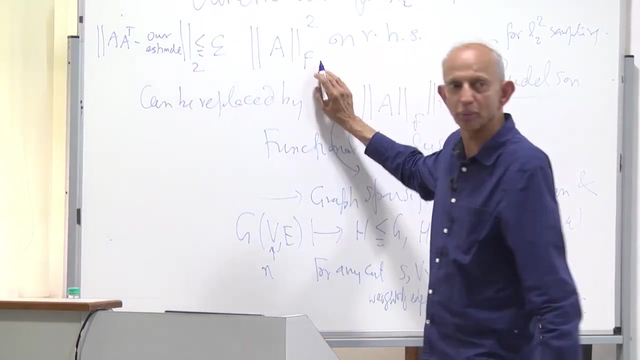 A and A transpose. let's say So: A and A transpose minus our estimate. Okay, even if I wanted to bound the two norm, the right hand side was only the Frobenius norm. What Rudelson proves is that for that specific bound, so 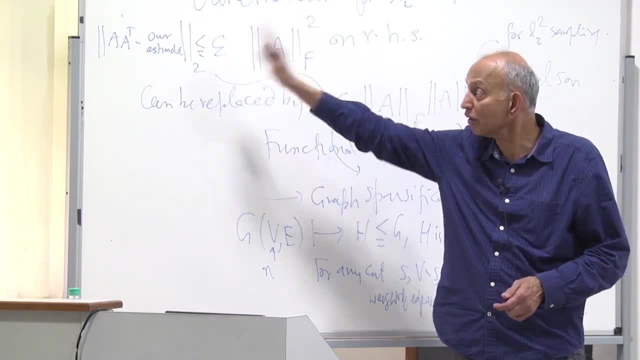 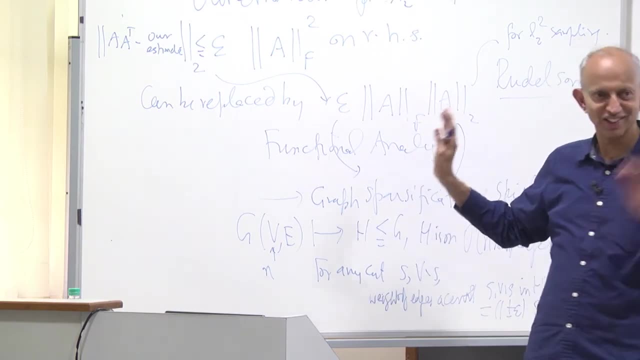 it was not precise enough for this specific bound that I want. the spectral norm of the error of the product is bounded by one Frobenius norm. you still can't get rid of this. It cannot be purely spectral. The center, I think, is for Frobenius. 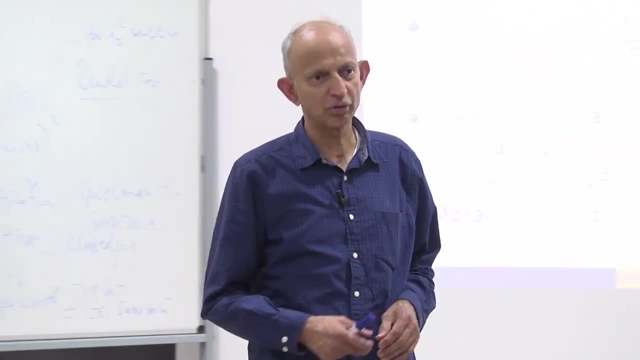 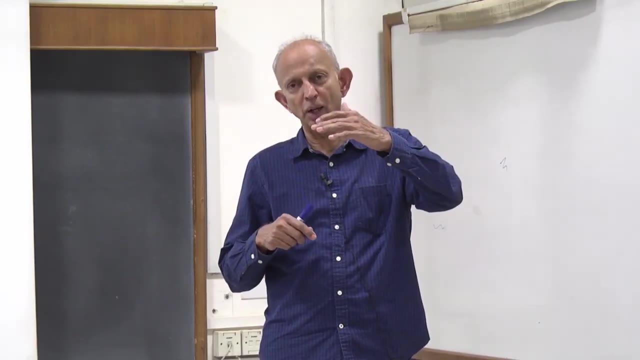 Yeah, you're right. The center, I think, is not for spectral. Actually, there's some interesting open questions there. but no, this is only for Frobenius. If the rows of A were picked from an IID distribution right. 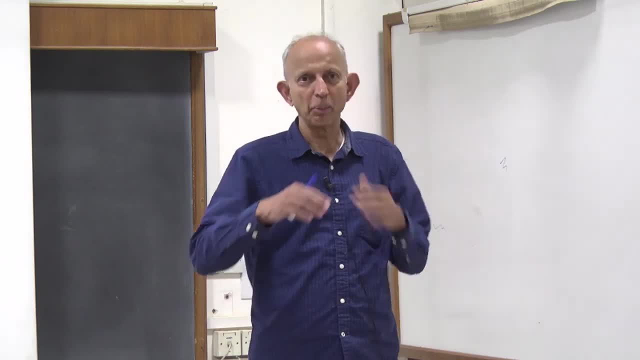 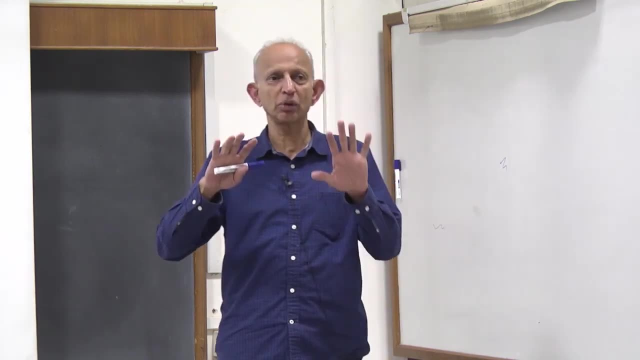 then you would probably want to center out by subtracting the mean. The mean is just the average of the rows. a very good estimate of the mean, because you've got enough samples. Then you subtract it out. then, as you said, 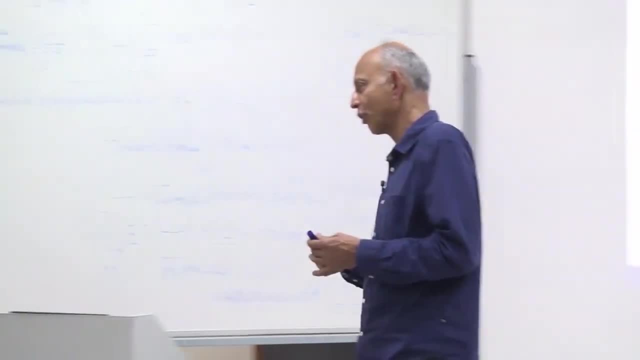 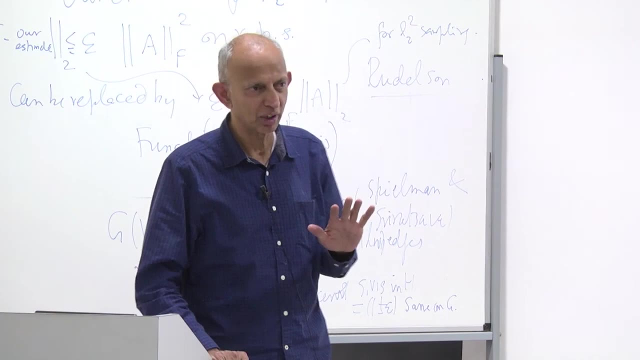 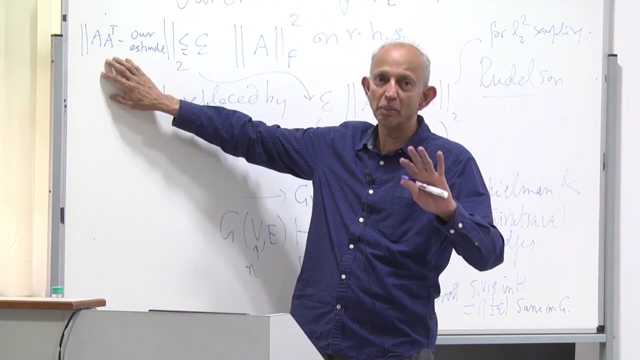 then the A transpose would be the variance Variance covariance matrix. A transpose, A AA transpose is really the variance covariance matrix. So I think I mentioned this once. the original motivation for all these sampling results basically came from trying to estimate the variance covariance distribution.